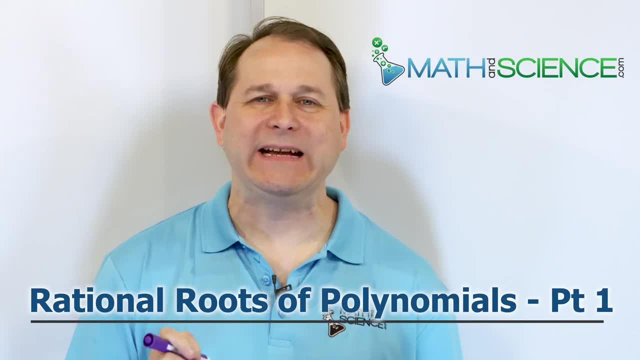 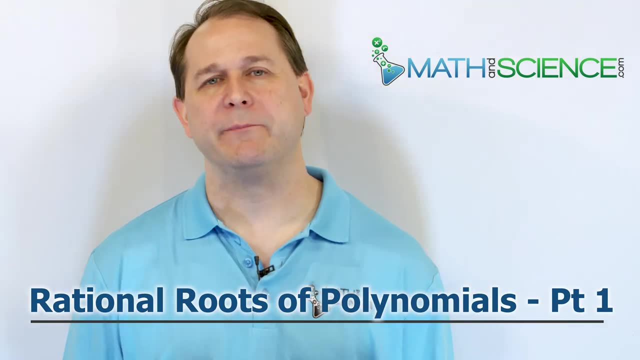 Hello, welcome back to Algebra. The title of this lesson is called Finding Rational Roots of Polynomials, Part 1.. I could also title this the Rational Root Theorem, Part 1.. It's a really important theorem of algebra. Again, we're talking mostly about 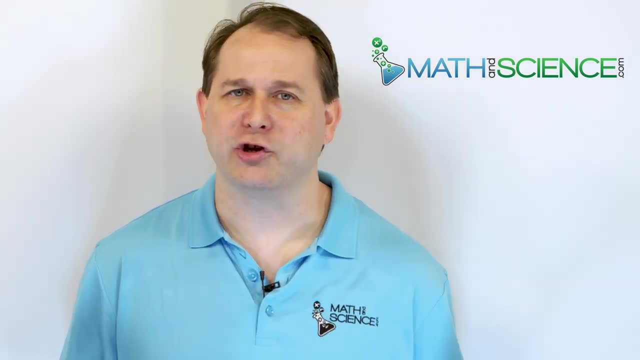 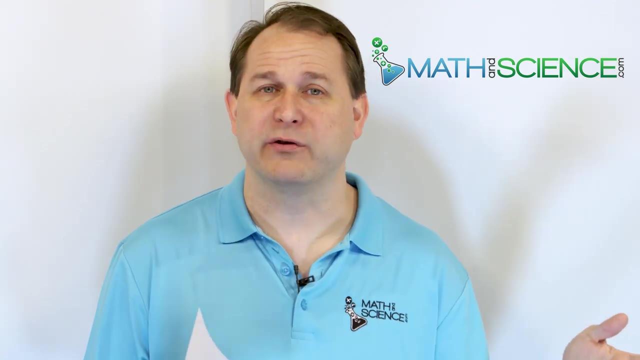 solving polynomials. You all know that we can solve quadratic polynomials just fine. Oftentimes we can solve cubic polynomials if we can guess one of the roots and then we remember we did it when we learned the factor theorem. We can divide that root in to find what's left over. 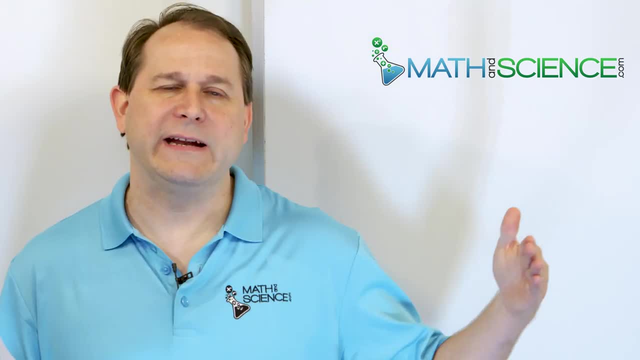 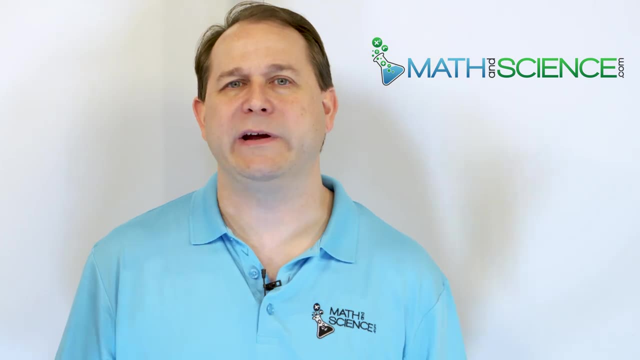 and solve what's left over and find the other two. But when you start getting into higher order polynomials, like fifth and sixth order polynomials, we don't have good tools to find all of those roots. concretely, We did learn in the last lesson Descartes' Rule of Signs, which tells us: 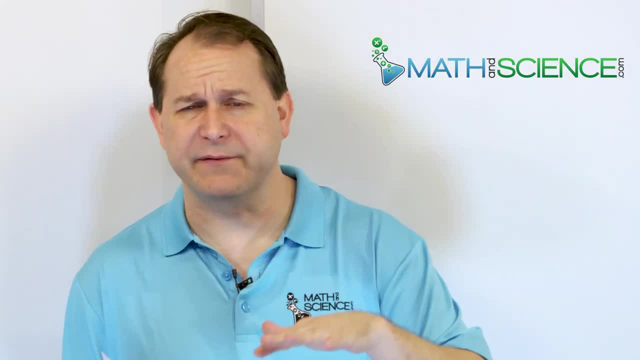 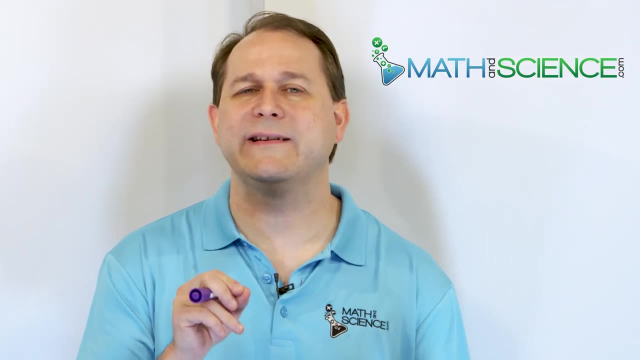 the different possibilities we have for the positive and the negative in the complex roots, but it didn't help us actually find the roots. Here's the other half of that. We're going to learn a technique to help us start to find some of the roots of these higher order. 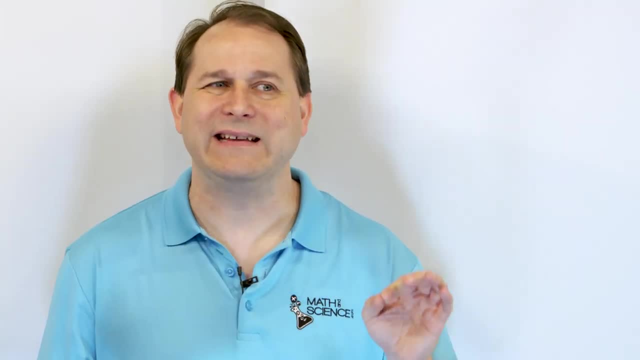 polynomials. We're going to learn a technique to help us start to find some of the roots of these higher order polynomials, and it still doesn't get us all the way there, but at least it gets us pretty close, All right. so this is called the rational root theorem and the reason that it's. 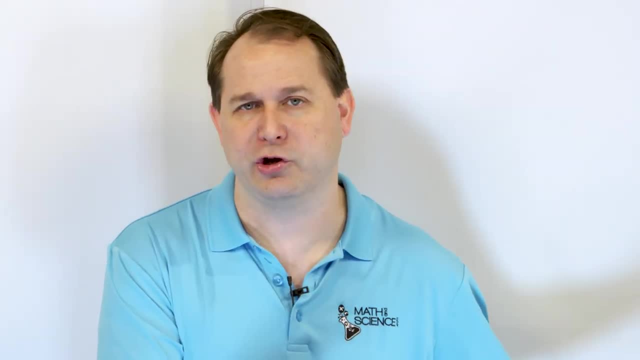 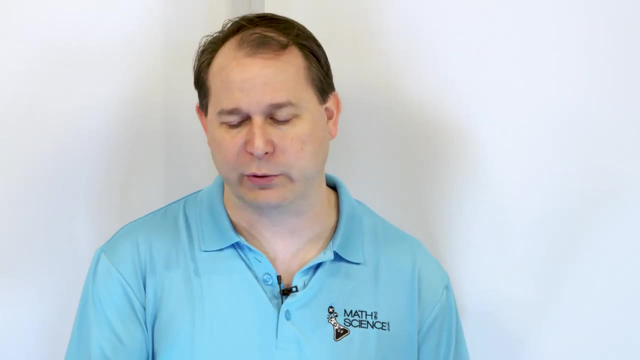 called. that is because it helps us find the rational roots of polynomials. It doesn't help us find the complex roots, It doesn't help us find the irrational roots, It just helps us find the rational roots. So let's review for a quick second that you are with me and you understand. 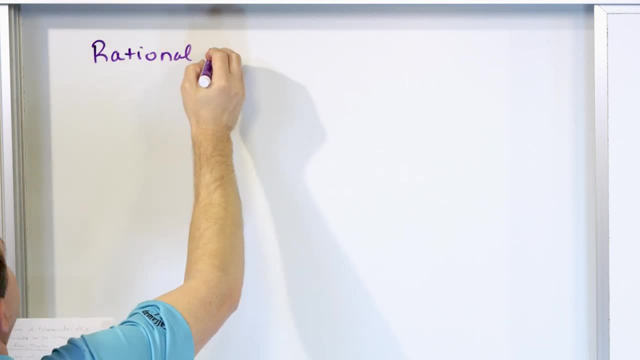 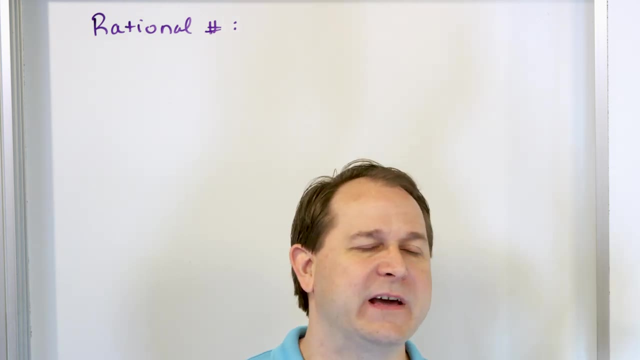 what a rational number is. Basically, a rational number is the number of roots of a polynomial. A rational number, as you've learned before, is just a number, any number that can be written as a fraction. If it can be written as a fraction, it can be written. it is called a rational number. 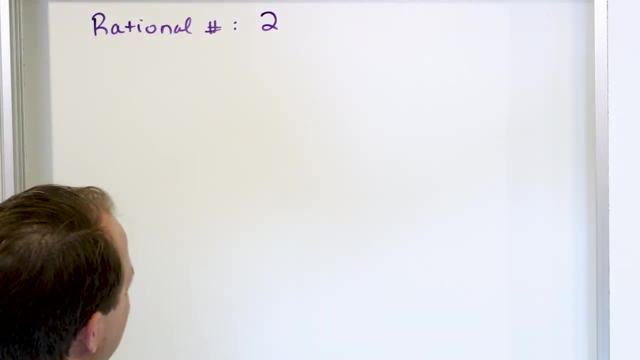 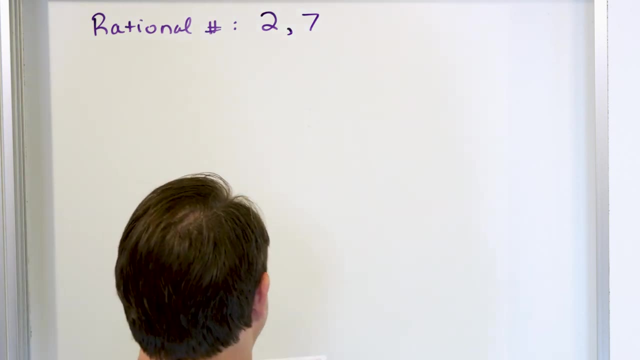 right. So the number 2 is actually a rational number. Why? Well, because you can write 2 as 2 over 1.. You can write that as a fraction, so it's a rational number. The number 7 is a rational. 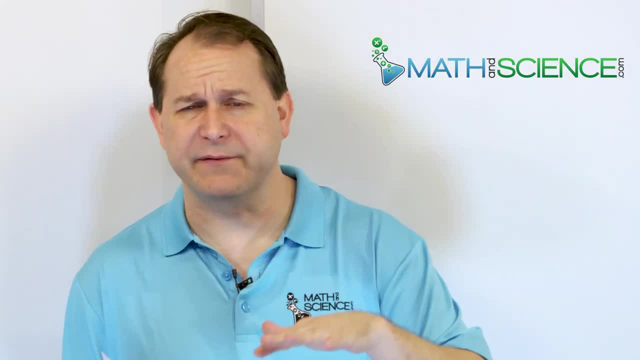 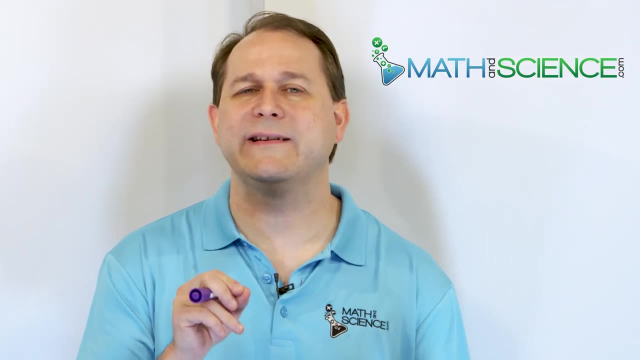 the different possibilities we have for the positive and the negative in the complex roots, but it didn't help us actually find the roots. Here's the other half of that. We're going to learn a technique to help us start to find some of the roots of these higher order. 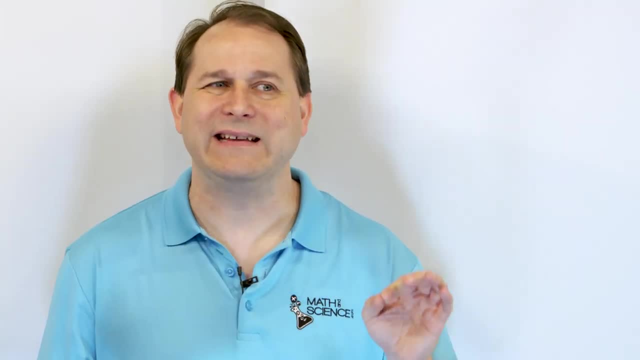 polynomials. We're going to learn a technique to help us start to find some of the roots of these higher order polynomials, and it still doesn't get us all the way there, but at least it gets us pretty close, All right. so this is called the rational root theorem and the reason that it's. 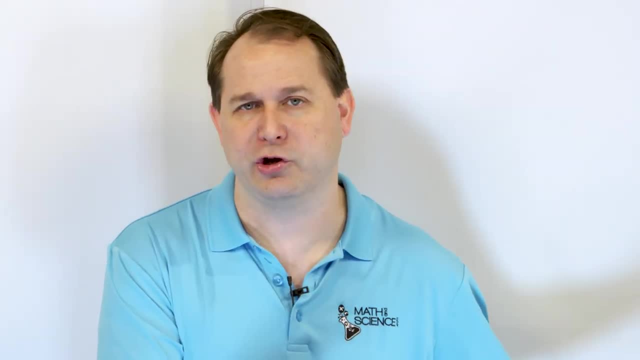 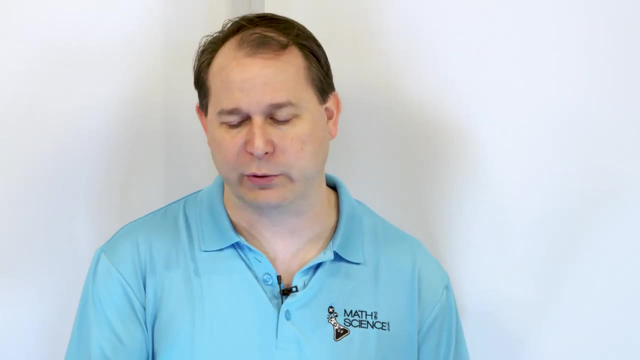 called. that is because it helps us find the rational roots of polynomials. It doesn't help us find the complex roots, It doesn't help us find the irrational roots, It just helps us find the rational roots. So let's review for a quick second that you are with me and you understand. 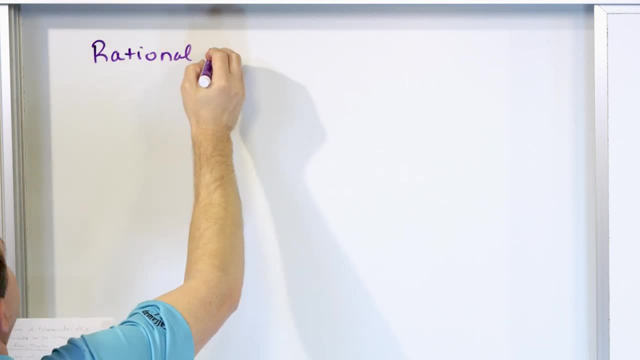 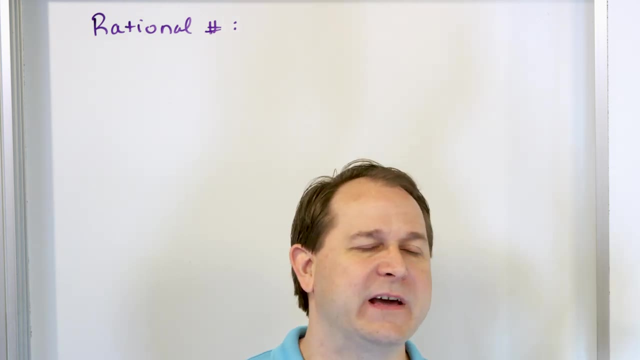 what a rational number is. Basically, a rational number is the number of roots of a polynomial. A rational number, as you've learned before, is just a number, any number that can be written as a fraction. If it can be written as a fraction, it can be written. it is called a rational number. 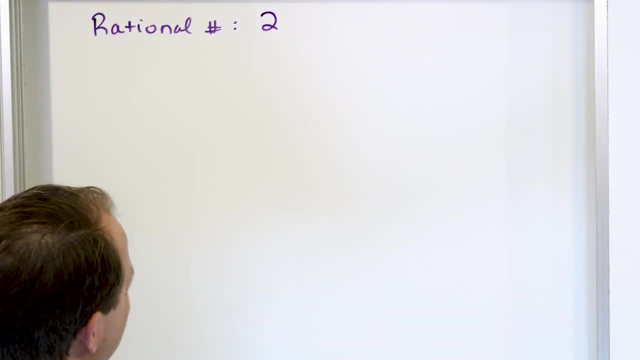 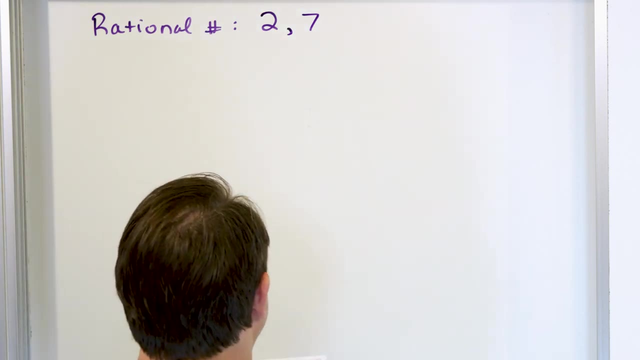 right. So the number 2 is actually a rational number. Why? Well, because you can write 2 as 2 over 1.. You can write that as a fraction, so it's a rational number. The number 7 is a rational. 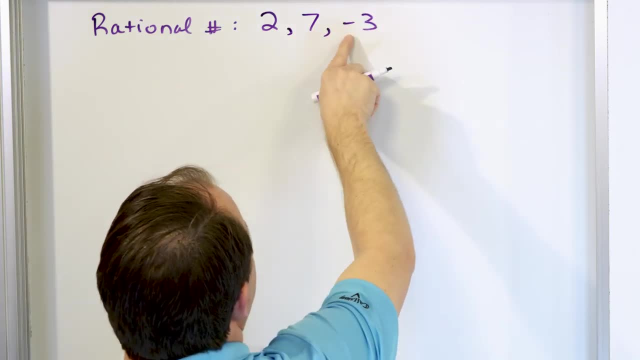 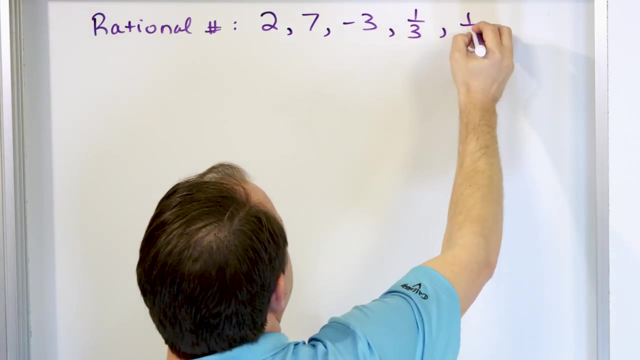 number, The number negative 3 is a rational number. Why? Because I can write it as negative: 3 over 1, right. And then of course you have the actual fractions. That's obviously written as a fraction, so it's a rational number: one half negative, one half. whatever Positive, negative doesn't. 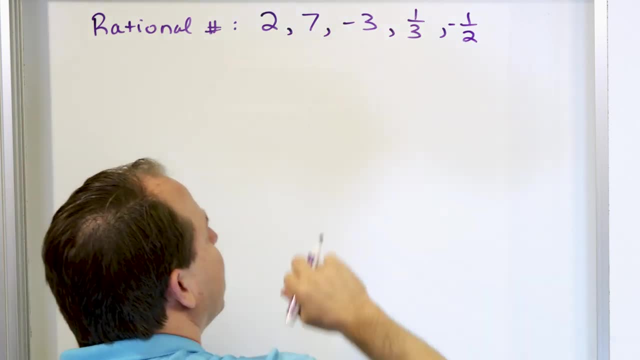 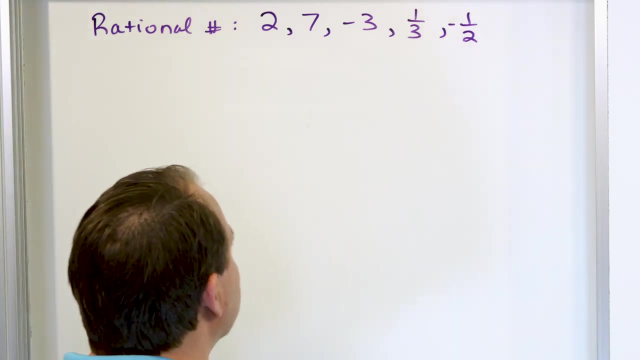 matter as long as it can be written as a fraction. So any whole number that you can think of can be written, as it is a rational number. Any fraction, of course, is a rational number. So most numbers are rational to some degree or other, But we have, of course, other numbers that we have learned. 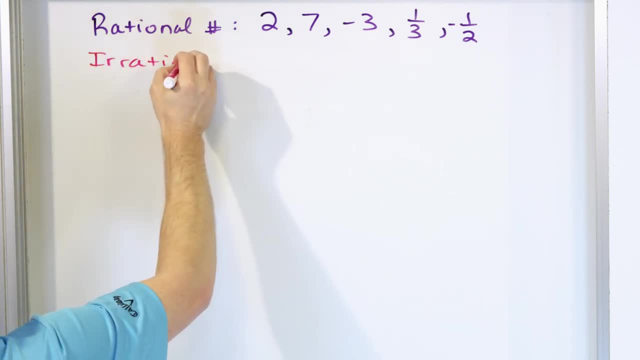 about called irrational numbers, And those are special numbers like pi. This number goes on and on and on. The decimal never repeats, And so you cannot write pi as a fraction. I should say you can't write pi as a fraction of whole numbers When I say you can write these as a fraction. 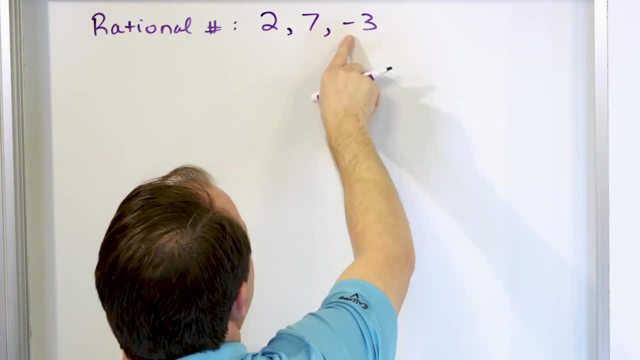 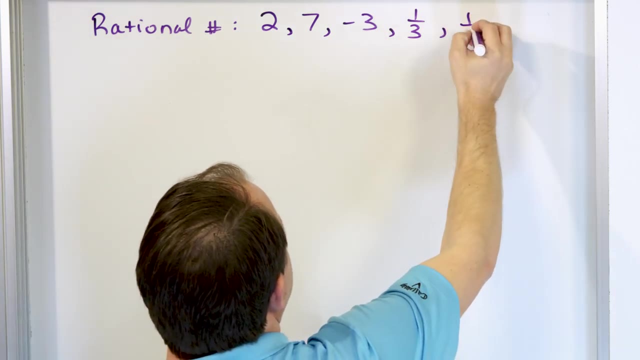 number, The number negative 3 is a rational number. Why? Because I can write it as negative: 3 over 1, right. And then of course you have the actual fractions. That's obviously written as a fraction, so it's a rational number: one half negative, one half. whatever Positive, negative doesn't. 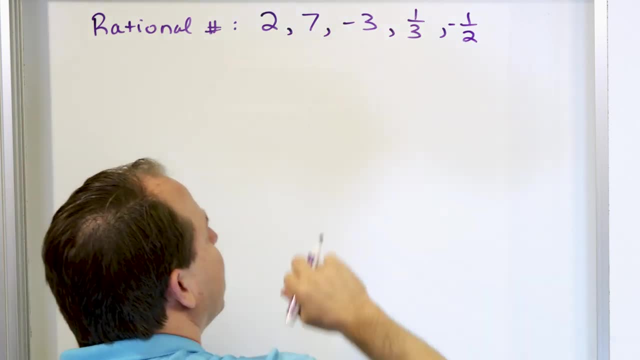 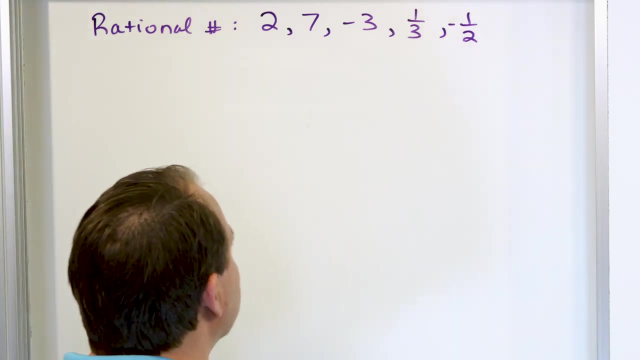 matter as long as it can be written as a fraction. So any whole number that you can think of can be written, as it is a rational number. Any fraction, of course, is a rational number. So most numbers are rational to some degree or other, But we have, of course, other numbers that we have learned. 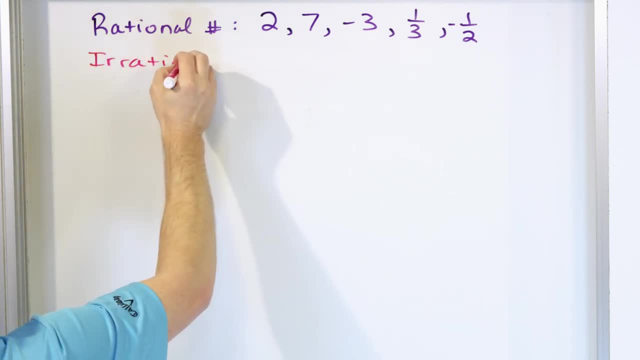 about called irrational numbers, And those are special numbers like pi. This number goes on and on and on. The decimal never repeats, And so you cannot write pi as a fraction. I should say you can't write pi as a fraction of whole numbers When I say you can write these as a fraction. 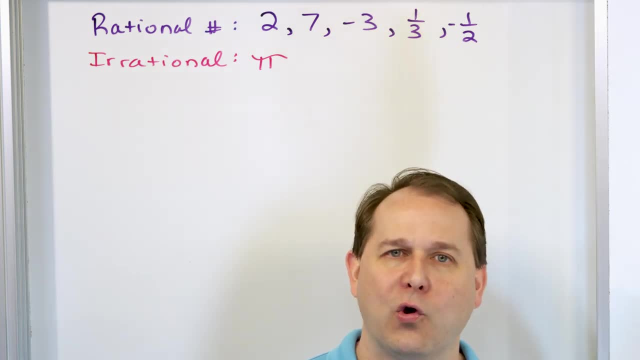 I'm saying can we write them as a fraction of whole numbers? Pi, of course, is the ratio of a circle's circumference and diameter, But those are not going to ever be whole numbers to give you pi. You're not going to be able to get pi by dividing two whole numbers. Some people say 22 over 7 is. 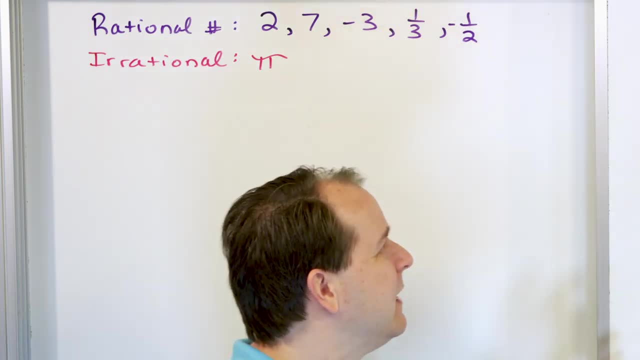 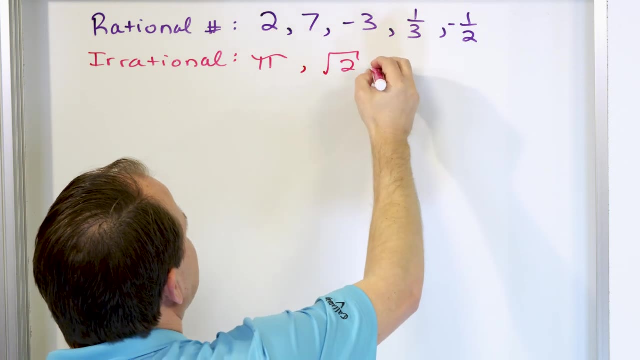 pretty close to pi. That's true, It's pretty close, But it's not equal to pi, right? Some other examples: Square root of 2.. You know we've gotten roots that are square root of 2 or minus square root of 2 in these polynomials. These are irrational Square root of 3.. I can go on and. 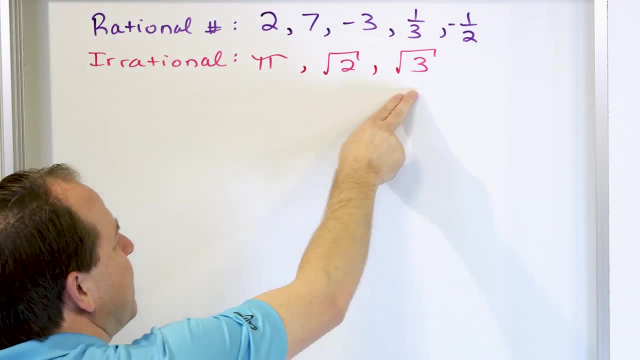 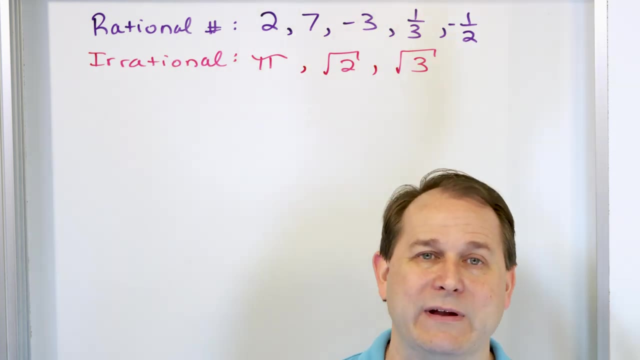 on, Lots of radicals end up becoming irrational. If I put these numbers in a calculator, or their negative counterparts, like negative square root of 3, the decimals are going to go on and on forever. They're never going to end, And when that happens, you cannot write those numbers as. 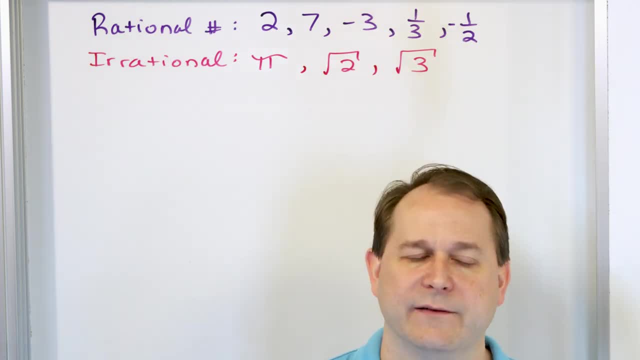 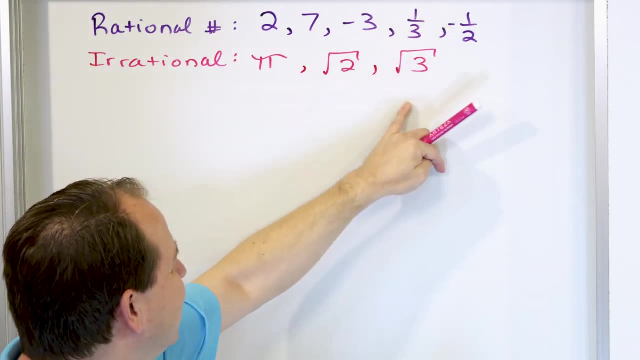 fractions, So they're irrational, So they're different, slightly different class of numbers. The rational root theorem that we're going to talk about does not help us figure out roots that are radicals like this or pi or anything like that. It doesn't help. 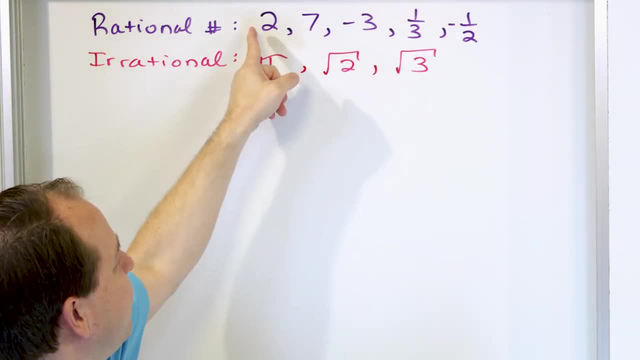 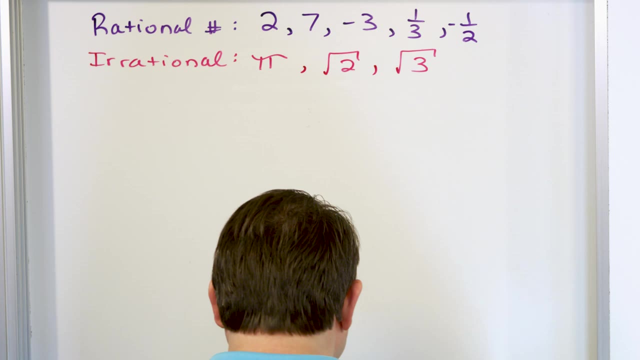 us with that. It doesn't help us with complex numbers, It just helps us figure out what roots we have. that can be written as a fraction, But that turns out to be a pretty common thing, So it is very useful, All right. So we have to first talk about this theorem And then we're going to do a 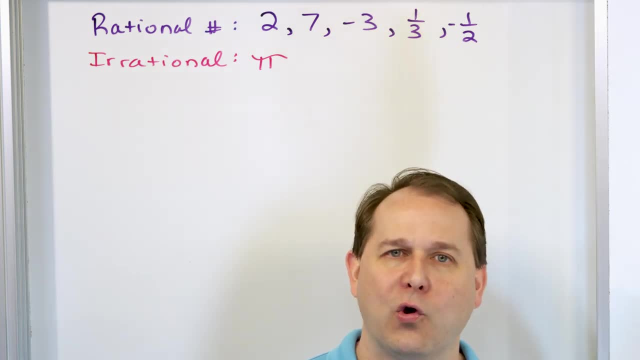 I'm saying can we write them as a fraction of whole numbers? Pi, of course, is the ratio of a circle's circumference and diameter, But those are not going to ever be whole numbers to give you pi. You're not going to be able to get pi by dividing two whole numbers. Some people say 22 over 7 is. 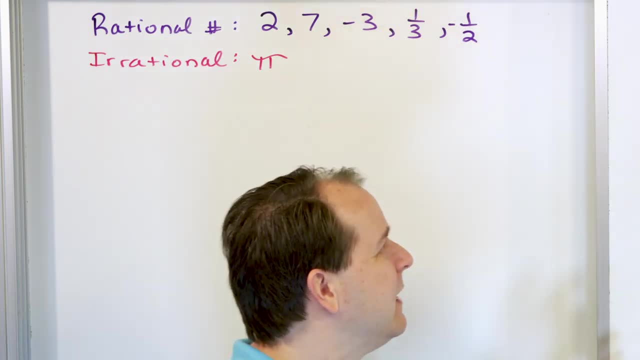 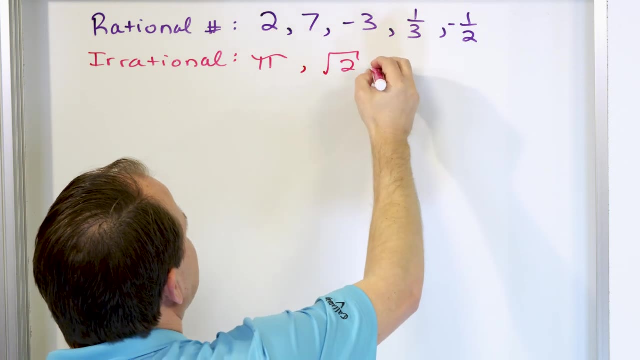 pretty close to pi. That's true, It's pretty close, But it's not equal to pi, right? Some other examples: Square root of 2.. You know we've gotten roots that are square root of 2 or minus square root of 2 in these polynomials. These are irrational Square root of 3.. I can go on and. 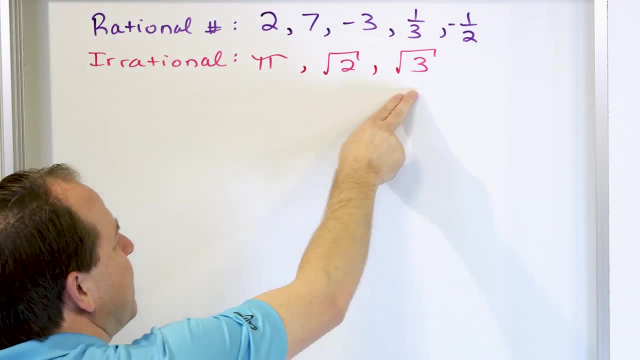 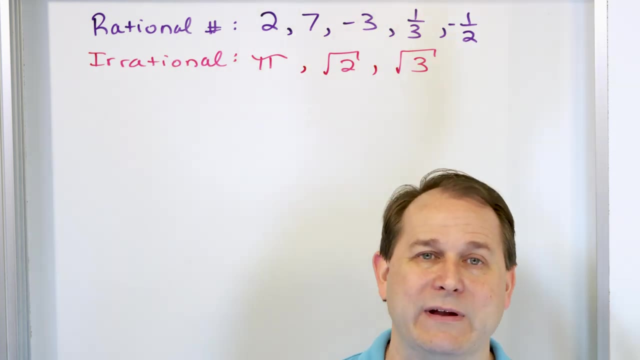 on, Lots of radicals end up becoming irrational. If I put these numbers in a calculator, or their negative counterparts, like negative square root of 3, the decimals are going to go on and on forever. They're never going to end, And when that happens, you cannot write those numbers as. 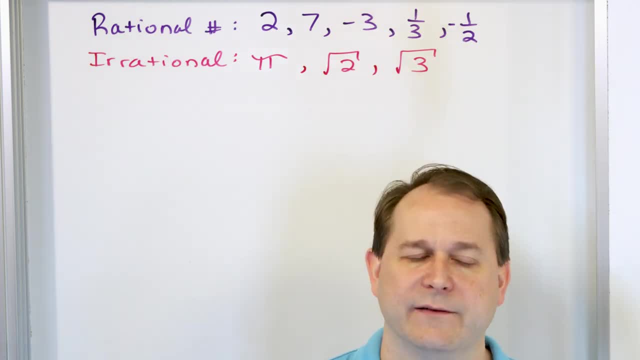 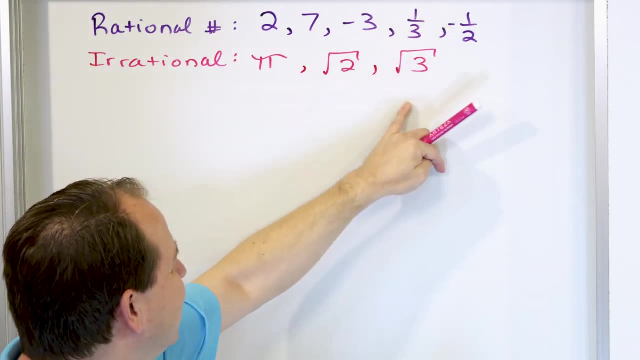 fractions, So they're irrational, So they're different, slightly different class of numbers. The rational root theorem that we're going to talk about does not help us figure out roots that are radicals like this or pi or anything like that. It doesn't help. 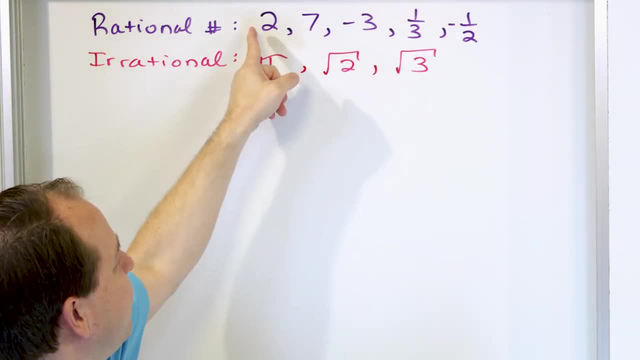 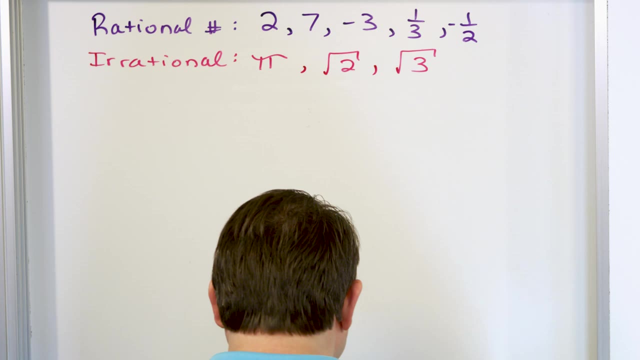 us with that. It doesn't help us with complex numbers, It just helps us figure out what roots we have. that can be written as a fraction, But that turns out to be a pretty common thing, So it is very useful, All right. So we have to first talk about this theorem And then we're going to do a 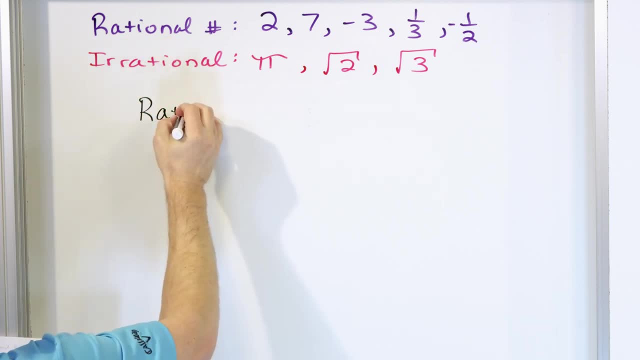 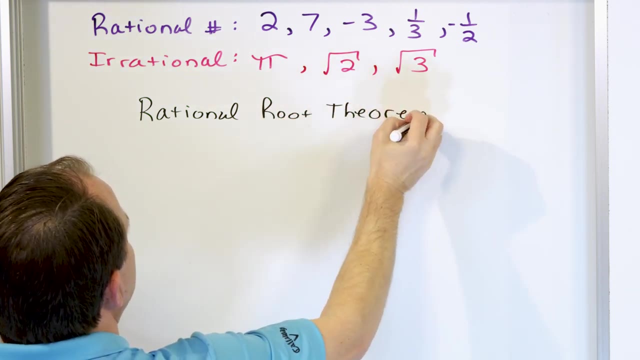 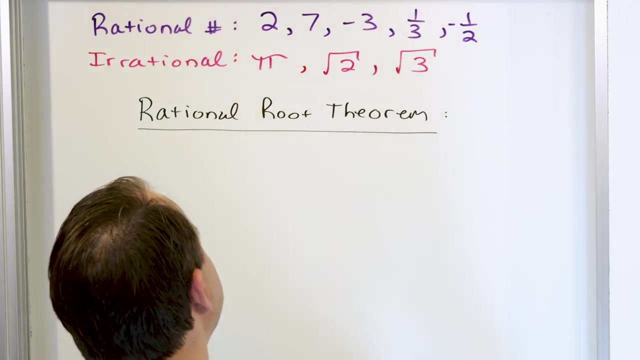 problem to show you how to use it. So this thing is called the rational root theorem, Really important, especially as you get higher up in terms of higher order polynomials, because we don't have concrete ways of finding the roots of those higher order ones. 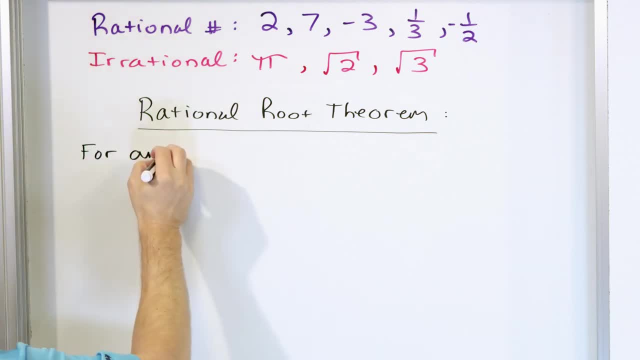 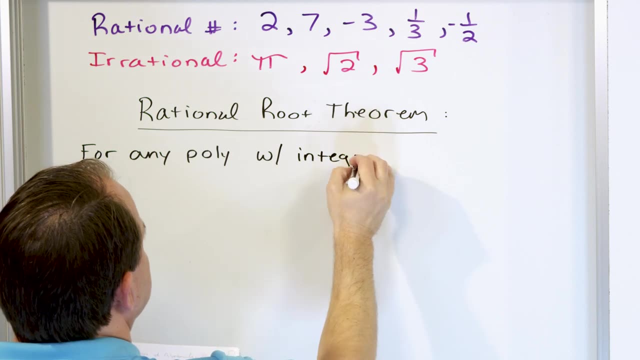 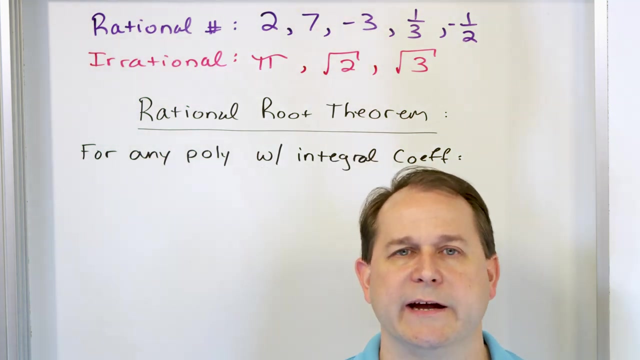 So the theorem goes like this: For any polynomial with integral coefficients- What do I mean by integral I'm talking about- the polynomial itself has to have, you know, 1, negative, 2, negative, 5. That's coefficients. The polynomial can't have 1 half as a coefficient or 1 seventh as a coefficient. But any polynomial 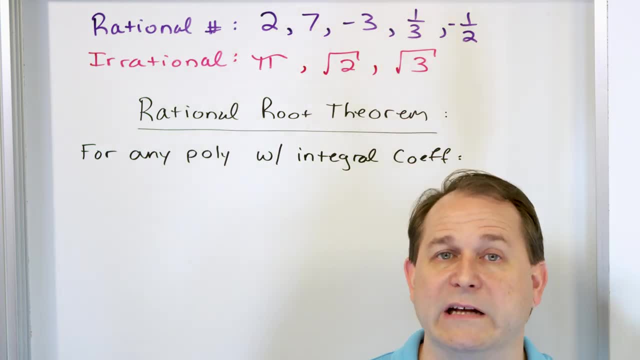 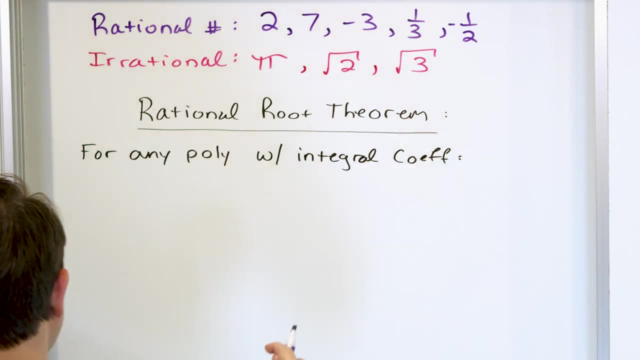 that you have with fractional coefficients. you can just multiply through the whole thing and clear any of those fractions out, So you can always get it into the form of a polynomial with integral coefficients. So let's give an example of a polynomial like this, So, for example, a polynomial with integral. 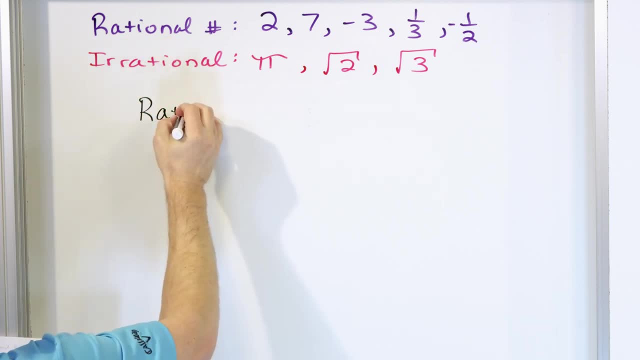 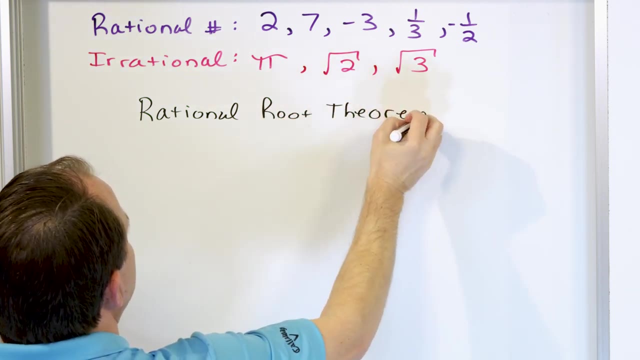 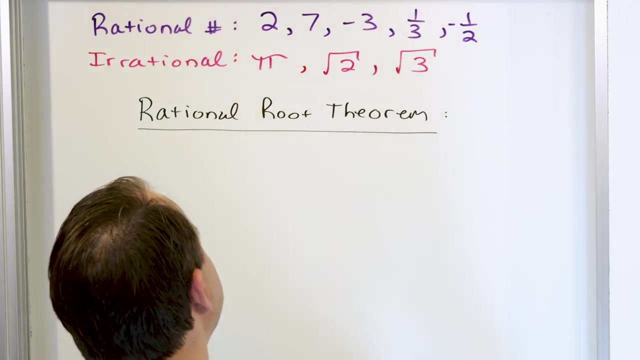 problem to show you how to use it. So this thing is called the rational root theorem, Really important, especially as you get higher up in terms of higher order polynomials, because we don't have concrete ways of finding the roots of those higher order ones. 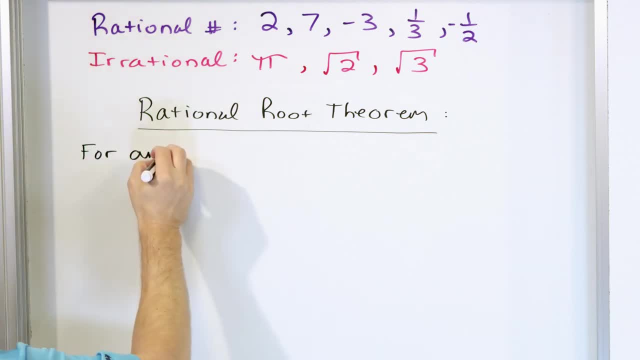 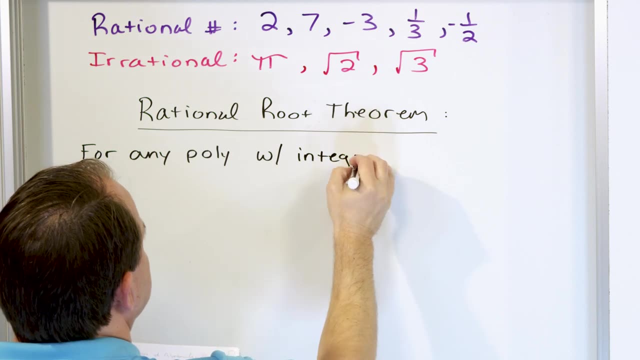 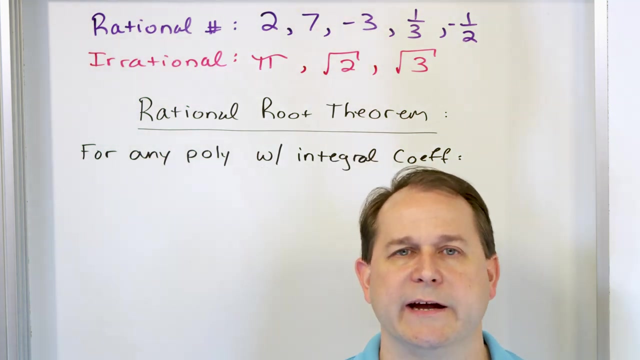 So the theorem goes like this: For any polynomial with integral coefficients- What do I mean by integral I'm talking about- the polynomial itself has to have, you know, 1, negative, 2, negative, 5. That's coefficients. The polynomial can't have 1 half as a coefficient or 1 seventh as a coefficient. But any polynomial 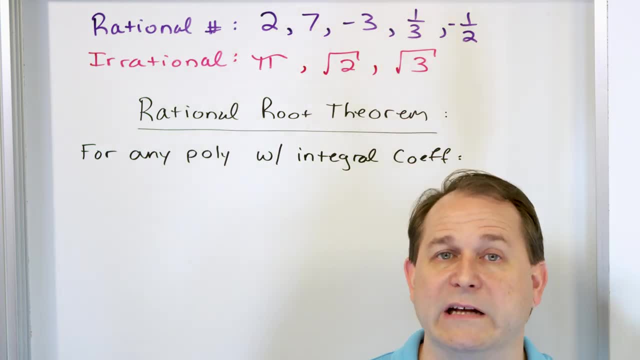 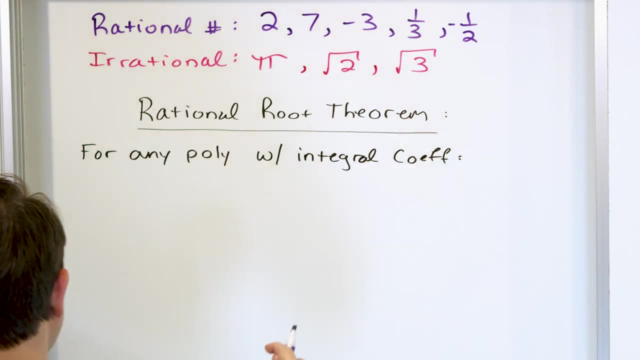 that you have with fractional coefficients. you can just multiply through the whole thing and clear any of those fractions out, So you can always get it into the form of a polynomial with integral coefficients. So let's give an example of a polynomial like this, So, for example, a polynomial with integral. 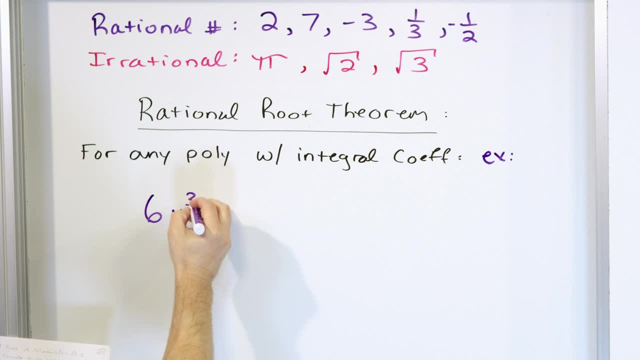 coefficients like this might be 6x cubed plus 7x squared, minus 7x minus 7x squared. So we might want to find the roots of this equation. We know we're going to have three of them And I'm using a third order just to show you what we're doing, But this whole 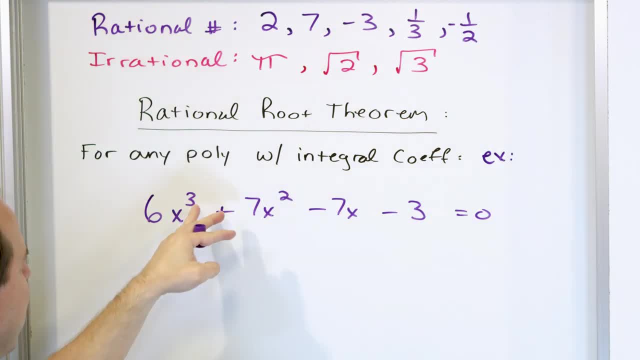 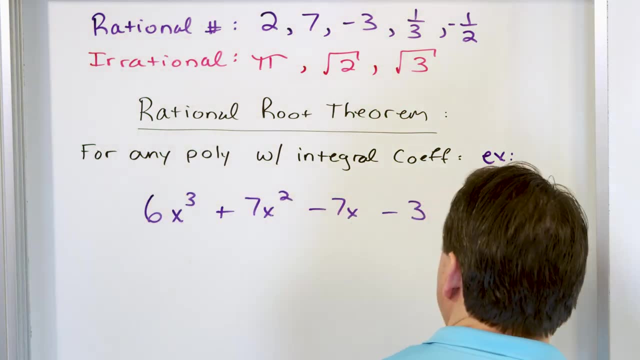 process works for any order of polynomial. You could have a tenth order or a fifteenth order or a thirty-ninth order polynomial. I hope you never have to deal with anything like that, But of course it works for anything. Integral coefficients Why? Because 6,, 7,. 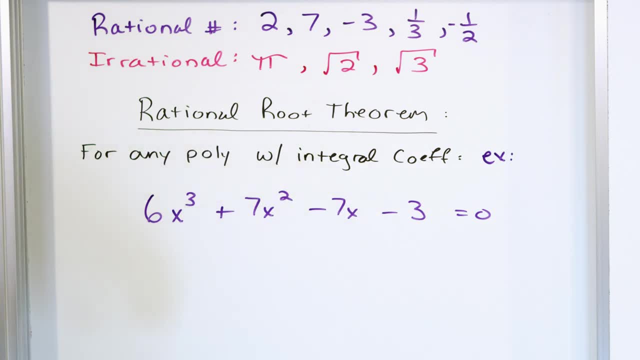 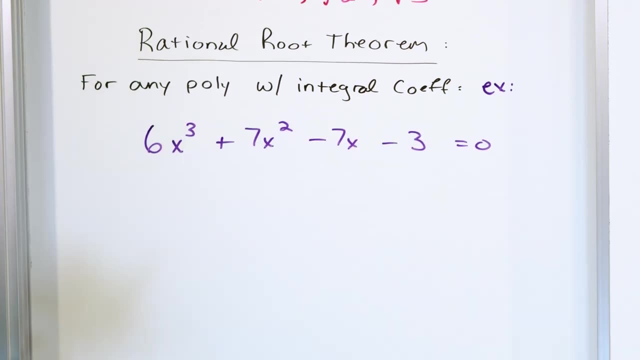 negative 7, and negative 3,. they're all whole numbers, They're not fractions. Well, you can write them as 6 over 1, but I'm saying there's no obvious fractions, They're all whole numbers, like this: 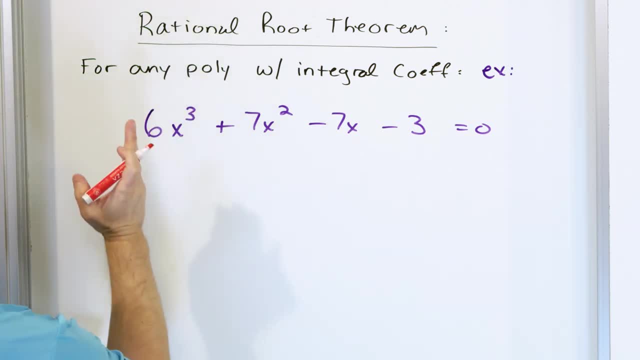 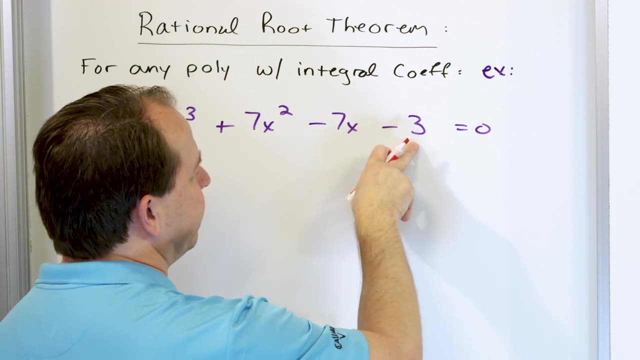 Now what we have to do to figure out how to use this rational root theorem. it all boils down to looking at the coefficient of the highest term, in this case x, cubed, and the coefficient of the lowest term, which means the constant term, negative 3 in this case. 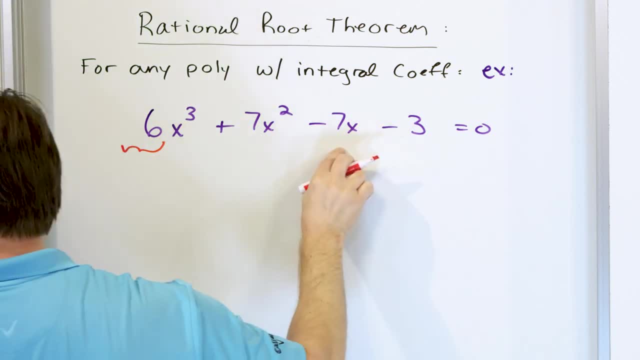 So we have special names for this. So this we're basically for the purpose of this theorem. we're going to basically ignore everything in the middle there, Because we're dealing with anything in the middle of the polynomial. we have special names for these guys, So we're. 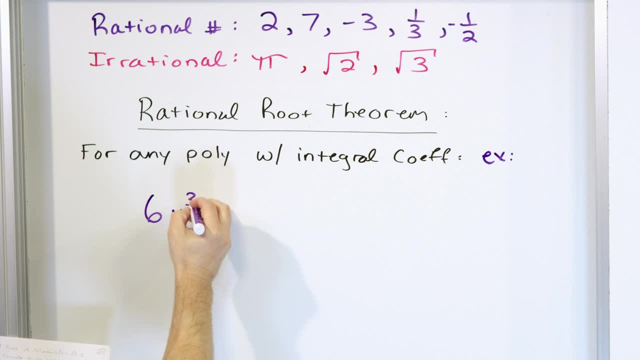 coefficients like this might be 6x cubed plus 7x squared, minus 7x minus 7x squared. So we might want to find the roots of this equation. We know we're going to have three of them And I'm using a third order just to show you what we're doing, But this whole 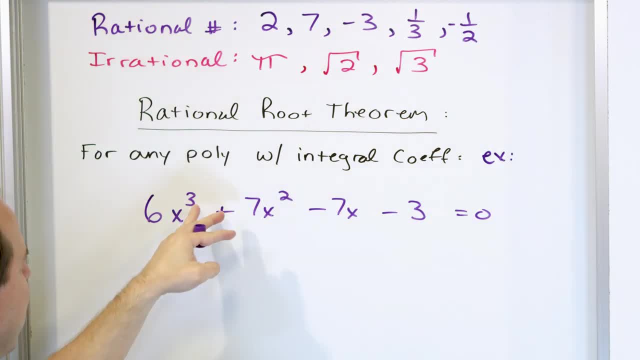 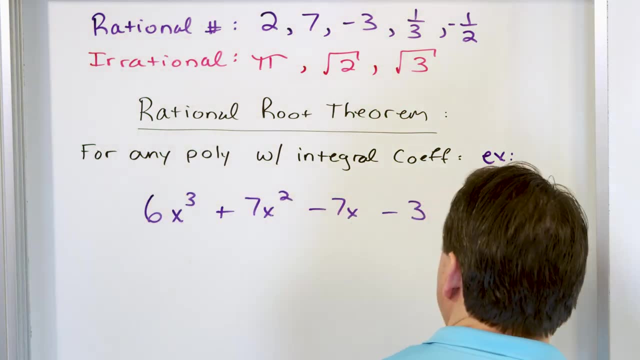 process works for any order of polynomial. You could have a tenth order or a fifteenth order or a thirty-ninth order polynomial. I hope you never have to deal with anything like that, But of course it works for anything. Integral coefficients Why? Because 6,, 7,. 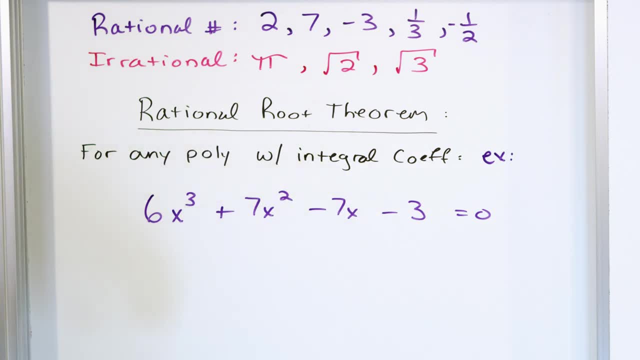 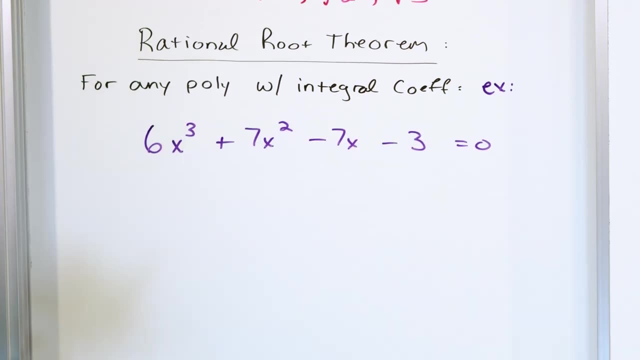 negative 7, and negative 3,. they're all whole numbers, They're not fractions. Well, you can write them as 6 over 1, but I'm saying there's no obvious fractions, They're all whole numbers, like this: 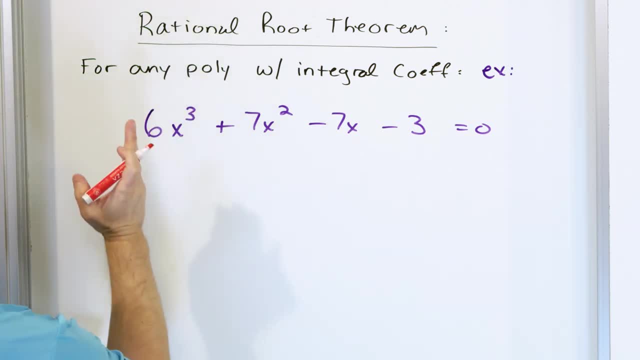 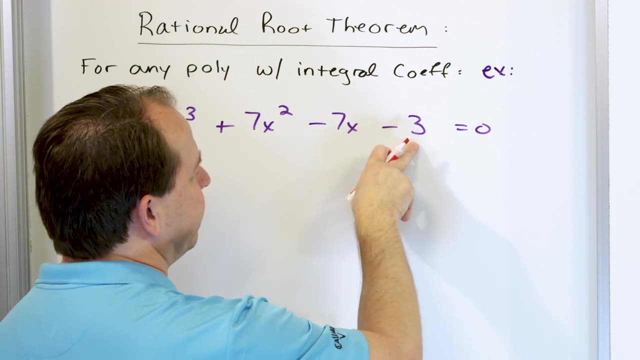 Now what we have to do to figure out how to use this rational root theorem. it all boils down to looking at the coefficient of the highest term, in this case x, cubed, and the coefficient of the lowest term, which means the constant term, negative 3 in this case. 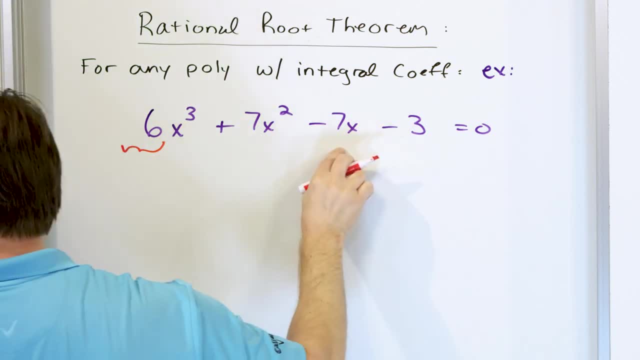 So we have special names for this. So this we're basically for the purpose of this theorem. we're going to basically ignore everything in the middle there, Because we're dealing with anything in the middle of the polynomial. we have special names for these guys, So we're. 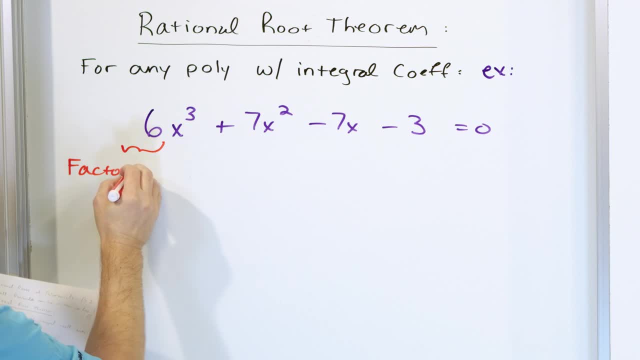 going to end up finding the factors of the leading coefficient, And we call these coefficients up here, we call them k, You'll see why, because there's a whole list of them, So we're not going to care about anything in the middle of the polynomial, only the first term, and 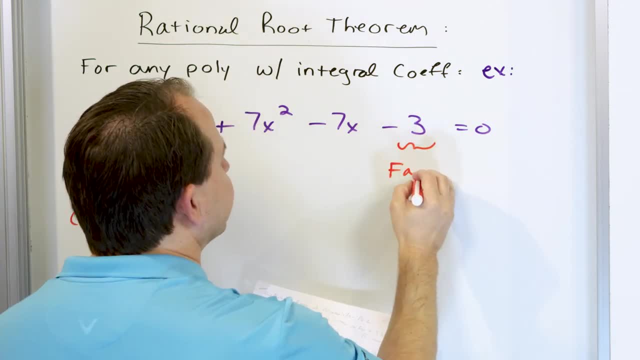 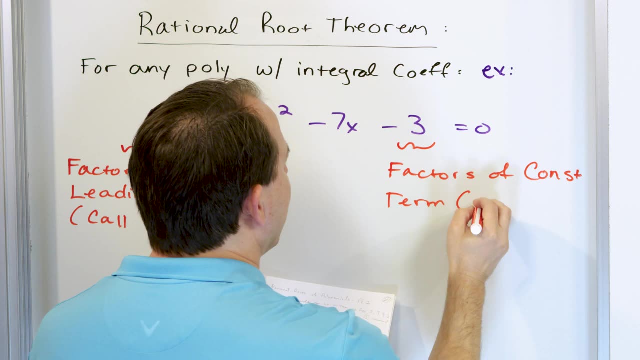 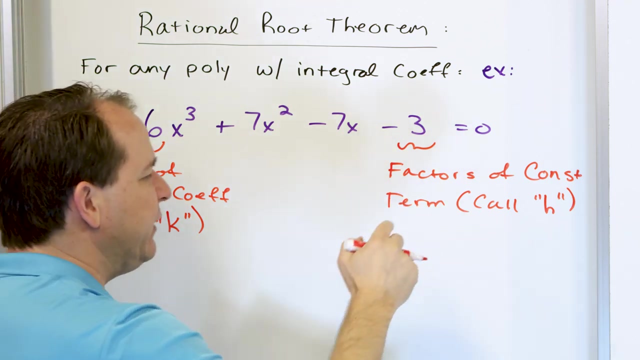 the last term. So the last one here: the factors of these, the factors of the constant term. we call these h. Now, your book might not say, or your teacher might not call them k and h, It might call them a and b or whatever, w and z. It doesn't matter, It's just we have to have 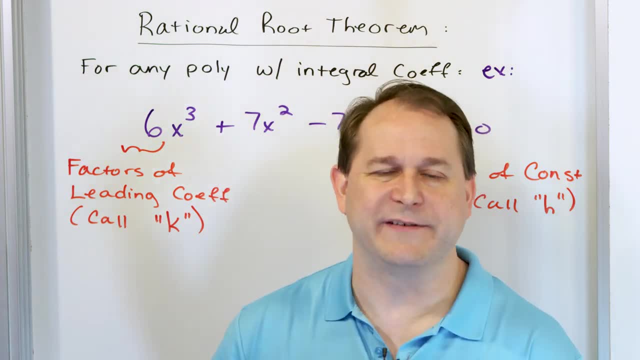 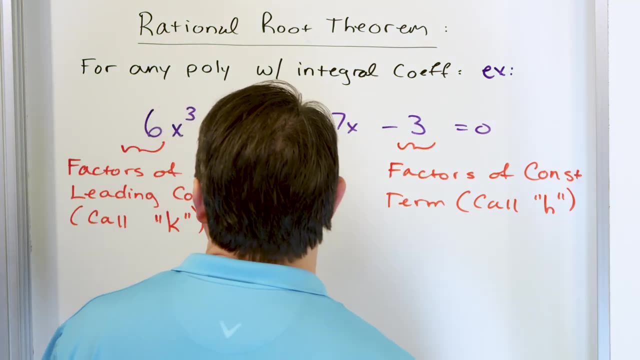 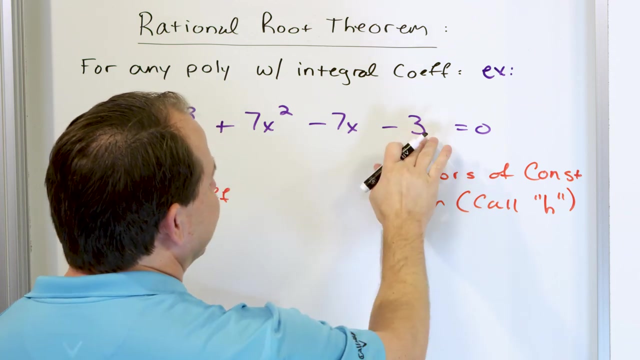 some label. We label all of the factors of the leading term, something, and the factors of the trailing term, something. You'll see why in a second. Let's first of all figure out what the factors of this last term are. This is a negative. 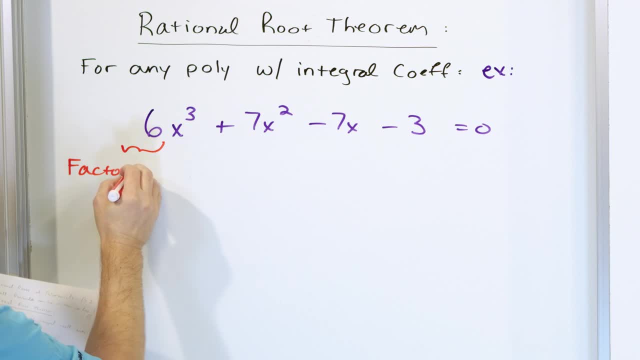 going to end up finding the factors of the leading coefficient, And we call these coefficients up here, we call them k, You'll see why, because there's a whole list of them, So we're not going to care about anything in the middle of the polynomial, only the first term, and 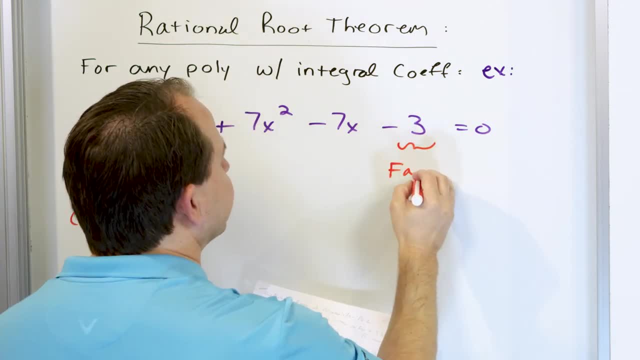 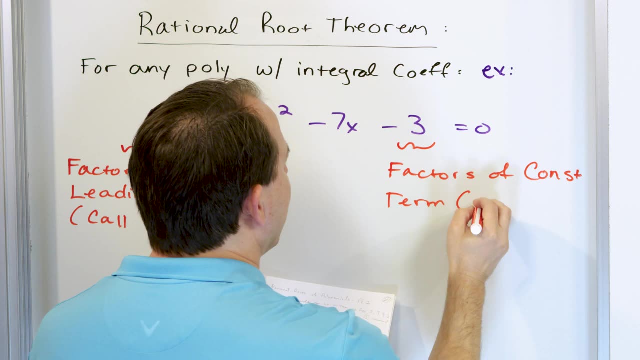 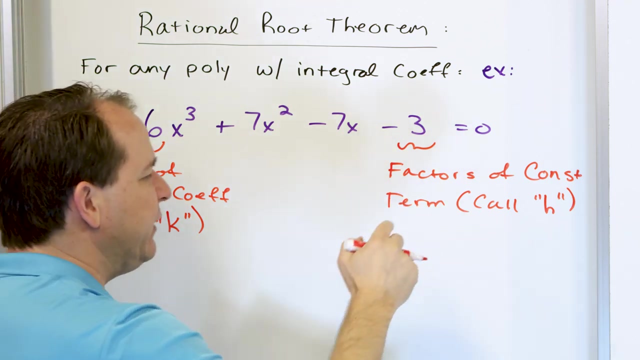 the last term. So the last one here: the factors of these, the factors of the constant term. we call these h. Now, your book might not say, or your teacher might not call them k and h, It might call them a and b or whatever, w and z. It doesn't matter, It's just we have to have 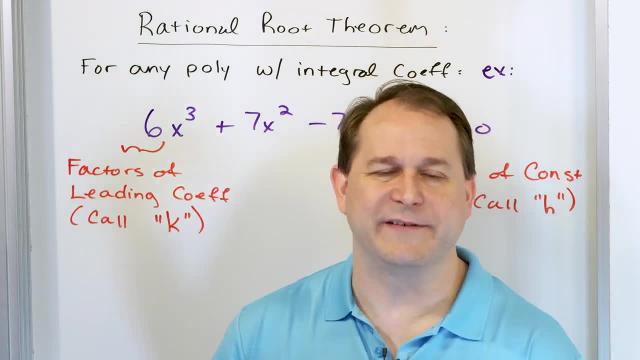 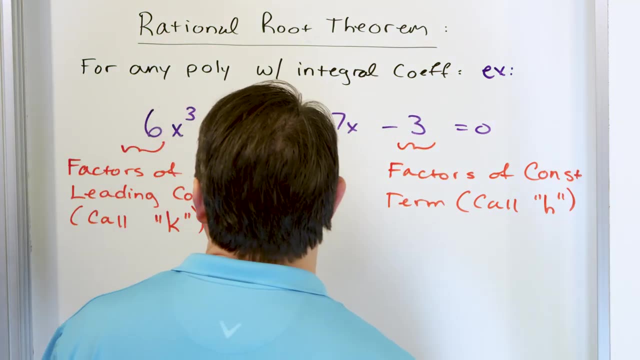 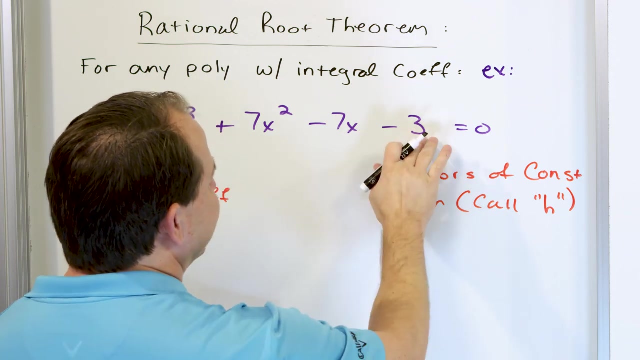 some label. We label all of the factors of the leading term, something, and the factors of the trailing term, something. You'll see why in a second. Because it makes it easier to deal with them. Let's first of all figure out what the factors of this last term are. This is a negative. 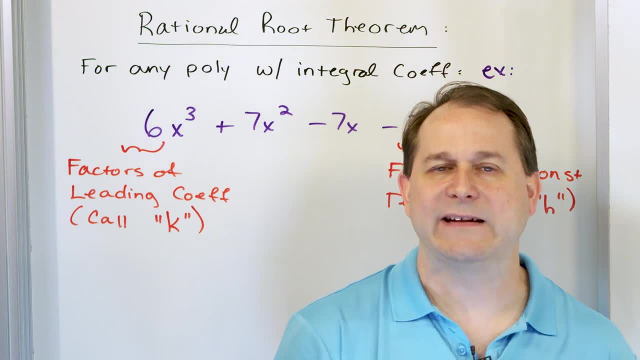 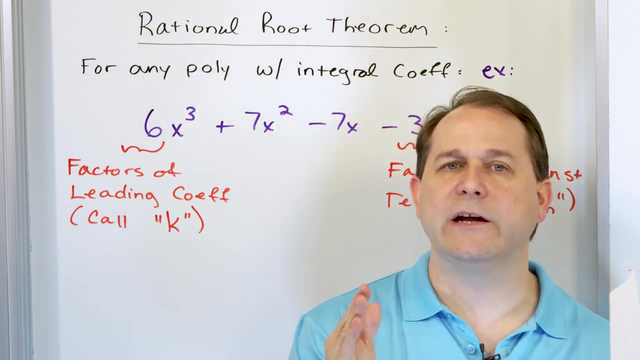 3. Remember what is a factor. anyway, We've been factoring things in algebra forever, but what is a factor? A factor means if you have something you're examining and you want to find the factors of that thing, you need to find all of the things that can multiply. 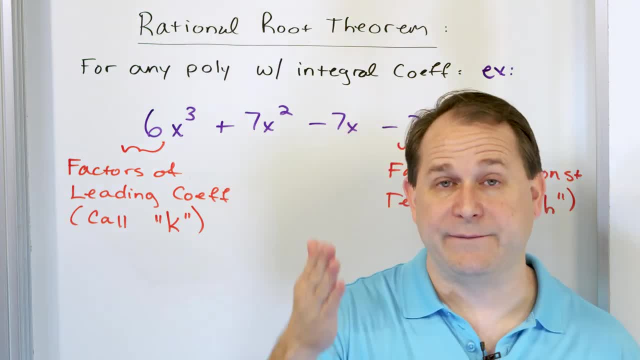 together to give you that thing. And we can typically find all the factors by doing a factor tree. But the number of factors is only going to be 1.. We'll get our answer from the last term because that's the last time we were taking things into respect. But the first thing: 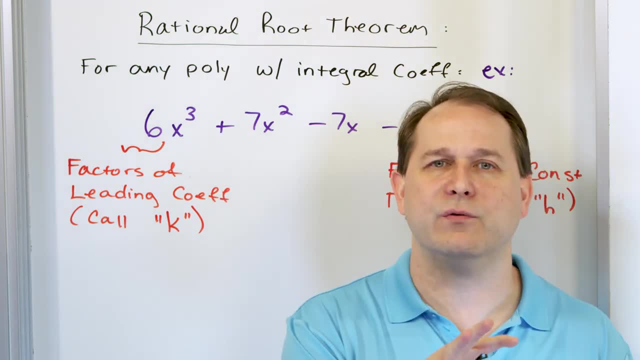 is to find the factors of the last term, Because the number of factors is only going to give us the number of factors. So in the first term we do have to find all the factors. you've been doing it long enough. we don't need to find, we don't need to build a factor tree for 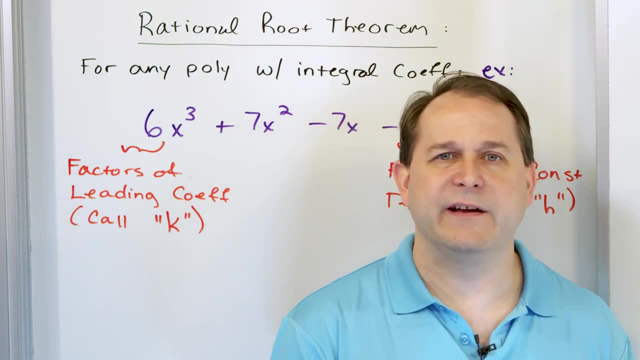 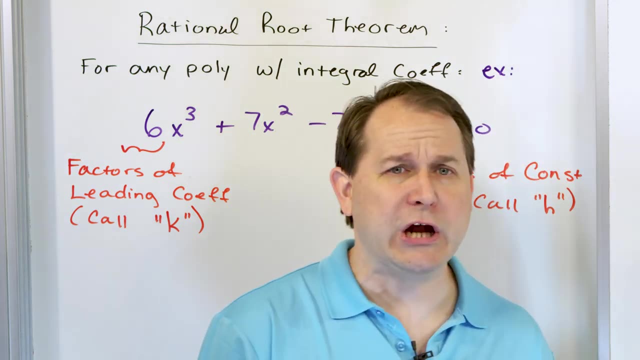 this exercise You're going to find out. it's pretty simple to do. But, for instance, we're going to take a number like three, negative three in this case, and we're going to figure out what are the factors of negative three. Well, we know that one is a factor because one times three is. 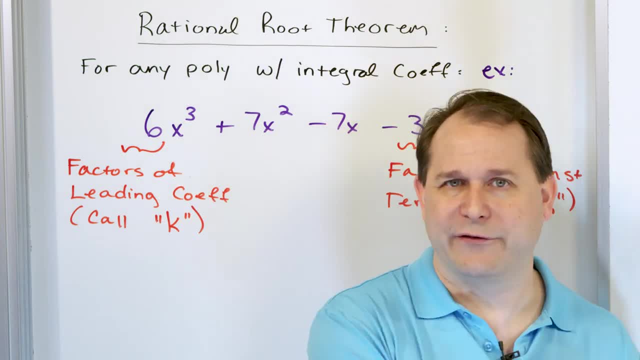 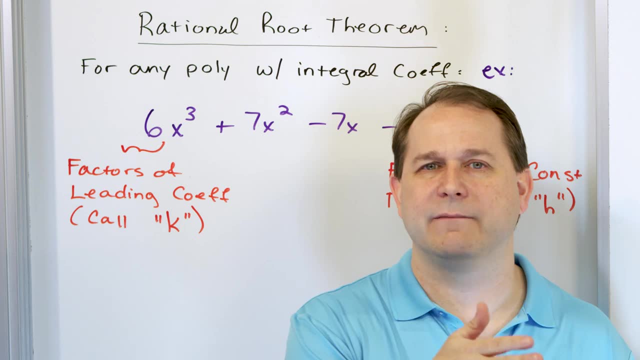 three, And we know that three is a factor. Three times one is three. But other than those two numbers there really are no other numbers. But five, for instance, is not a factor of three, because five times something, nothing really works to give you three And there are no other. 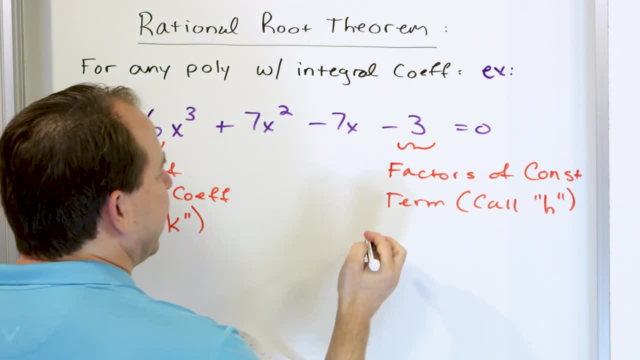 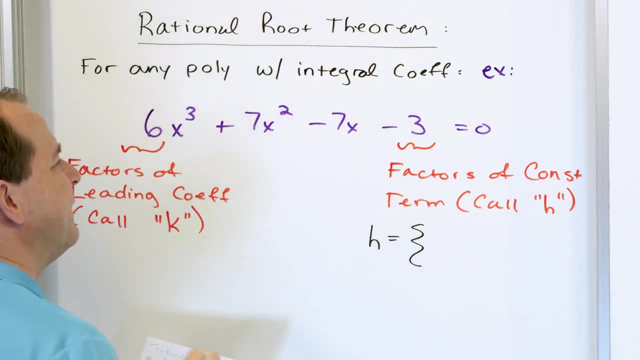 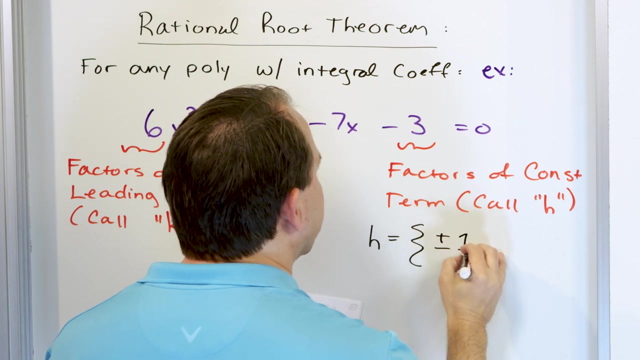 really numbers. So only one and three are factors there, But these factors we're going to call them h. I'm going to open up a little curly brace, which means we have a set of numbers right. So the factors of this last term is not just one and three, it's actually plus or minus one. 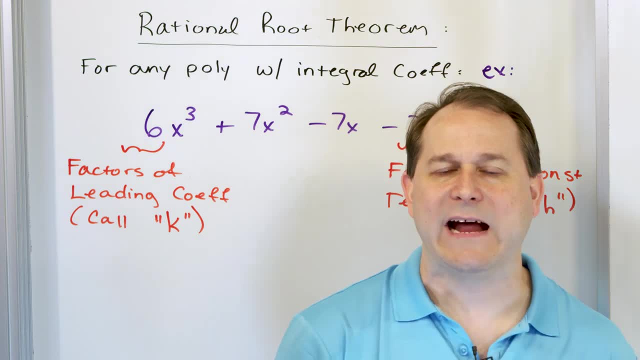 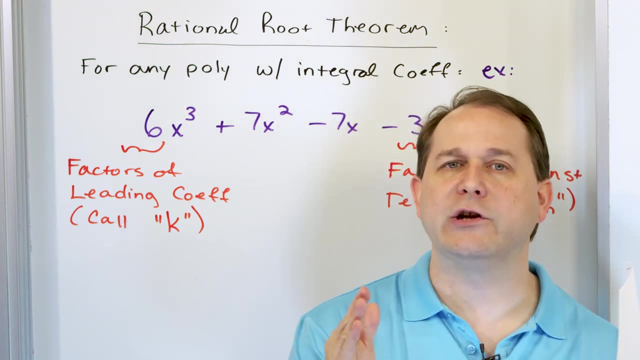 three. Remember what is a factor. anyway, We've been factoring things in algebra forever, But what is a factor? A factor means it's: if you have something you're examining and you want to find the factors of that thing, you need to find all of the things that can. 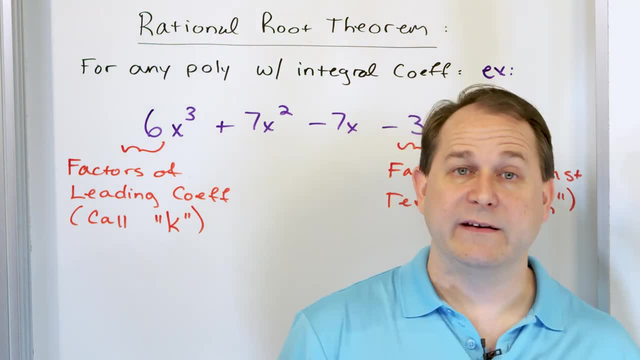 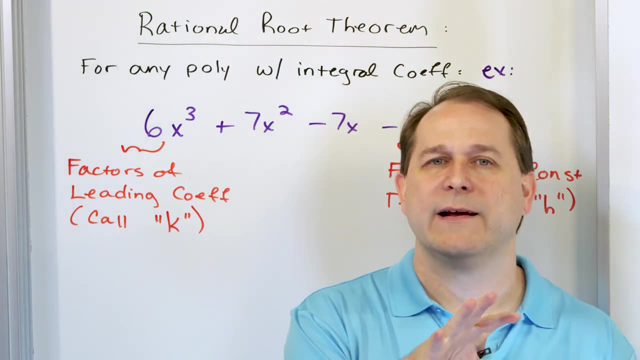 multiply together to give you that thing, And we can typically find all the factors by doing a factor tree. Okay, Okay, you've been doing it long enough, we don't need to find, we don't need to build a factor tree for. 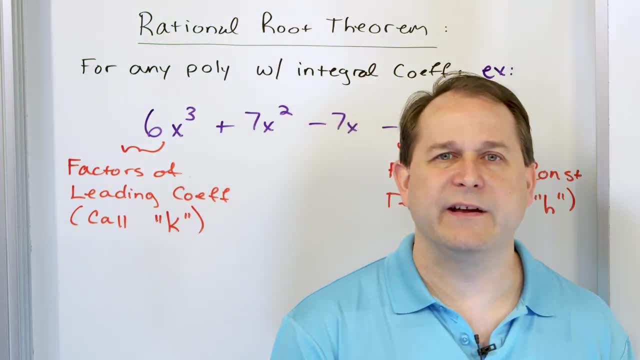 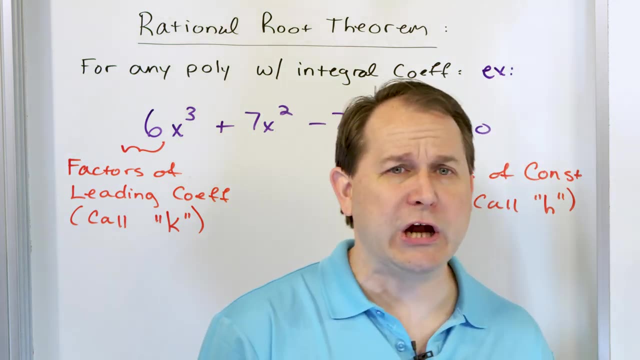 this exercise You're going to find out. it's pretty simple to do. But, for instance, we're going to take a number like three and we're going to negative three in this case, and we're going to figure out what are the factors of negative three. Well, we know that one is a factor because 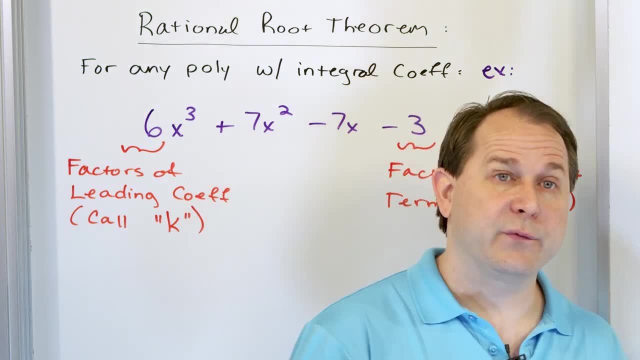 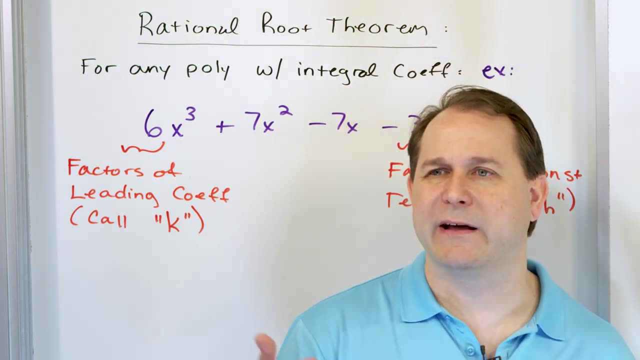 one times three is three, And we know that three is a factor. Three times one is three. But other than those two numbers, there really are no other numbers. But five, for instance, is not a factor of three, because five times something nothing really works to give you three. And there are no. 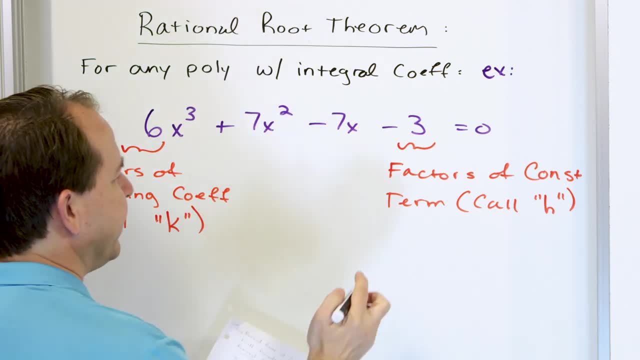 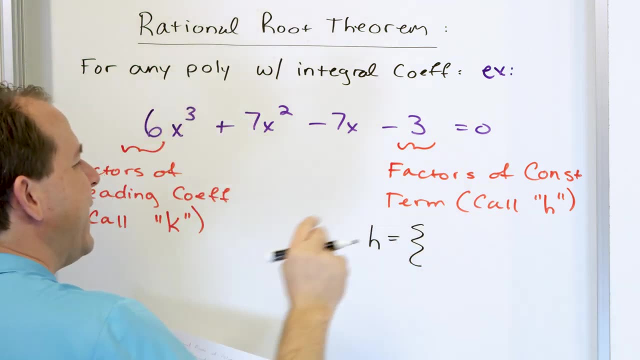 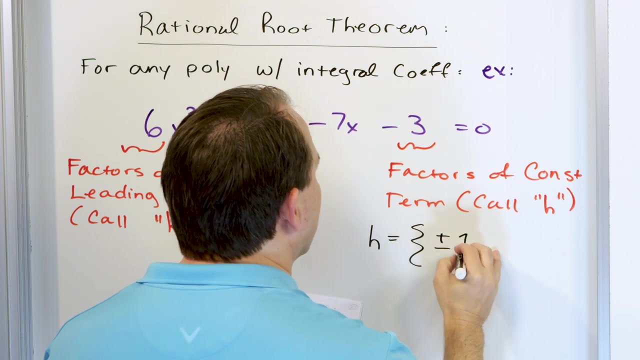 other really numbers. So only one and three are factors there, But these factors we're going to call them h. I'm going to open up a little curly brace, which means we have a set of numbers. So the factors of this last term is not just one and three, it's actually plus or minus one. 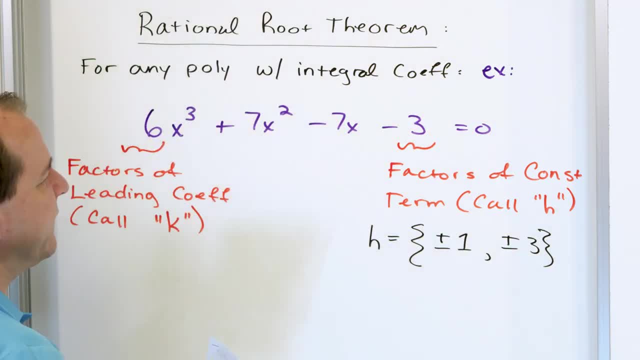 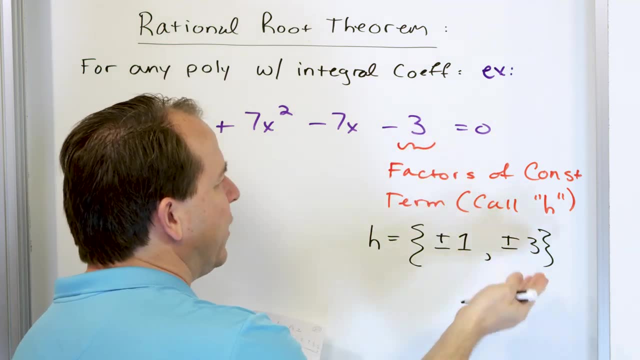 and plus or minus three. Why do we have factors of two of them? Because the last term here is negative. three right, So positive Positive 1 times something can give me negative 3.. Positive 1 times negative 3 gives me that. 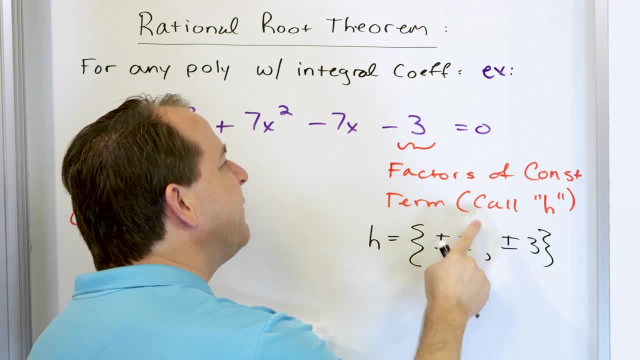 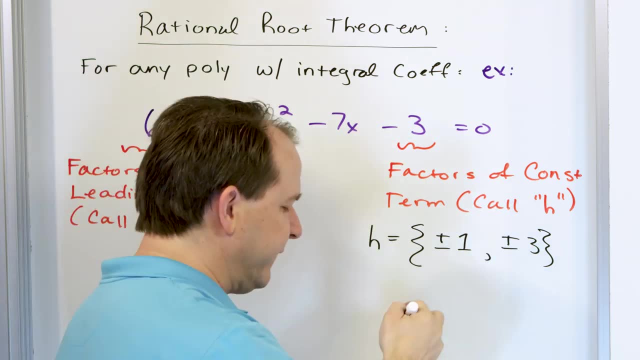 But negative 1 is a factor as well, because negative 1 times positive 3 gives me this Same thing here. Positive 3 times negative 1 gives me this. Negative 3 times positive 1 gives me this. So, as long as it can be multiplied, 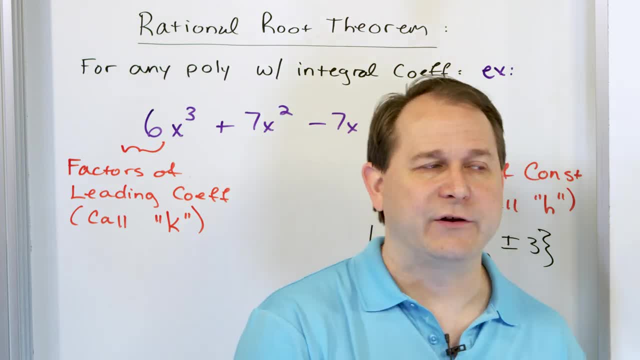 by anything to give me the thing that I'm looking for, then it's a factor. So for this exercise, when you find the factors, it's always going to have plus or minuses in front, So you find the numbers that are factors. 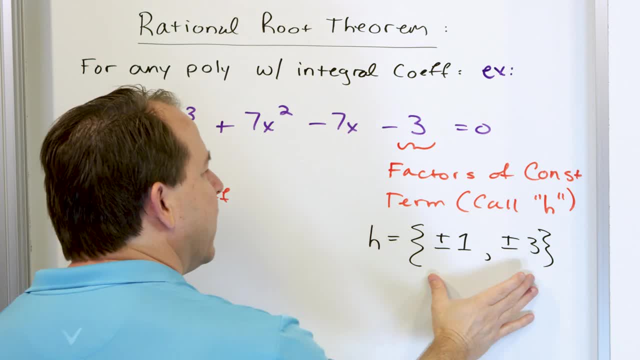 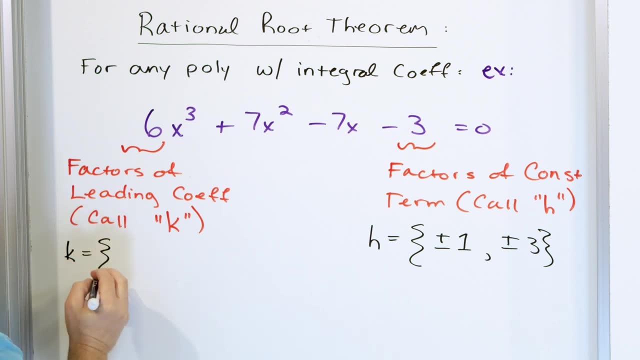 and you slap positive minus in front of that. That's the set of factors of this term. We call them h. Now we're going to find this one. This is a longer set. We call this one k. So I'm going to put a little curly brace. 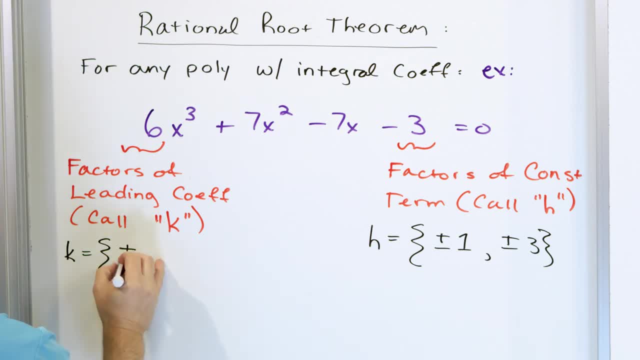 The set of numbers that are factors of this guy is plus or minus 1.. 1 times 6 is 6.. Plus or minus 2. 2 times 3 is 6, so that works Plus or minus 3.. 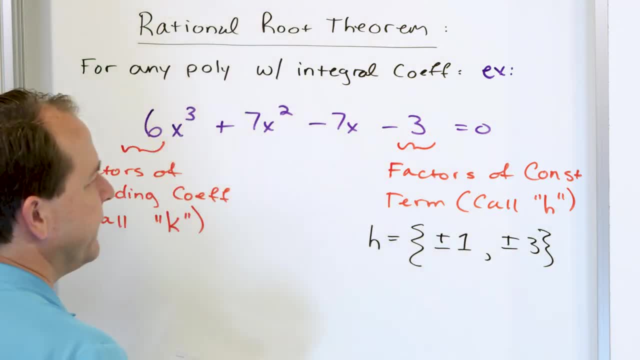 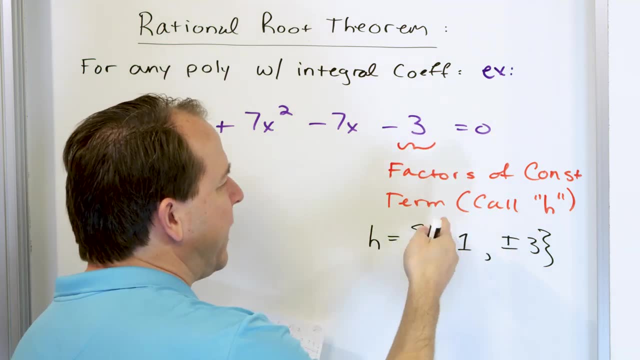 and plus or minus three. Why do we have factors of two of them? Because the last term here is negative three, right? So positive one 1 times something can give me negative 3.. Positive 1 times negative 3 gives me that. 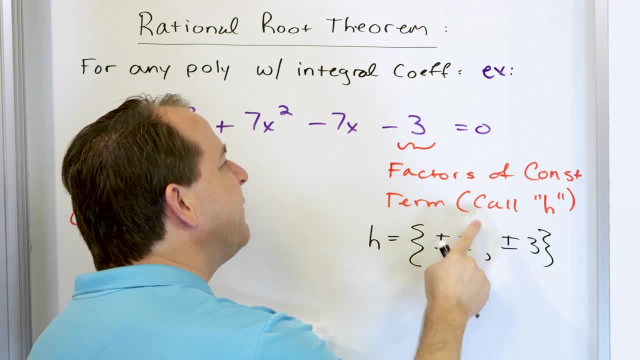 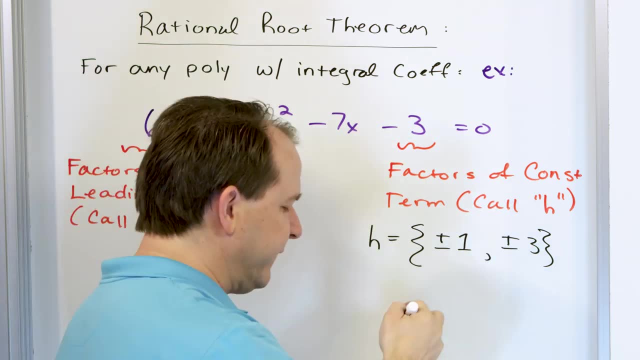 But negative 1 is a factor as well, because negative 1 times positive 3 gives me this Same thing here. Positive 3 times negative 1 gives me this. Negative 3 times positive 1 gives me this. So, as long as it can be multiplied, 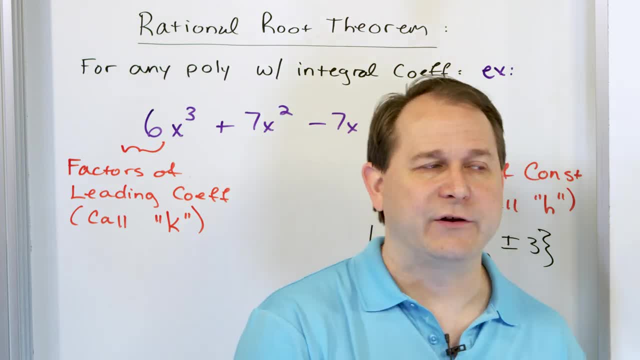 by anything to give me the thing that I'm looking for, then it's a factor. So for this exercise, when you find the factors, it's always going to have pluses or minuses in front, So you find the numbers that are factors. 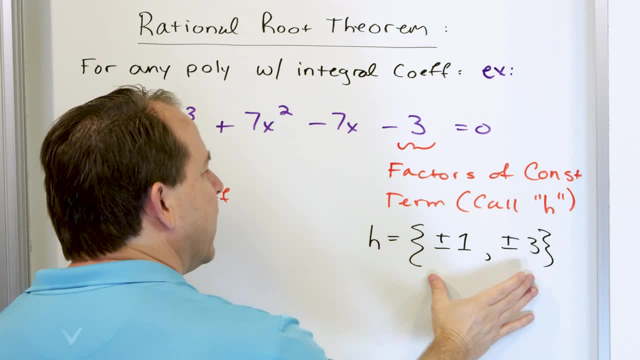 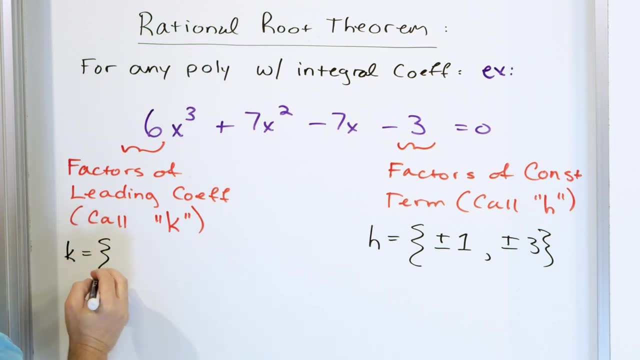 and you slap positive minus in front of that. That's the set of factors of this term. We call them h. Now we're going to find this one. This is a longer set. We call this one k. So I'm going to put a little curly brace. 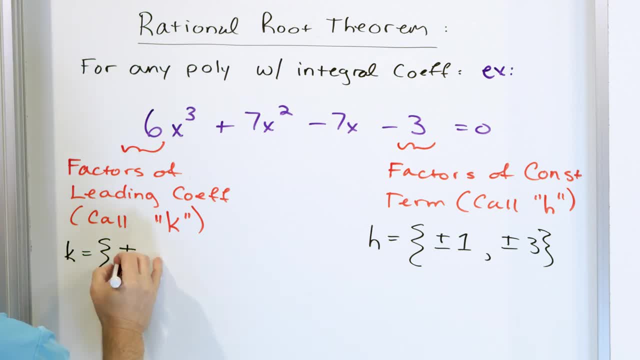 The set of numbers that are factors of this guy is plus or minus 1.. 1 times 6 is 6.. Plus or minus 2. 2 times 3 is 6, so that works Plus or minus 3.. 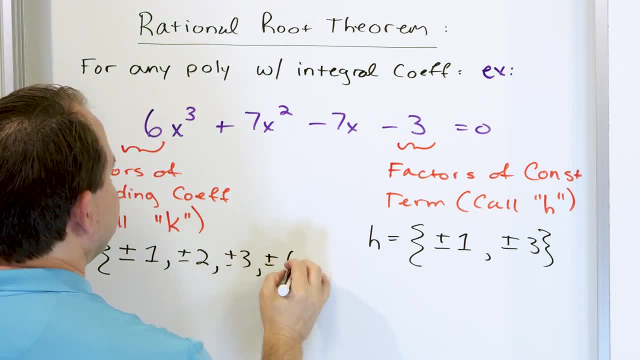 3 times 2 is 6, so that's a factor And plus or minus 6,, because 6 times 1 is 6.. Notice that something like 4 is not in this list, because 4 times nothing works to give me 6.. 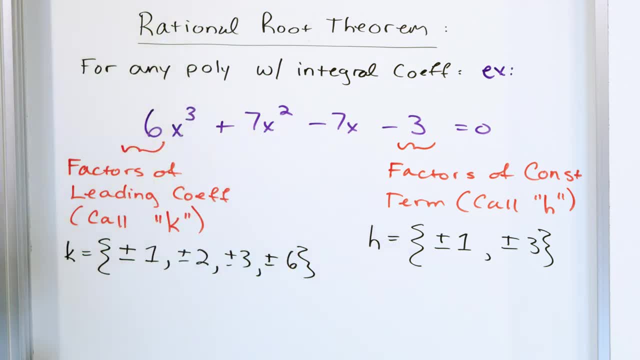 5 isn't in this list because 5 times nothing works to give me 6.. In order to be in the list it has to be a factor of the coefficient. here We call these the h factors and these the k factors. 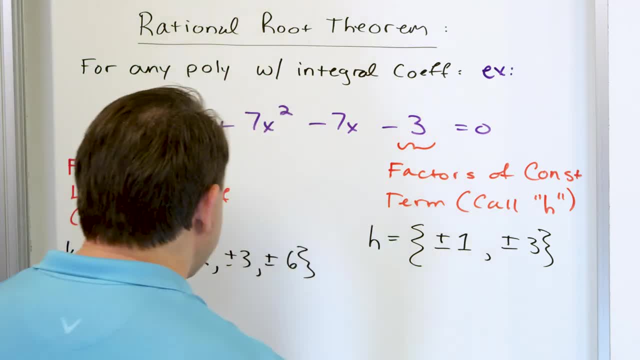 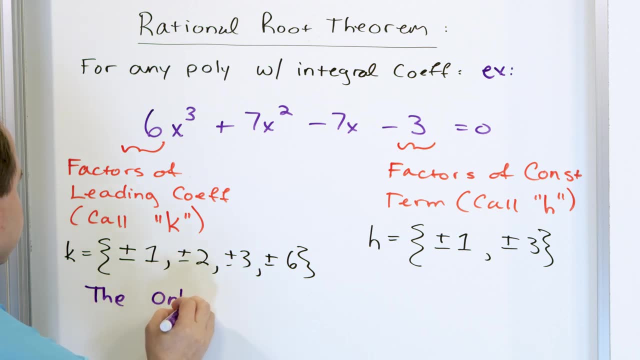 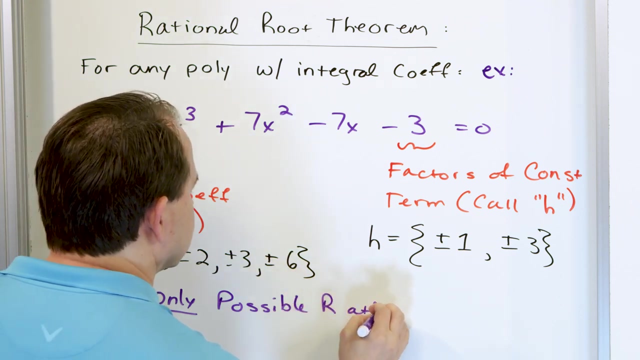 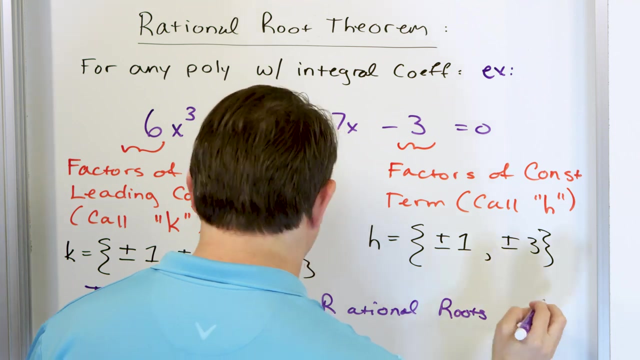 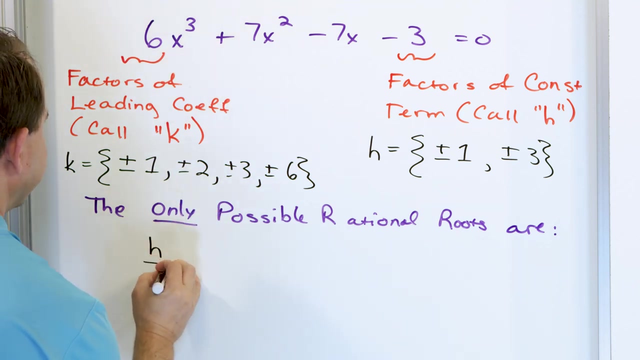 Now, why did we go through the trouble of naming them like this? And it's because of the following thing. So the only possible rational root of this polynomial are the following: And basically I'm just going to write them down as h divided by k. 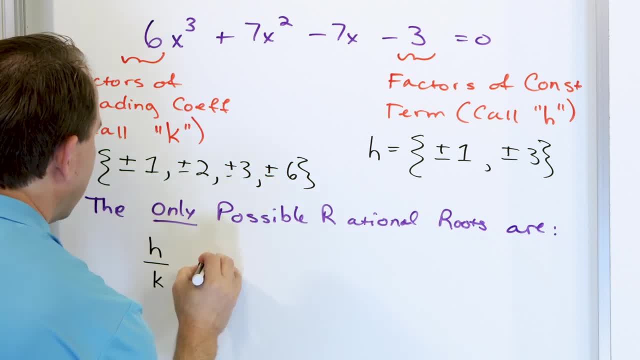 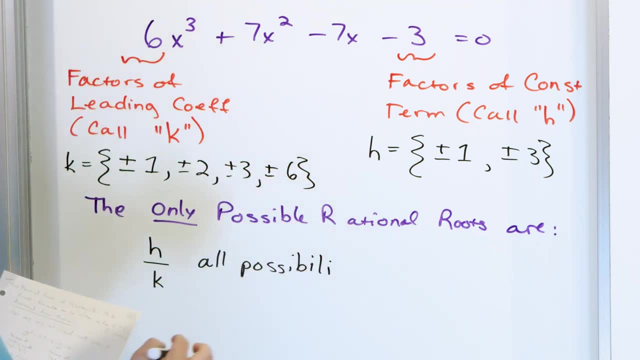 So what you have- and I'm going to write this down- all possibilities, Possibilities, Possibilities. Yeah, Sorry about that, It took me a minute to make sure I can spell possibilities, All right, So basically, what I'm going to do is I'm going to write this down. 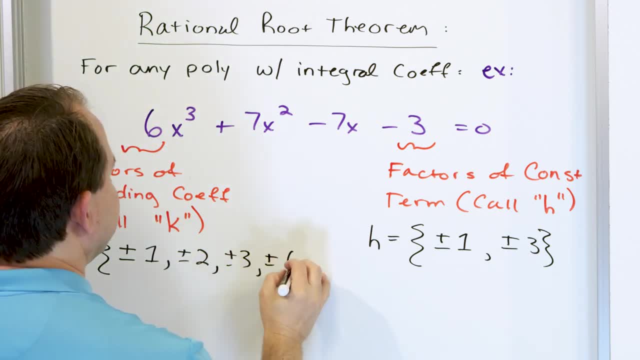 3 times 2 is 6, so that's a factor And plus or minus 6,, because 6 times 1 is 6.. Notice that something like 4 is not in this list, because 4 times nothing works to give me 6.. 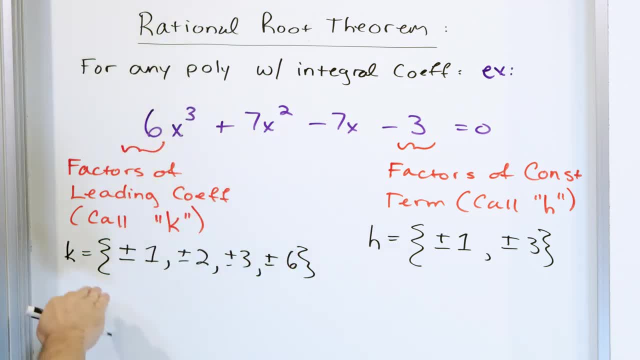 5 isn't in this list because 5 times nothing works to give me 6.. In order to be in the list it has to be a factor of the coefficient. here We call these the h factors and these the k factors. 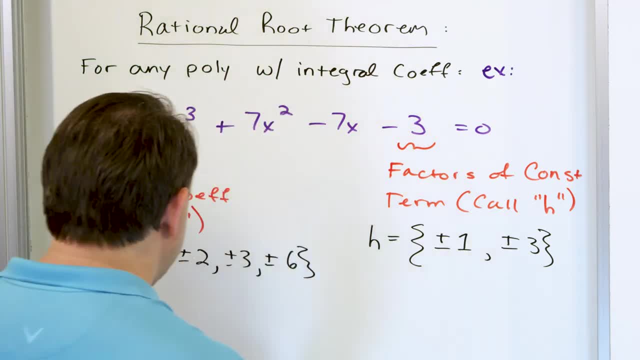 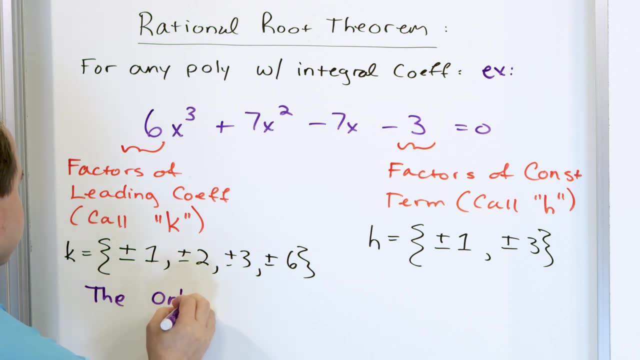 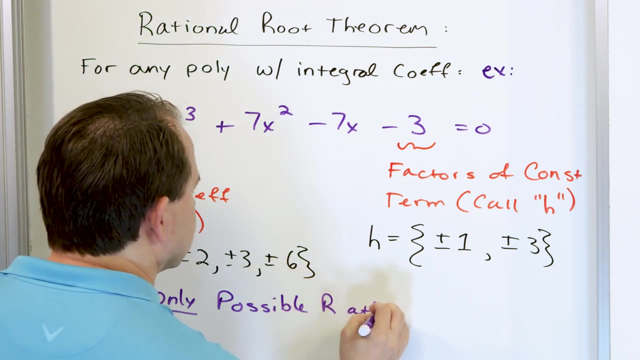 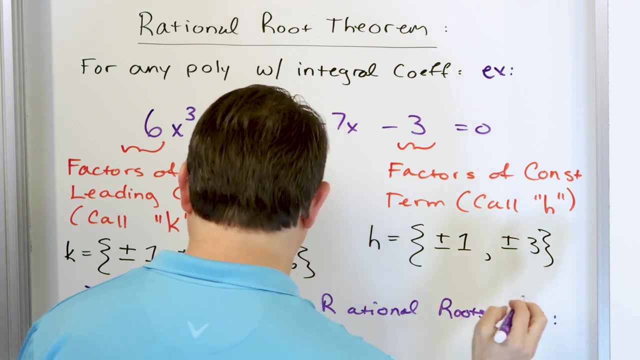 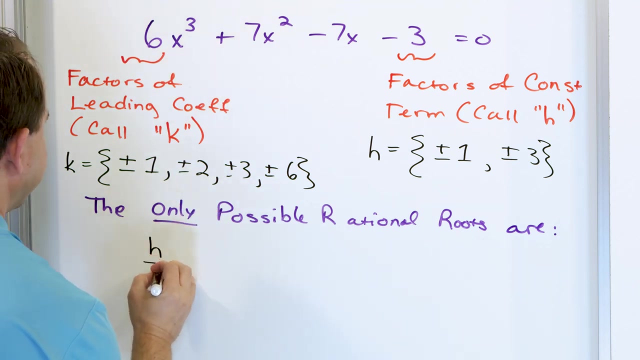 Now, why did we go through the trouble of naming them like this? And it's because of the following thing. So the only only possible rational root of this polynomial are the following: And basically I'm just going to write them down as h divided by k. 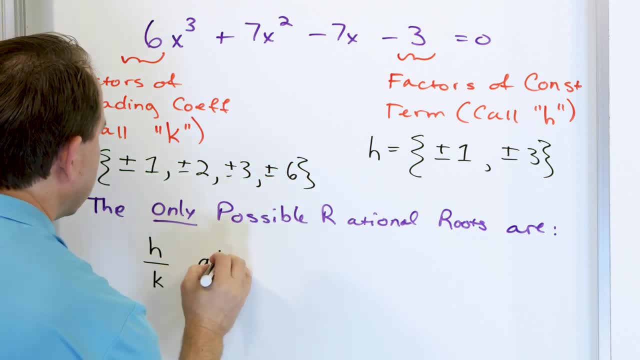 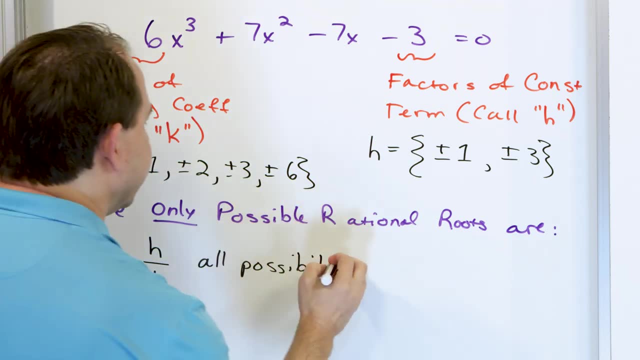 So what you have- and I'm going to write this down- all possibilities, Possibilities, Possibilities. Yeah, Sorry about that, It took me a minute to make sure I can spell possibilities, All right, so basically what you're saying: 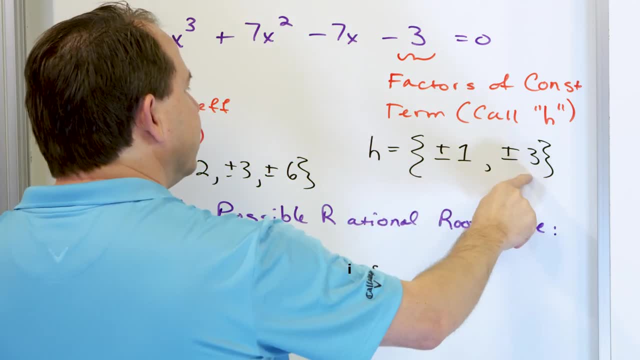 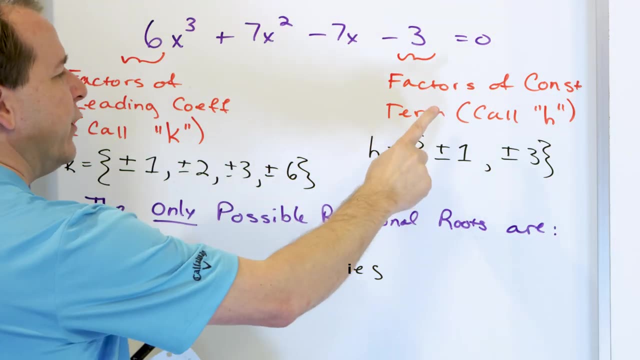 is you take h over k, which means all of the numbers in this set of lists divided by all of the numbers in this set of lists. But you have a lot of combinations because, don't forget, I have, for instance, 1 over 1.. 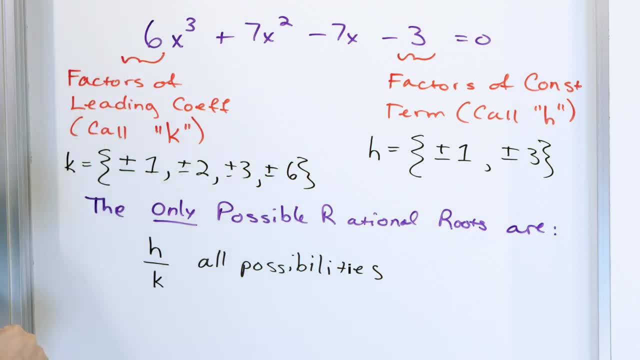 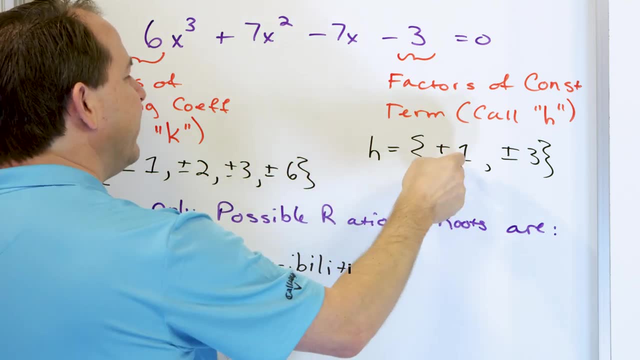 That is one of the possibilities to be a root right, 1 over 2,, 1 over 3,, 1 over 6, those are all possibilities. However, I have negative 1 here, so it's negative 1 over 1,. 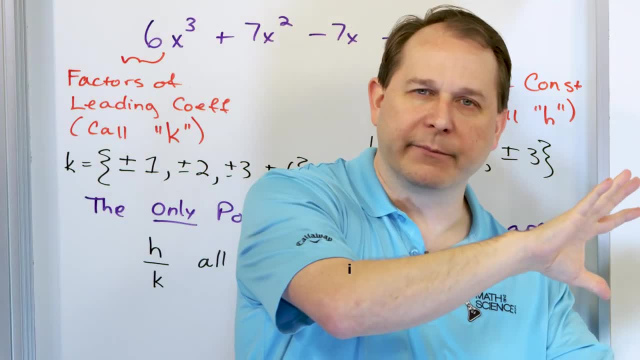 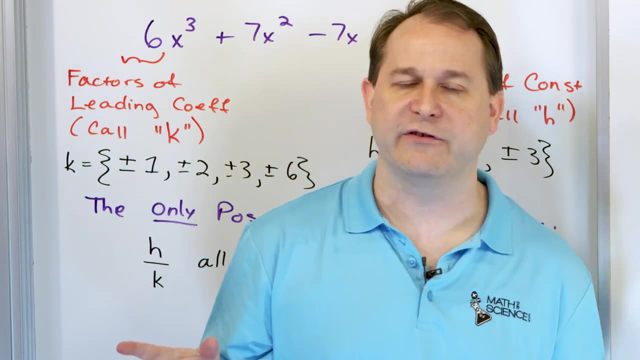 negative 1 over. So I have all the possibilities of all the numbers over here divided by all the numbers here, and I also have all the possibilities of all the signs: positive over negative, negative over positive and so on. Now, that's not telling me that all of these possibilities 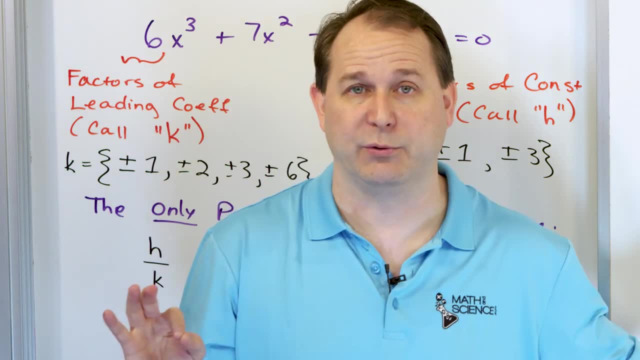 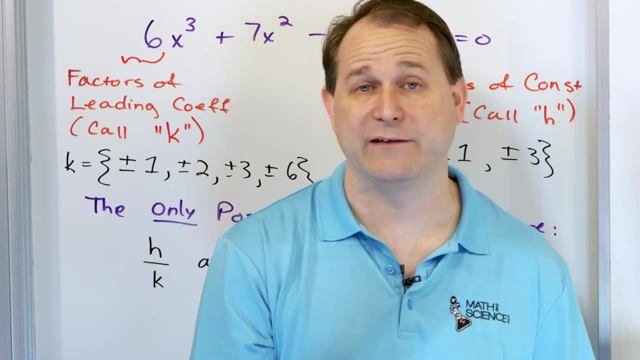 are actually roots. It's telling me all of the possible ones. So if you're going to find the rational roots of the polynomial, they have to be in this list of numbers that we're about to write down. So the easiest way to do it is to do something like this: 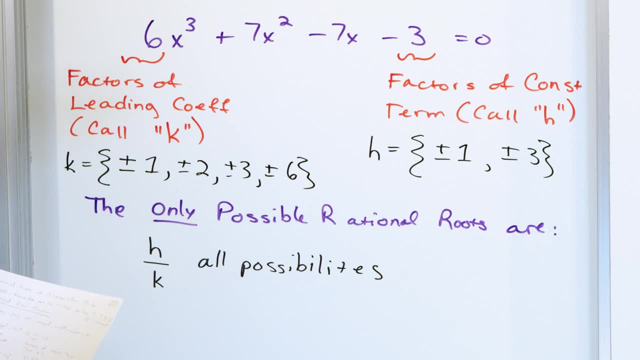 We say the following thing: Let's see where do I want to write this. I think I'm going to go to the next board, so I don't crunch it up. So I have 1 and 3, and then 1,, 2, 3, and 6,. all right, 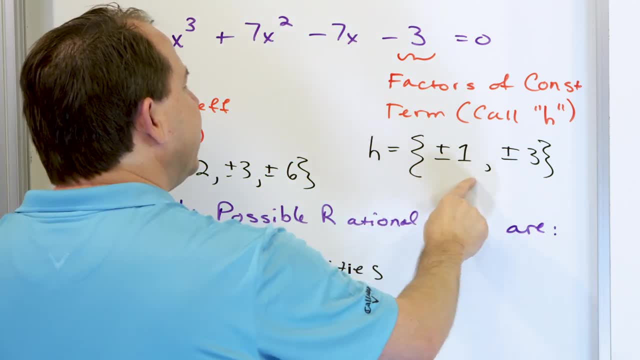 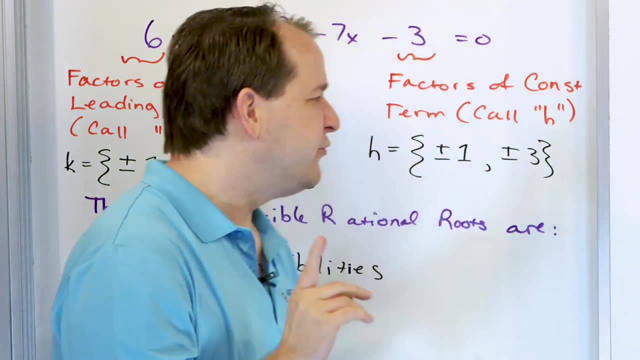 So, basically, what you're saying is you take h over k, which means all of the numbers in this set of lists divided by all of the numbers in this set of lists. But you have a lot of combinations Because, don't forget, I have, for instance, 1 over 1.. 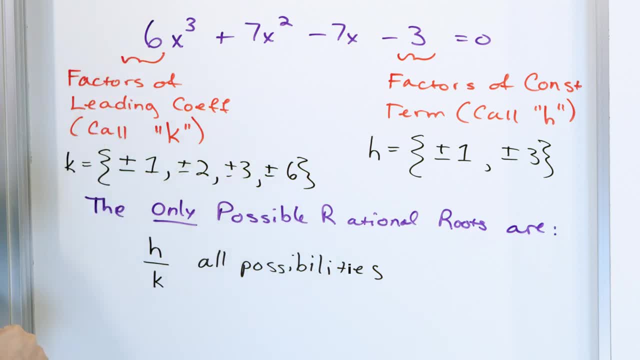 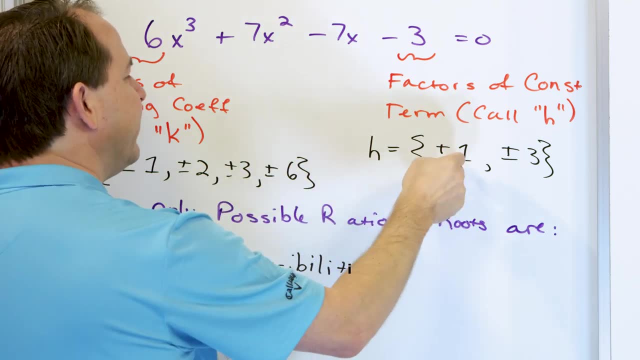 That is one of the possibilities to be a root right, 1 over 2,, 1 over 3, 1 over 6, those are all possibilities. However, I have negative 1 here, So it's negative 1 over 1, negative 1 over 2.. 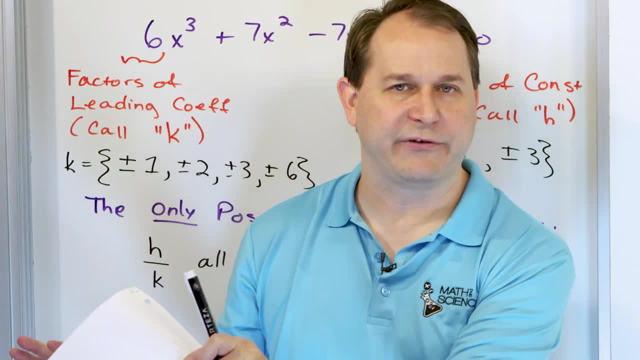 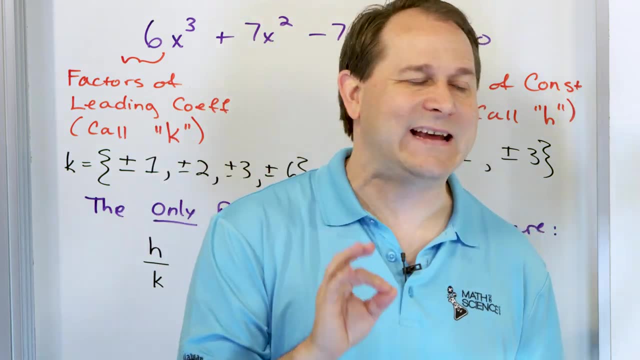 I have all the possibilities of all the numbers over here divided by all the numbers here, And I also have all the possibilities of all the signs: positive over negative, negative over positive, and so on. Now, that's not telling me that all of these possibilities 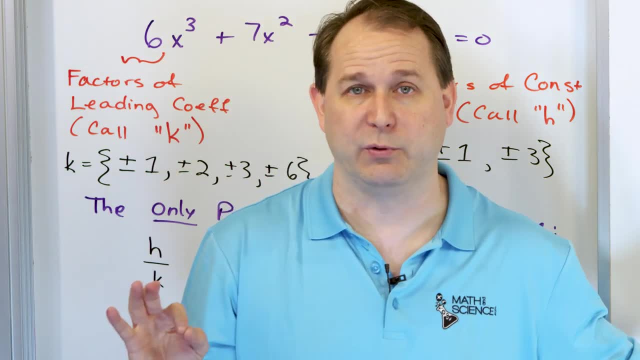 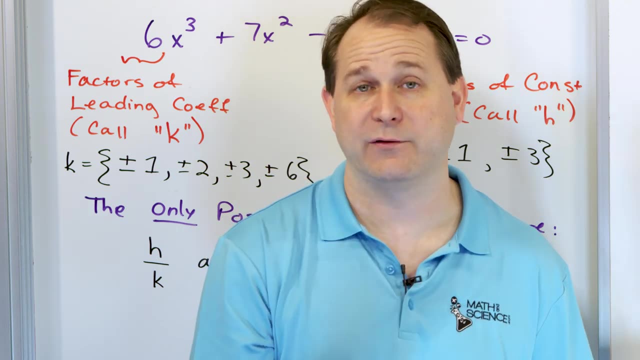 are actually roots. It's telling me all of the possible ones. So if you're going to find the rational roots of the polynomial, they have to be in this list of numbers that we're about to write down. So the easiest way to do it is to do something like this: 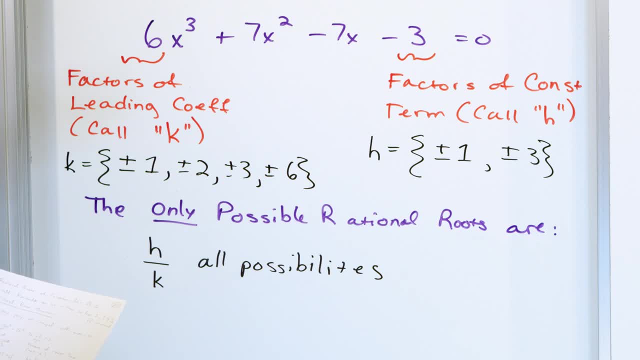 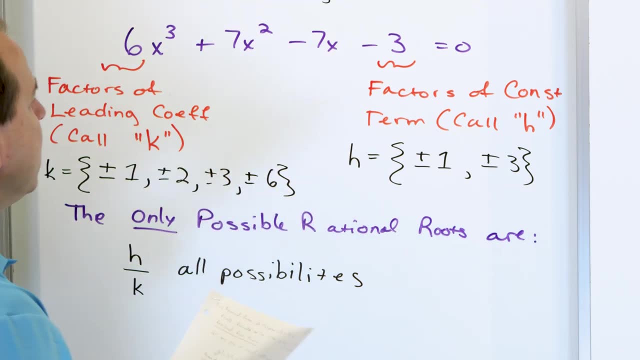 We say the following thing: Let's see Where do I want to write this. I think I'm going to go to the next board, so I don't crunch it up. So I have 1 and 3, and then 1,, 2, 3, and 6,. all right, 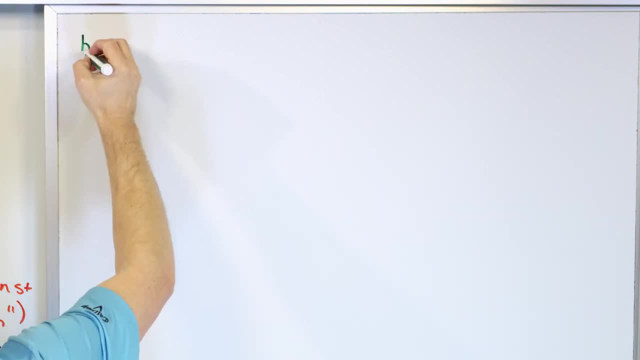 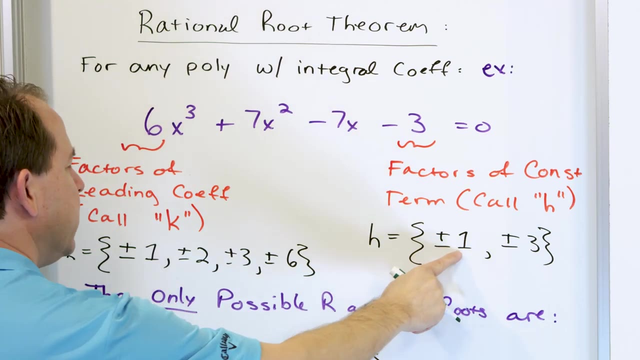 So the way we're going to write it is this: We're going to say h over k And that's going to be- I'll put a little colon here- right? So we have 1 over 1,, 2,, 3, and 6.. 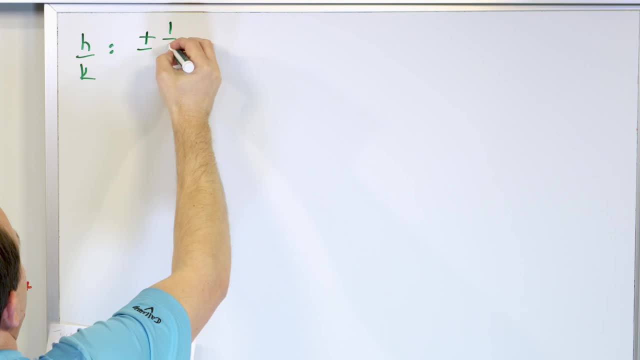 Here's how we're going to write it. It's going to be plus or minus 1 over 1, plus or minus 1 over 1, then plus or minus 1 over 2, then plus or minus 1 over 3.. 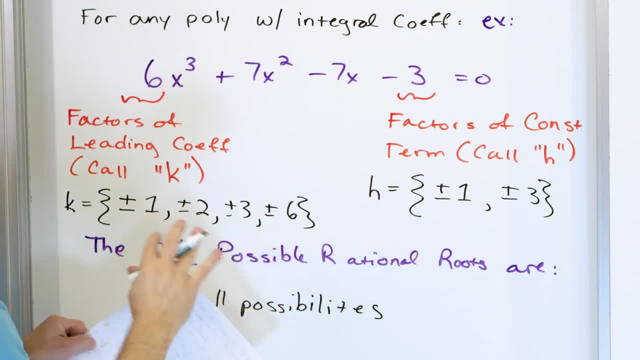 Then plus or minus 1 over 6.. The plus and minus catches all of the possibilities And then the dividing catches, of course the fraction. So 1 over 2, 1 over 3,, 1 over 6.. 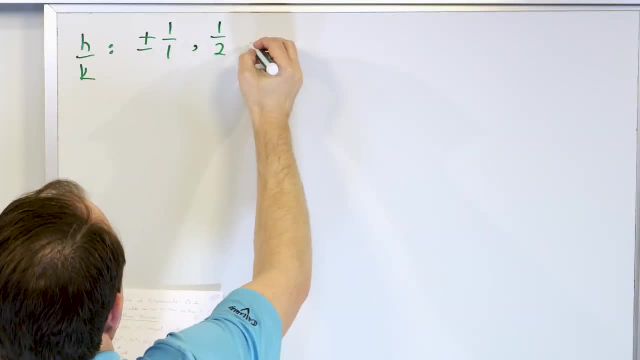 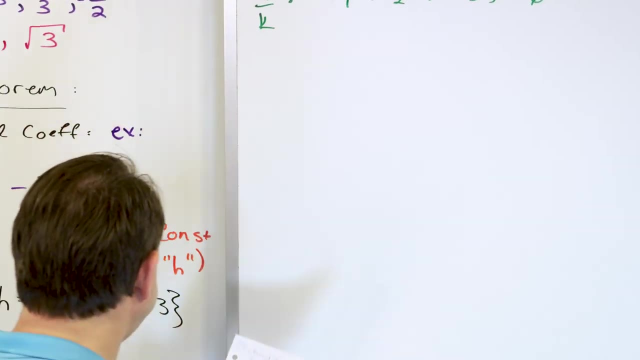 But we have to have the plus or minuses in front: 1 over 2. Got to have plus or minus, sorry. Plus or minus 1 over 3, plus or minus 1 over 6.. So now we've exhausted all the possibilities of 1 over 1, 1. 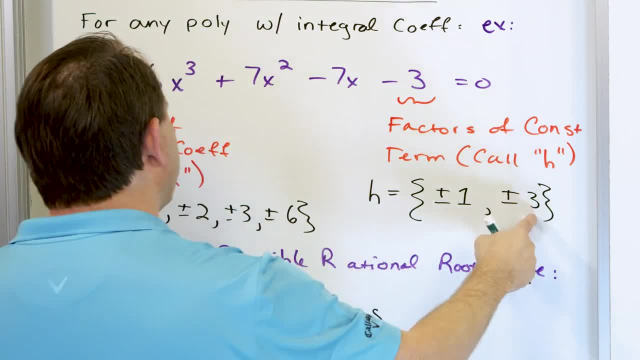 over 2, 1 over 3, 1 over 6.. Then we switch to this one: 3 over 1, 3 over 2, 3 over 3,, 3 over 6.. And they continue on in the list here. 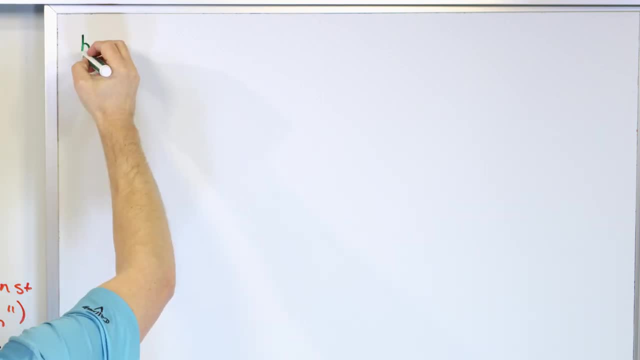 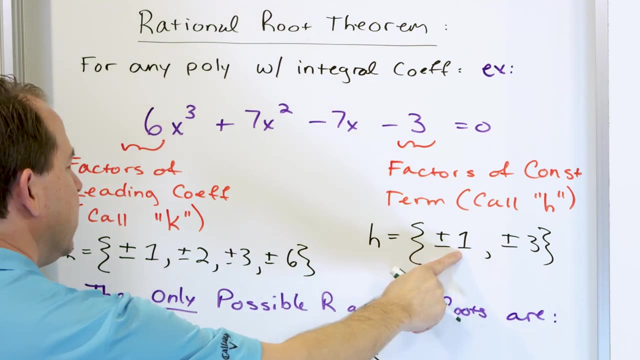 So the way we're going to write it is this: We're going to say h over k, And that's going to be- I'm going to put a little colon here- right? So we have 1 over 1,, 2,, 3, and 6.. 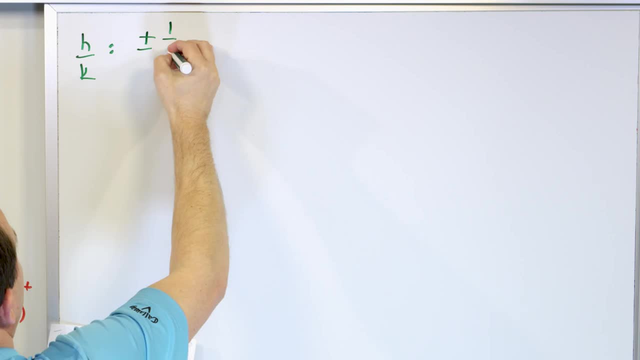 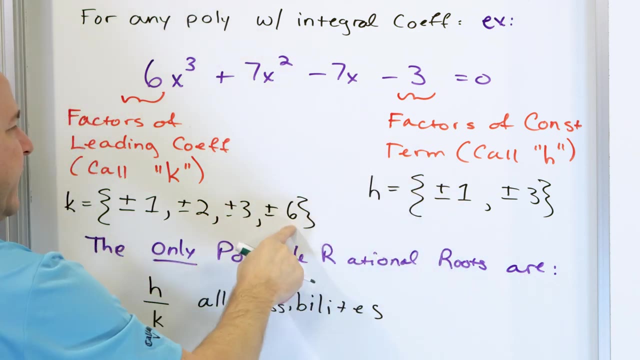 Here's how we're going to write it. It's going to be plus or minus 1 over 1, plus or minus 1 over 1, then plus or minus 1 over 2,, then plus or minus 1 over 3,, then plus or minus 1 over 6.. 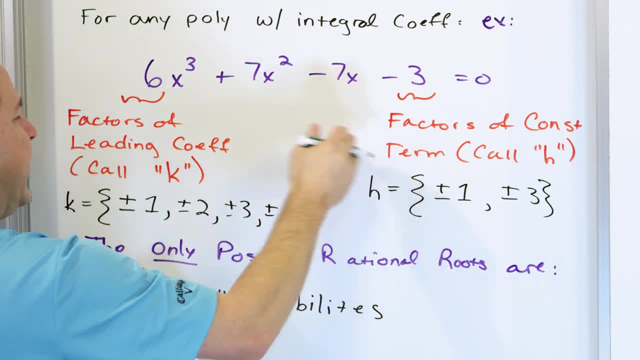 The plus and minus catches all of the possibilities, and then the dividing catches of course the fraction, So 1 over 2,, 1 over 3,, 1 over 6.. But we have to have the plus or minuses in front. 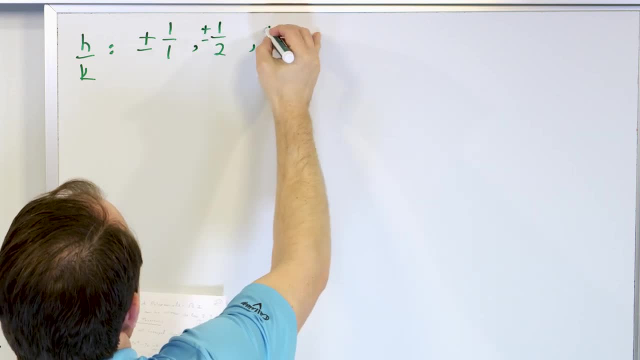 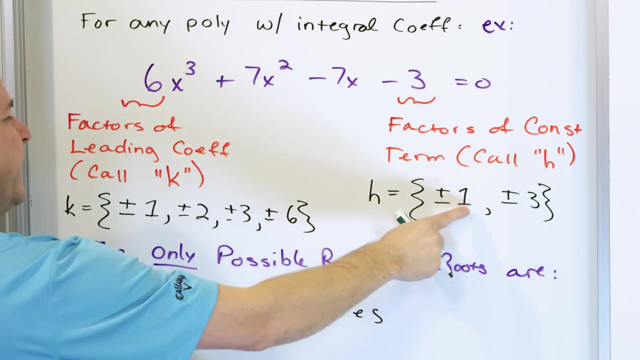 1 over 2, got to have plus or minus, sorry, Plus or minus, 1 over 3,, plus or minus 1 over 6.. So now we've exhausted all the possibilities of 1 over 1,, 1 over 2,, 1 over 3,, 1 over 6.. 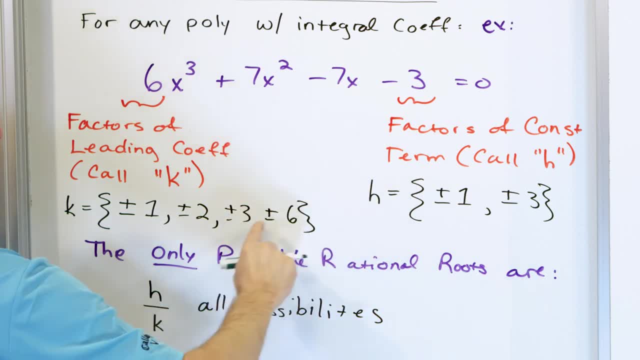 Then we switch to this one: 3 over 1,, 3 over 2,, 3 over 3,, 3 over 6.. And they continue on in the list here. So we have plus or minus- don't forget that- 3 over 1,. 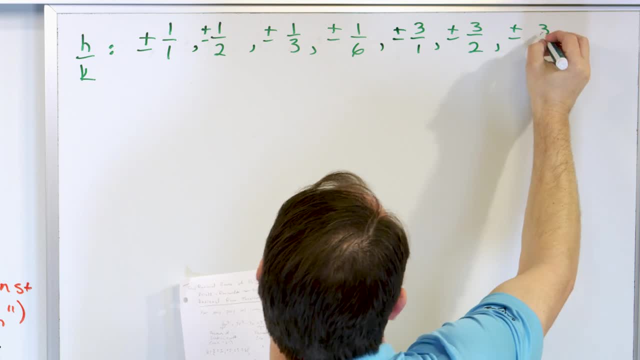 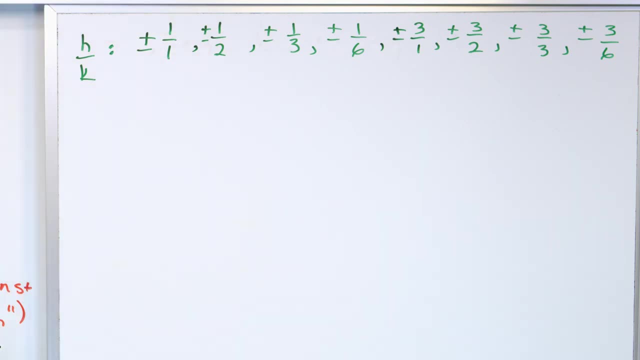 plus or minus 3 over 2, plus or minus 3 over 3, plus or minus 3 over 6.. You can see there's a lot of numbers there, But we can simplify this list quite a bit. So what you do is you first write it all down. 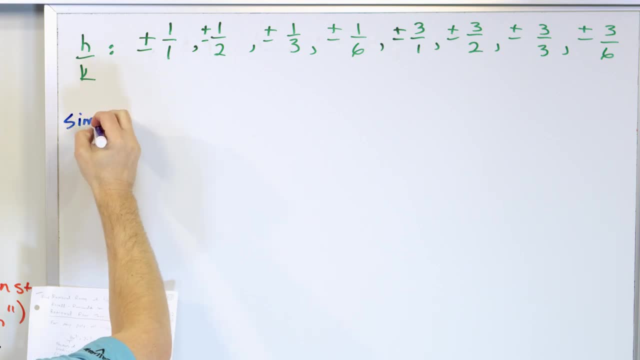 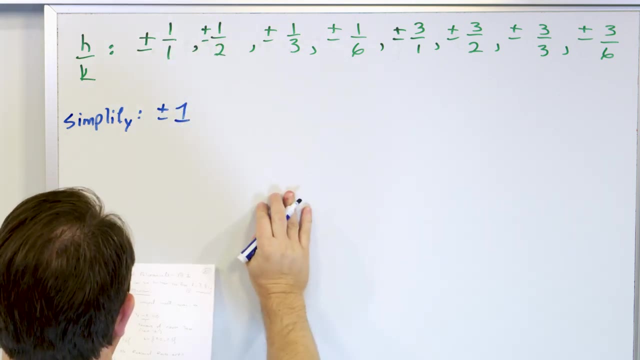 Then we need to go one more step and simplify. We simplify it like this: Plus or minus 1 over 1 is just plus or minus 1.. Plus or minus 1- half. we can't do anything more with that, So we're just going to leave it like this. 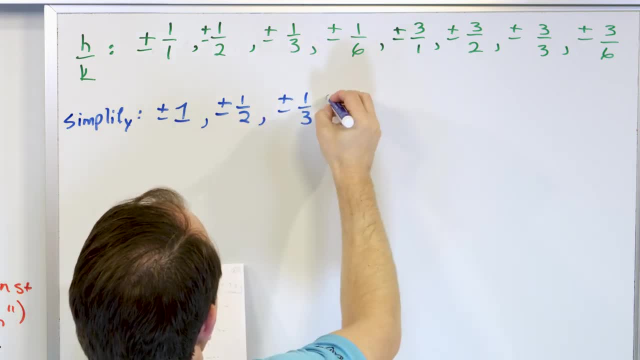 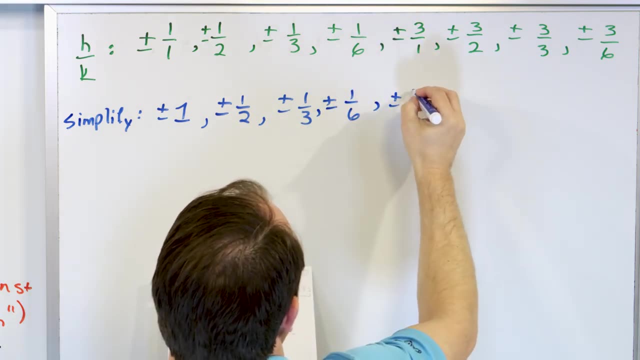 Plus or minus 1. third, that's in the list. We can't do much with that. Plus or minus 1 over 6, can't do much with that. But 3 over 1 is just plus or minus 3.. 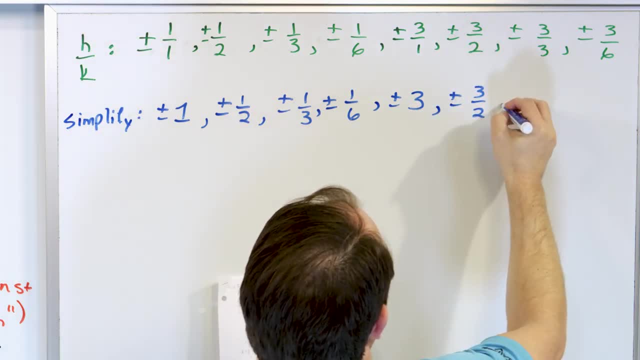 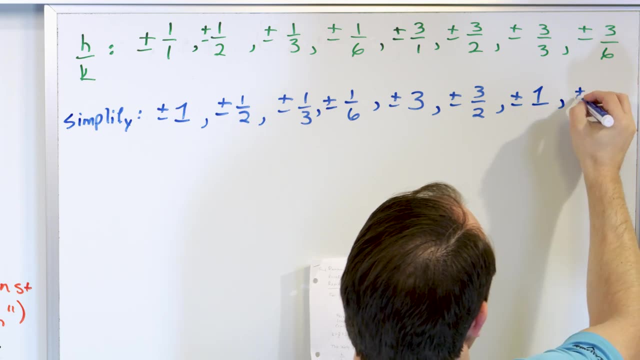 3 halves. we can't do much with that. So we have 3 halves, But then we have plus or minus 3 over 3.. But notice that becomes 1.. 3 over 3 is 1.. And then over here we have plus or minus 3 over 6.. 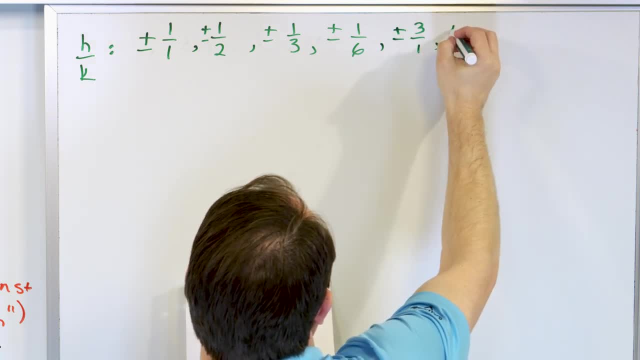 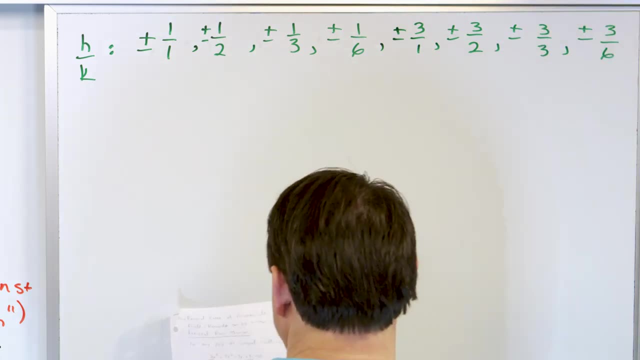 So we have plus or minus- don't forget that- 3 over 1, plus or minus 3 over 2, plus or minus 3 over 3, plus or minus 3 over 6.. You can see there's a lot of numbers there. 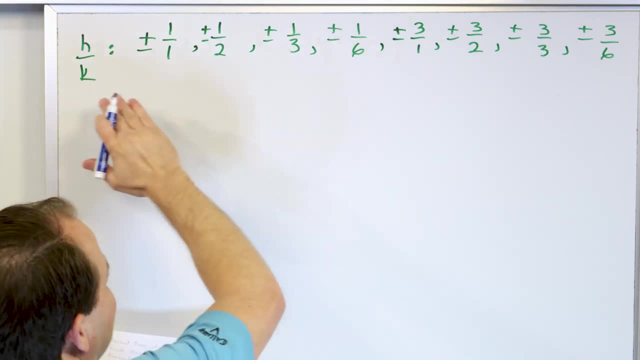 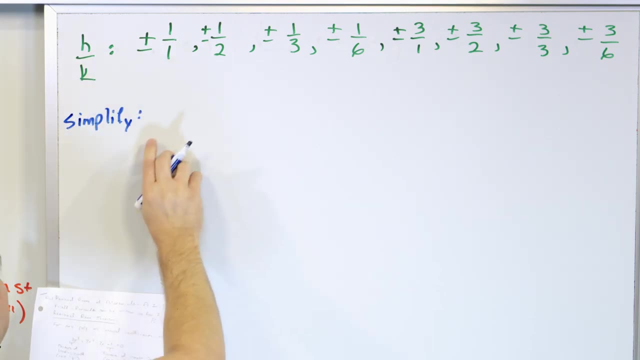 But we can simplify this list quite a bit. So what you do is you first write it all down, Then we need to go one more step and simplify. We simplify it like this: Plus or minus 1 over 1.. It's just plus or minus 1.. 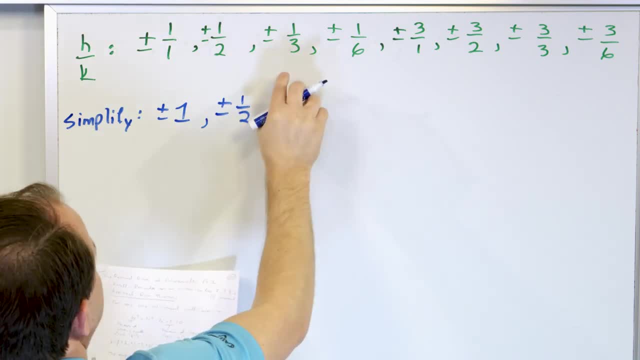 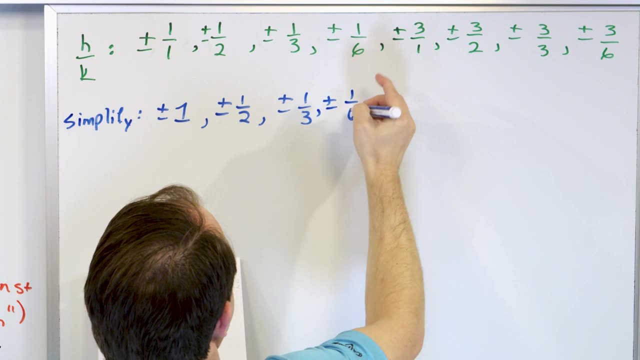 Plus or minus 1 half. We can't do anything more with that, So we're just going to leave it like this. Plus or minus 1 third. That's in the list. We can't do much with that. Plus or minus 1 over 6.. 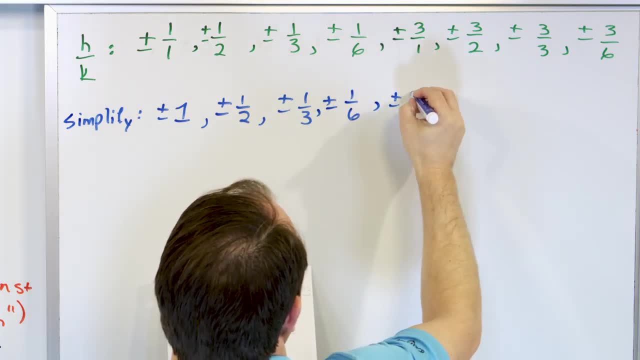 Can't do much with that. But 3 over 1 is just plus or minus 3.. 3 halves- we can't do much with that. So we have 3 halves, But then we have plus or minus 3 over 3.. 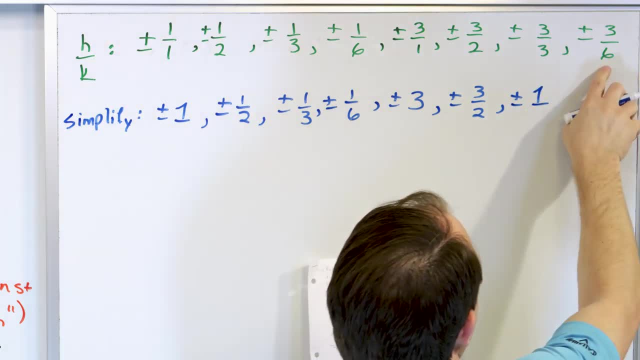 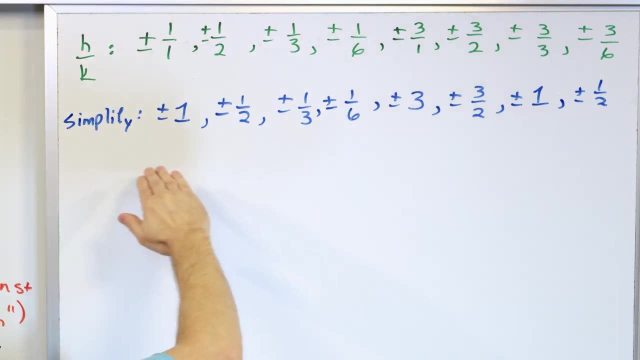 But notice that becomes 1.. 3 over 3 is 1.. And then over here we have plus or minus 3 over 6. But we know that reduces 1. It reduces to 1 half. So now what we've done is we've simplified our list. 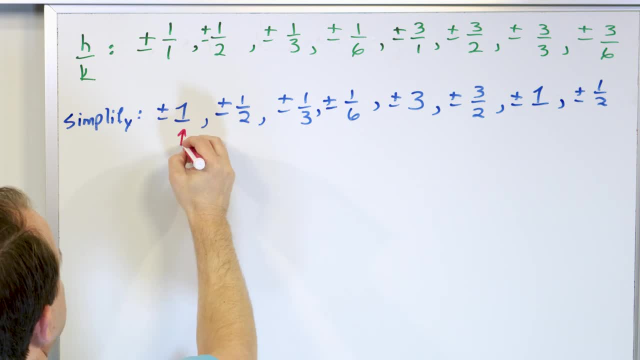 But then we notice right away that we actually have some duplicates in the list. This is a duplicate of that number 1. We don't need duplicates in the list. Either it's a root or it's not a root. And then this guy, the 1 half is also a dupe. 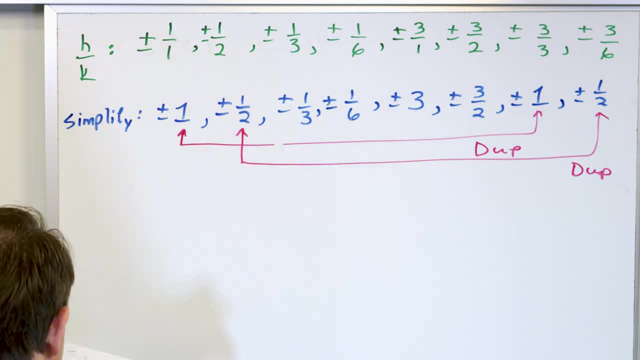 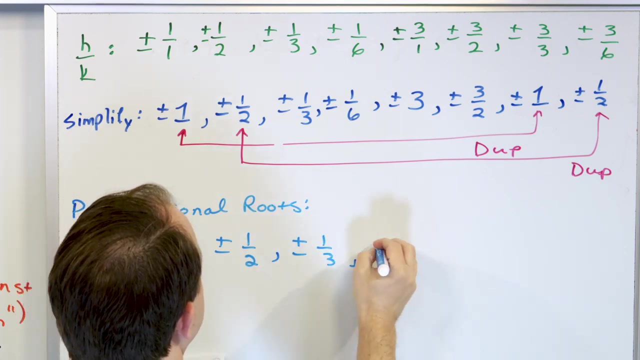 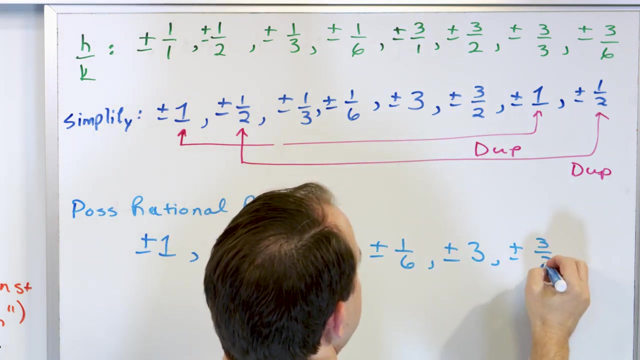 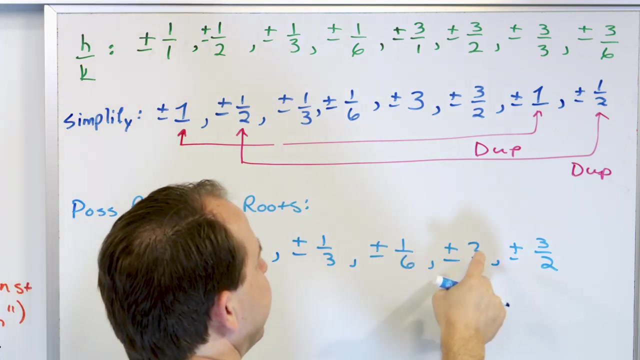 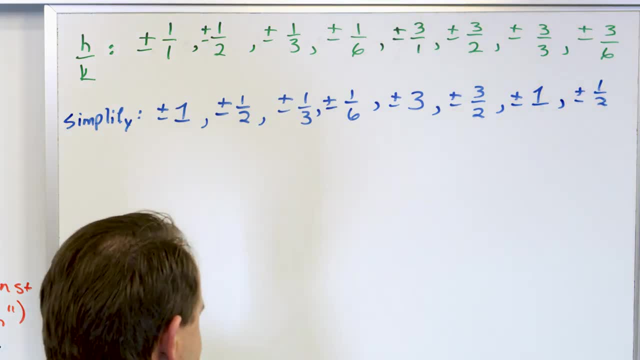 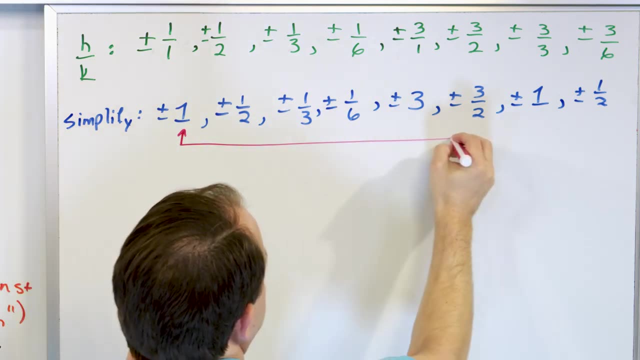 But we know that reduces to 1 half. So now what we've done is we've simplified our list, But then we notice right away that we actually have some duplicates in the list. This is a duplicate of that number 1.. We don't need duplicates in the list. 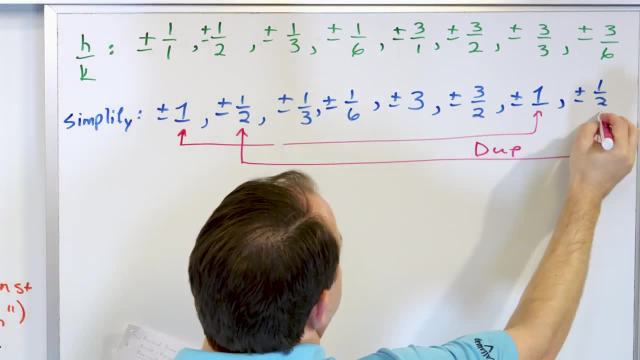 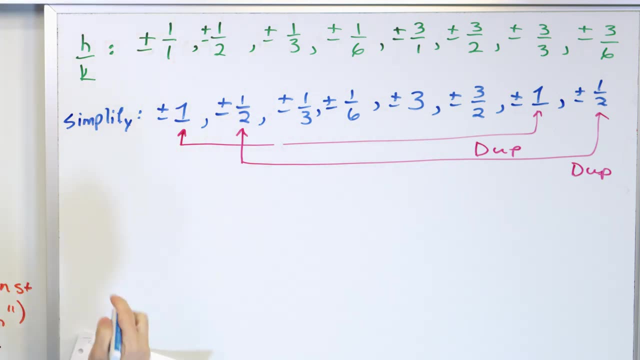 Either it's a root or it's not a root. And then this guy, the 1 half, is also a dupe. So what I do whenever I'm doing these problems is then we say: the possible, Possible rational roots can only be in this list. 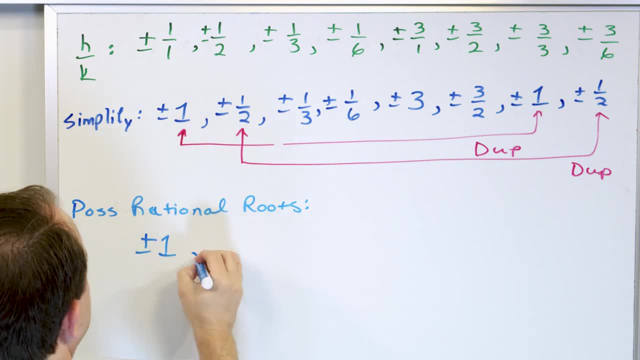 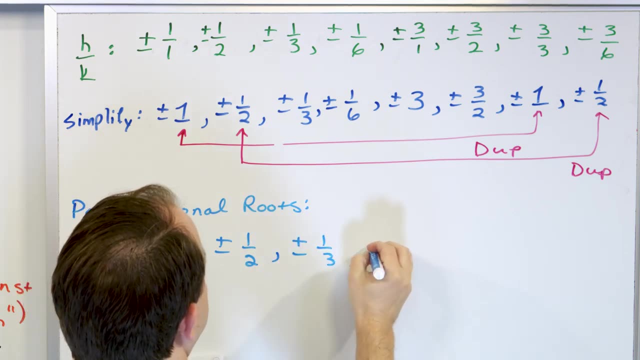 We can only have plus or minus 1 here, plus or minus 1 half from there, We're not going to count those twice. Then we have plus or minus 1 third, plus or minus 1 sixth, plus or minus 3 from here, and then plus or minus 3 halves. 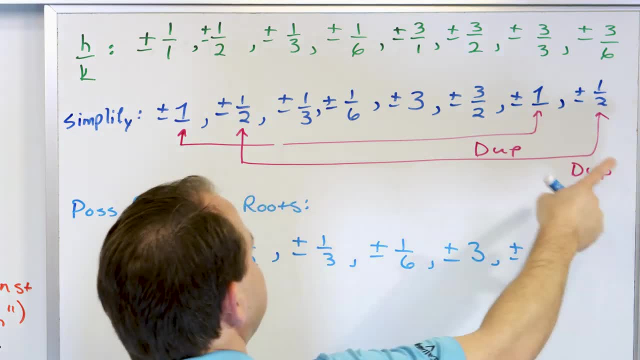 I'm not going to put this one down again because it's already in the list. And I'm not going to put this one down again because it's already in the list. So you have 1,, 2,, 3,, 4,, 5, 6,, but each one of them. 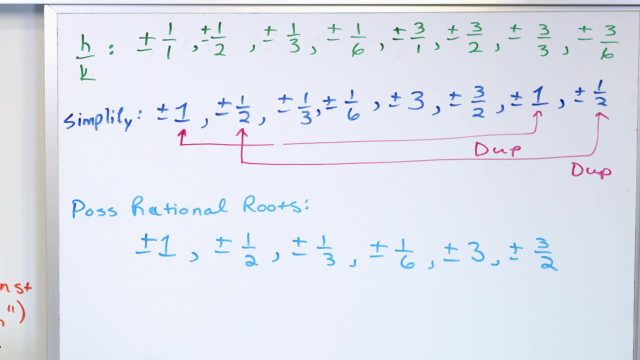 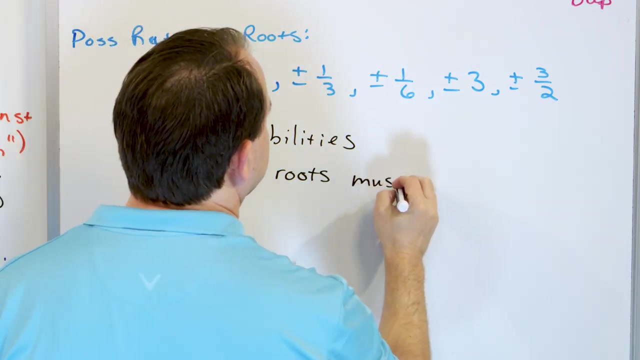 has positive or negative possibilities. So we actually have 12 possibilities. So you have 12 possibilities for the rational roots. So that must mean that all other roots that this polynomial has, all other roots, must be Either irrational, like square root of 2 or something like that. 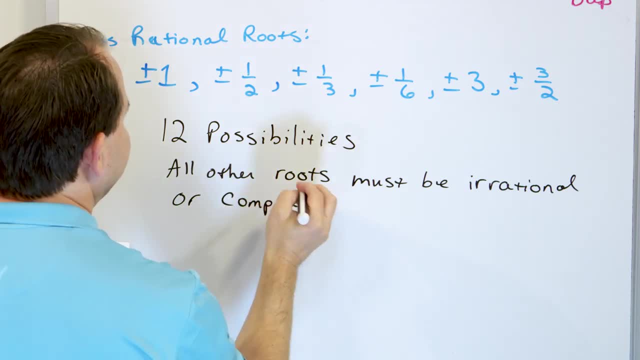 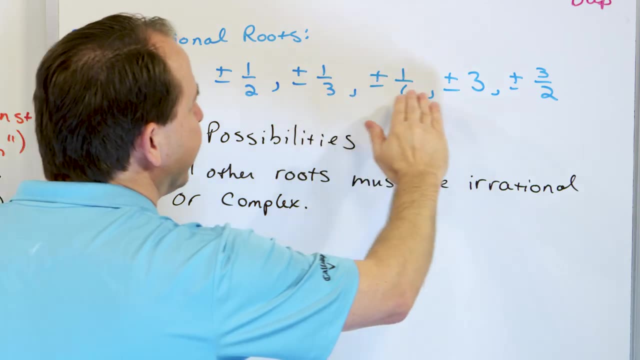 or complex, which means like 2i or 3i or something like that. So I have 12 possibilities here, And I'm not saying that these are all of the roots. I'm just saying that the only roots that any polynomial can. 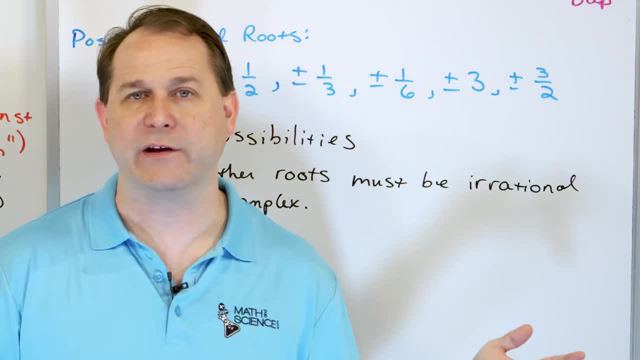 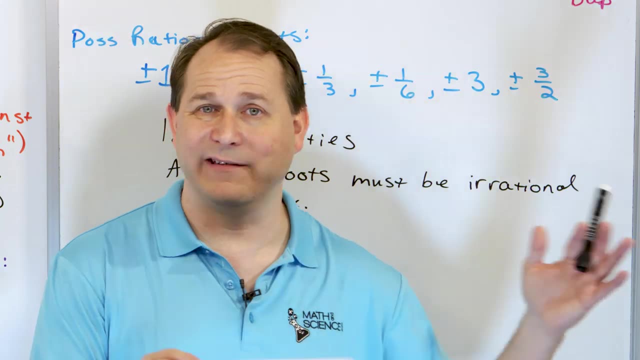 have are either going to be complex numbers, which this doesn't help you with at all, or they can be like radicals and irrational things like that. pi radical things like that, Things like this, which this isn't going to help you for. 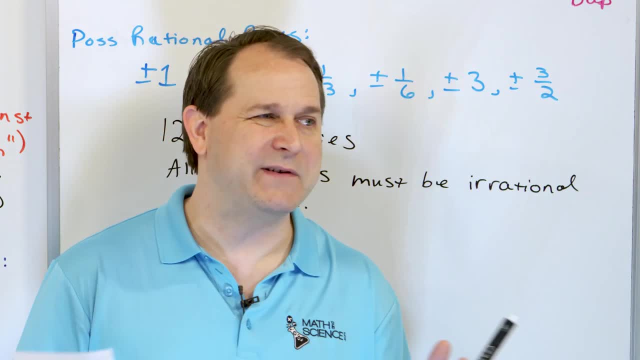 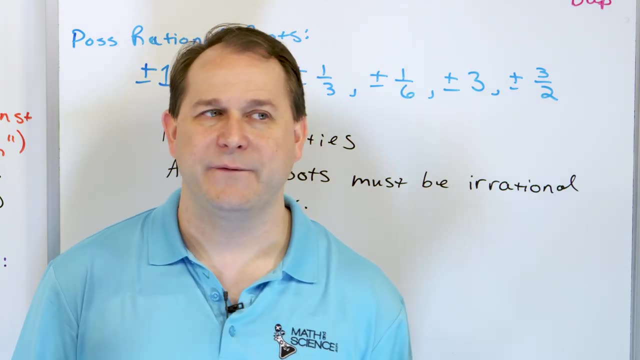 But any whole number roots, any fractional roots- positive, negative numbers, fractions, whole numbers, things like that- they have to be in this list of 12 numbers, 12 numbers. How do you actually figure out which of these things actually are the roots? 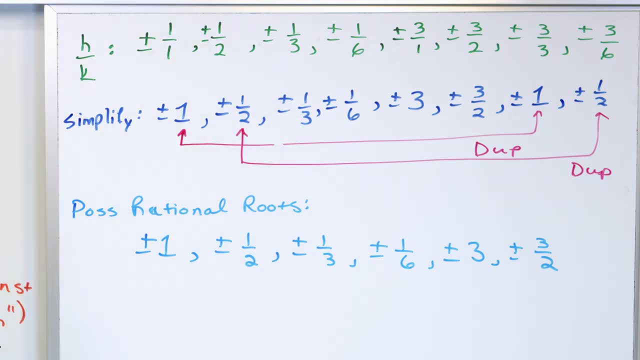 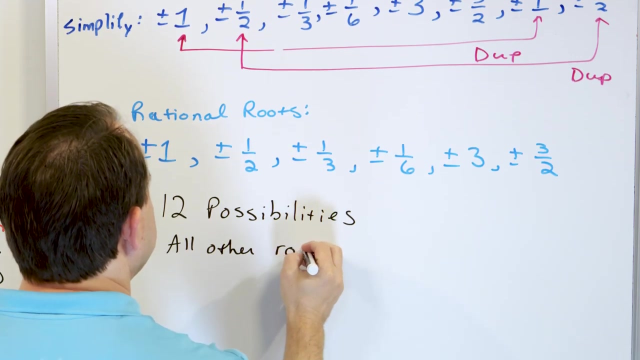 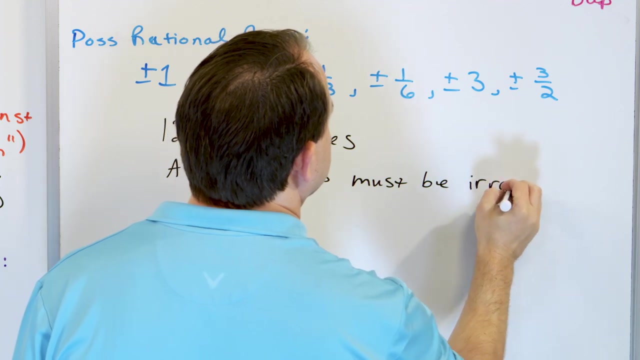 have 12 possibilities. So you have 12 possibilities for the rational roots. So that must mean that all other roots that this polynomial has, all other roots, must be either irrational, like square root of 2 or something like that, or complex, which. 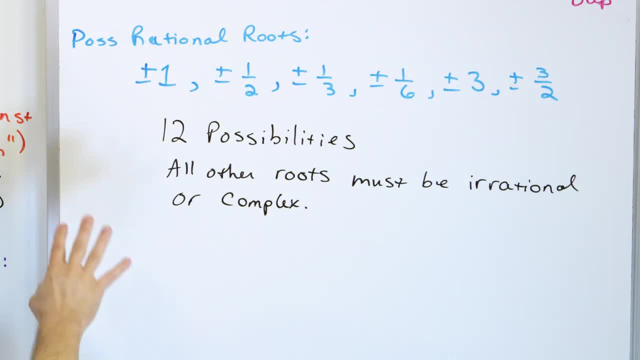 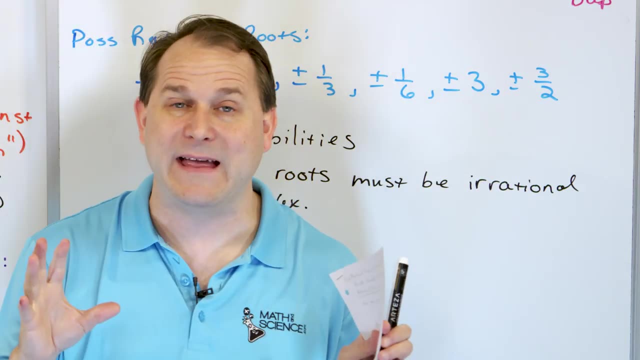 means like 2i or 3i or something like that. So I have 12 possibilities here, And I'm not saying that these are all of the roots. I'm just saying that the only roots that any polynomial can have are either going to be complex numbers, which this doesn't help. 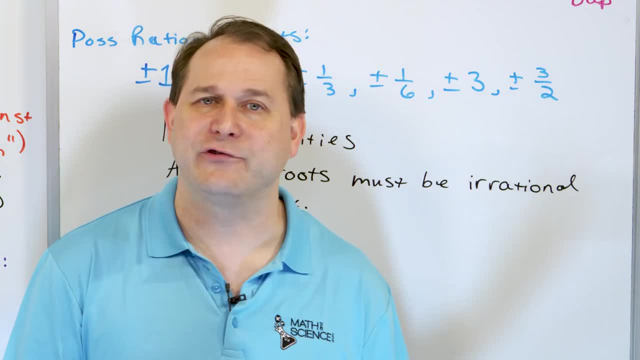 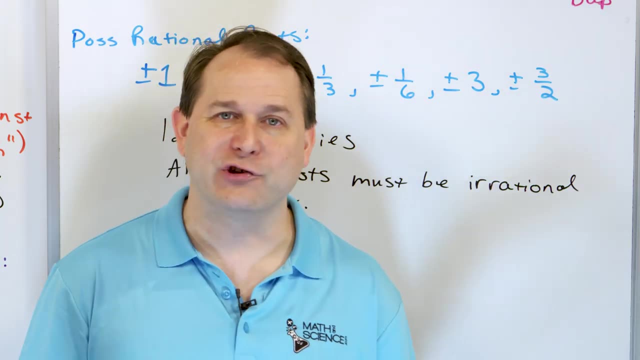 you with at all, or they can be like radicals and irrational things like that, Pi rational or radical things like this, which this isn't going to help you for. But any whole number roots, any fractional roots- positive, negative numbers, fractions whole. 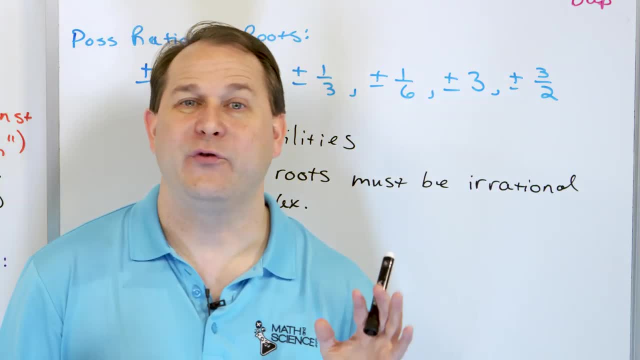 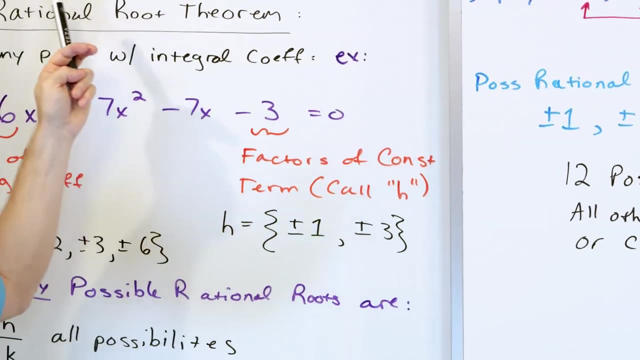 numbers, things like that. they have to be in this list of 12 numbers, 12 numbers. How do you actually figure out which of these things actually are the roots? Obviously, the equation is only a third order equation. It can only be three roots total. How can I find? 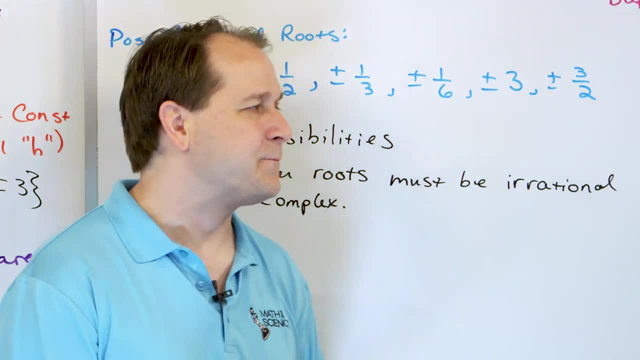 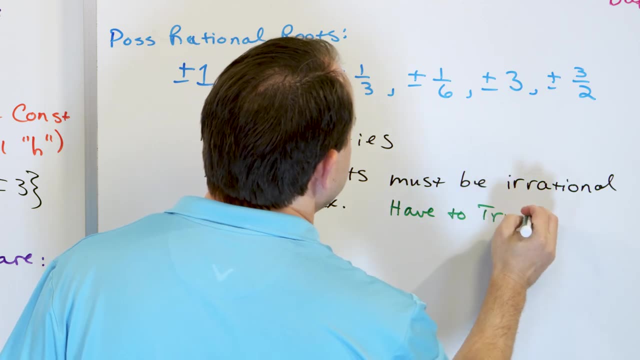 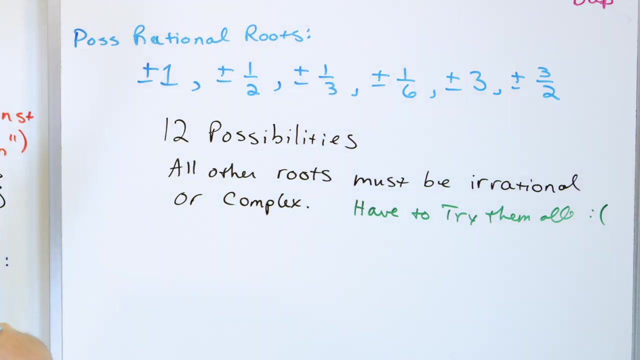 out which of these, if any of them, actually are a root of that. Well, unfortunately, you have To try them all, And that is not fun, right? Because that means you have to take the number one and stick it into this polynomial, see if it equals zero. Take negative one, put 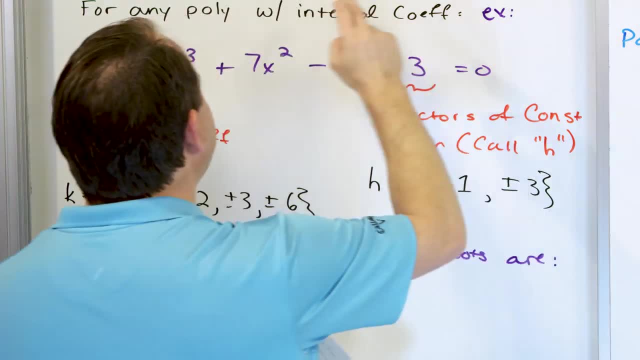 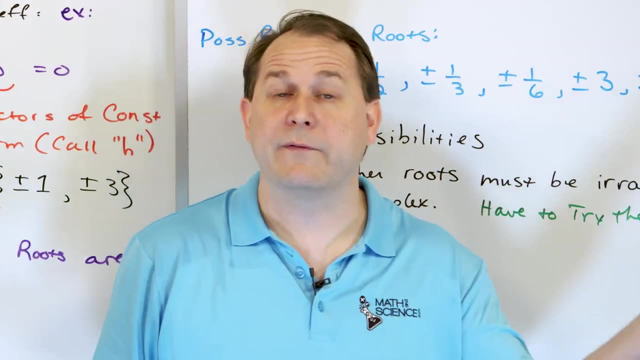 it in this polynomial, see if it equals zero. Then I have plus or minus one half. so I put one half in here, cube it and all this stuff, and see if it equals zero. Negative one half, put it in here, see if it equals zero. And I could go through all 12 of them I might. 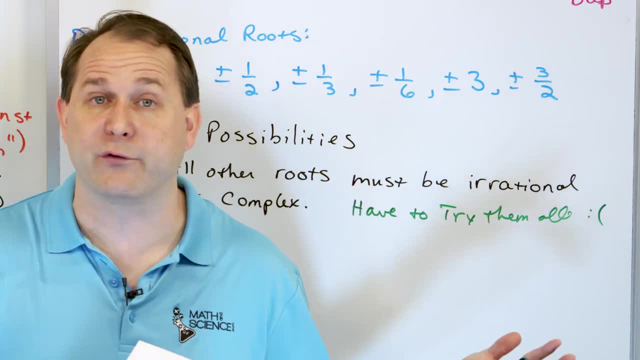 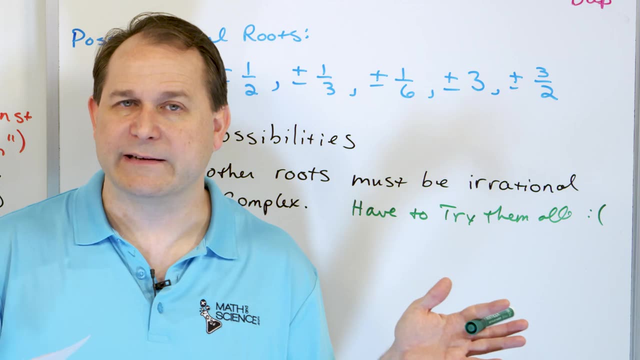 figure out because it's a third order polynomial. I might find that all three of the roots are actually in this list, And I'm done, But maybe I'll only find out that one of them is in this list, Or something like this, Because you could have complex roots as well, which 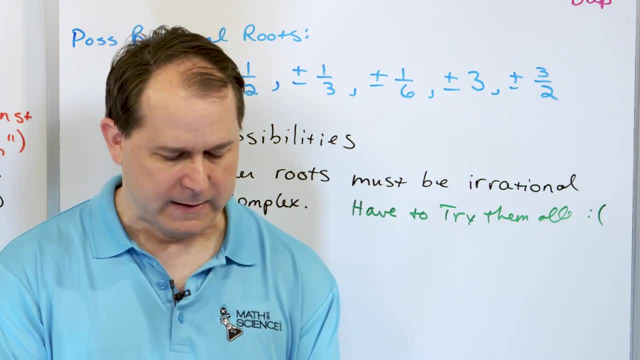 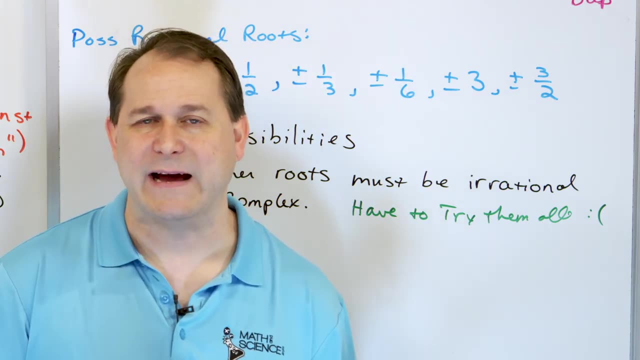 this doesn't help you. It only helps you with the rational roots- Then you might say, well, if it doesn't help you with all of the roots, then why do we even learn this thing? And for that I need to do a real example problem to show you how you can use this to help. 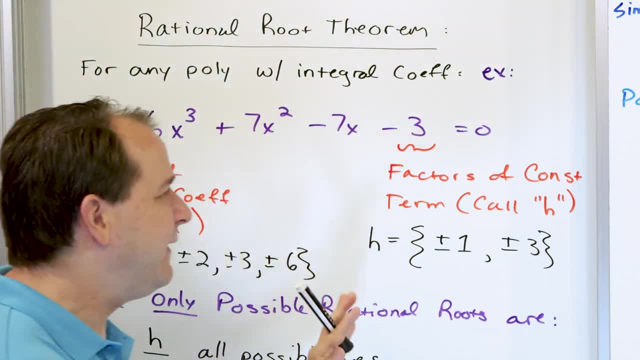 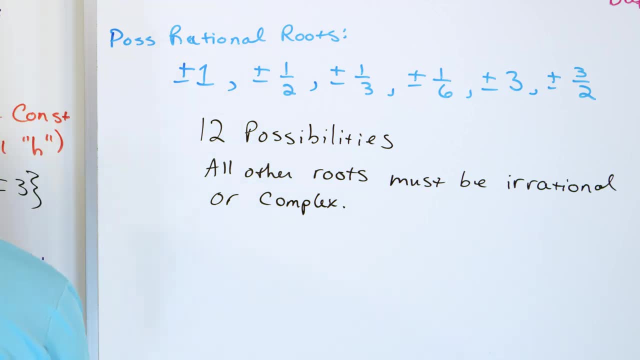 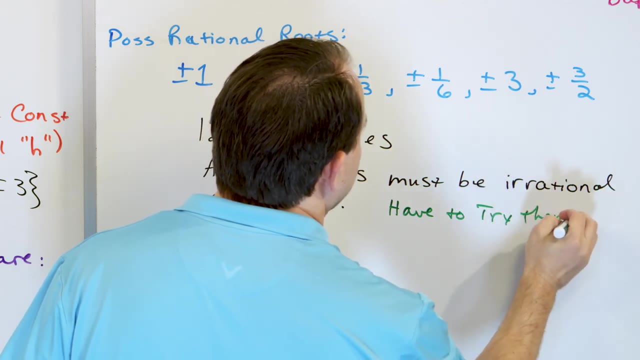 Obviously, the equation is only a third order equation. There can only be three roots total. How can I find out which of these, if any of them, actually are a root of that? Well, unfortunately you have two. You have to try them all. 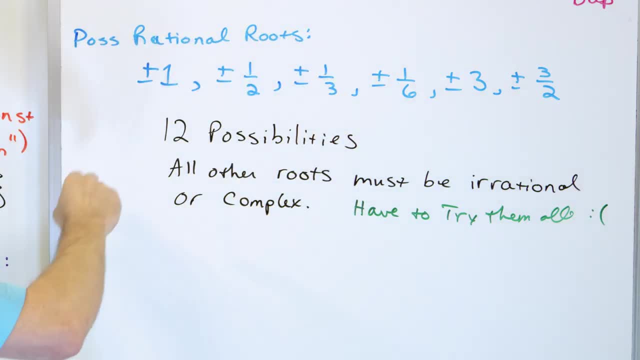 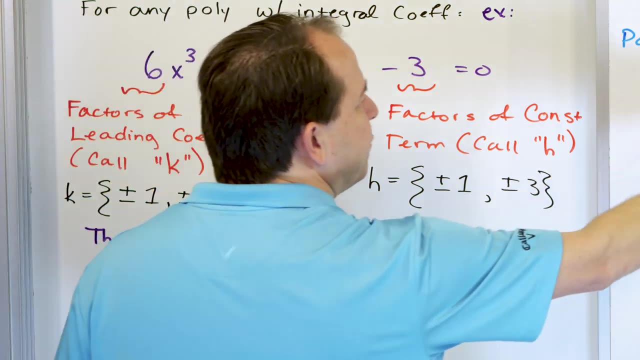 And that is not fun, right? Because that means you have to take the number 1 and stick it into this polynomial: see if it equals 0.. Take negative 1, put it in this polynomial: see if it equals 0.. 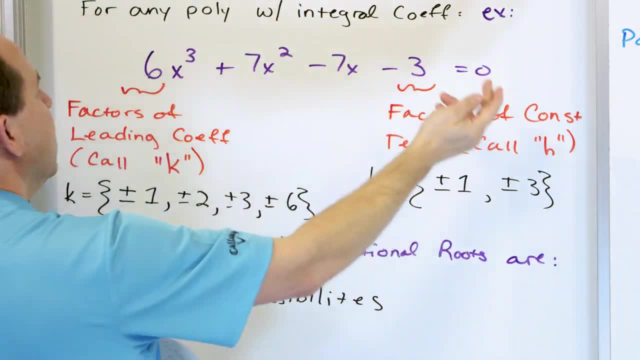 Then I have plus or minus 1 half. so I put 1 half in here, cube it and all this stuff and see if it equals 0.. Negative 1 half: put it in here, see if it equals 0.. 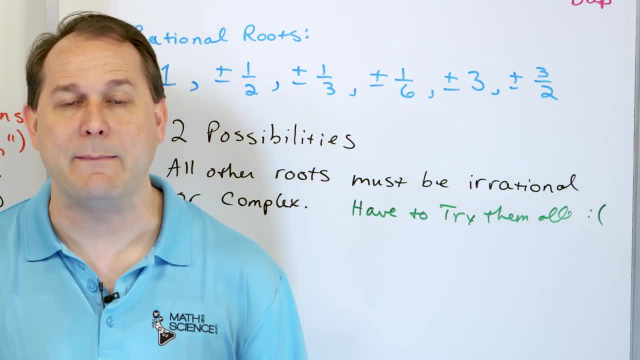 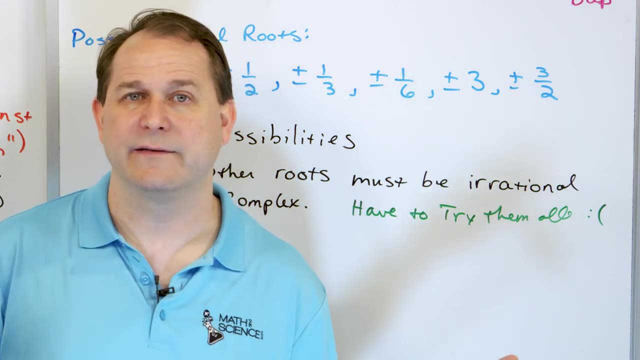 And I could go through all 12 of them, I might figure out, because it's a third order polynomial. I might find that all three of the roots actually are in this list, Then I'm done. But maybe I'll only find out that one of them is in this list. 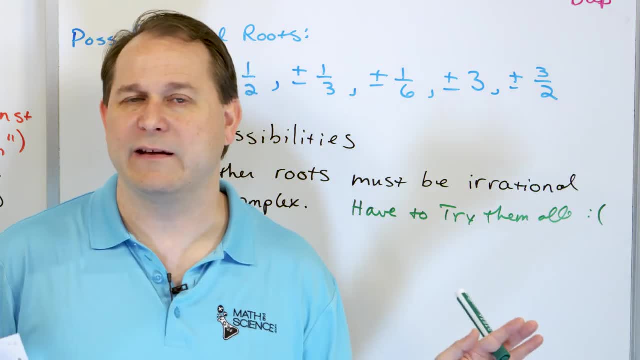 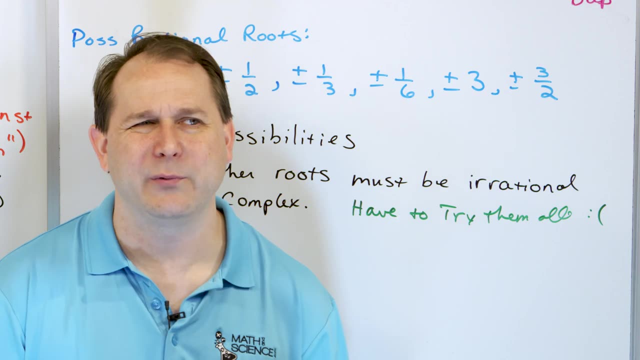 or something like this, Because you could have complex roots as well, which this doesn't help you. It only helps you with the rational roots. Then you might say: well, if it doesn't help you with all of the roots, then why do we even learn this thing? 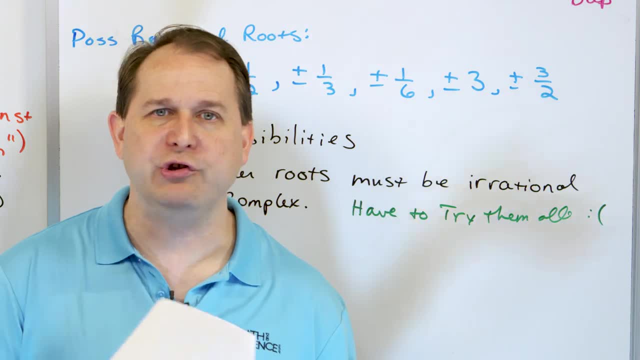 And for that I need to do a real example problem to show you how you can use this to help. even if it doesn't give you all of the answers, it could still be very useful. So this was a larger equation, because you 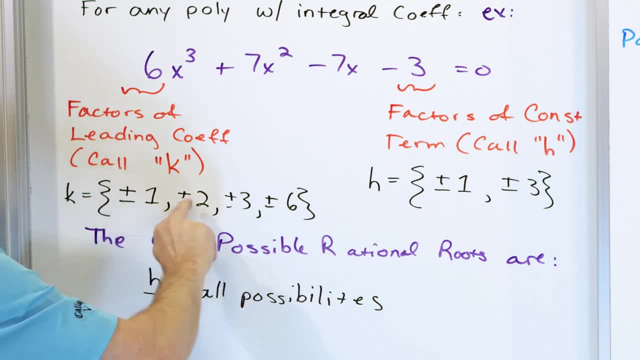 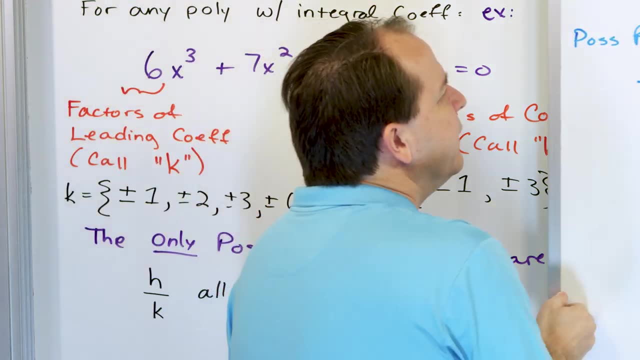 had big coefficients here, especially this one to give you a long list of numbers. The smaller the numbers you're going to have, the smaller the number of factors and the easier the problem is going to be. So let's crawl before we can walk. 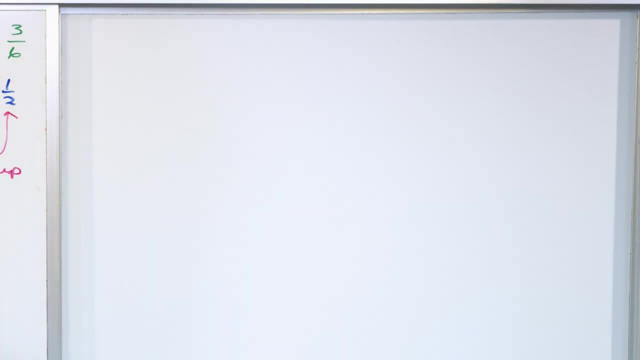 Now that we know how to figure out what the possibilities are, let's do a real problem. The problem basically says: I want to solve, And your problem will say something like this: Solve the following polynomial x cubed minus 7x plus 6.. 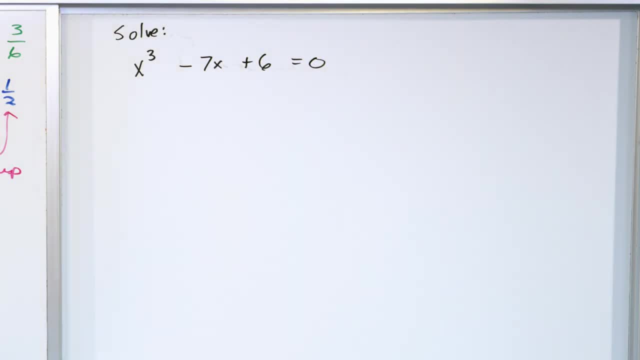 And obviously we're finding the roots, so we're going to set it equal to 0.. So you want to solve this Now you know that there's three roots, So you know that there can be some rational roots in there. 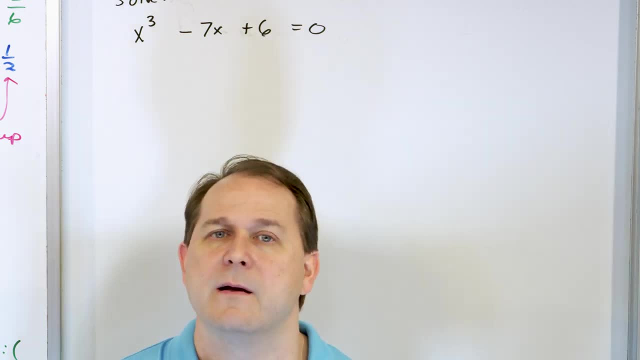 There can be some irrational roots in there, There can be some complex roots in there. But you know you could do Descartes' rule of sines if you wanted to and it would tell you how many positive and negative roots you have. 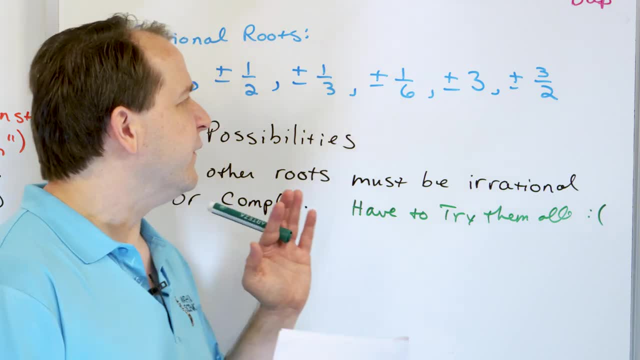 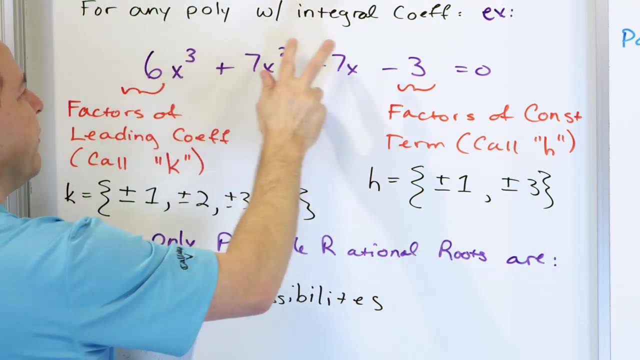 Even if it doesn't give you all of the answers, it can still be very useful. This was a larger equation Because you had big coefficients here, especially this one to give you a long list of numbers. The smaller the numbers you're going to have, the smaller the number of factors and the 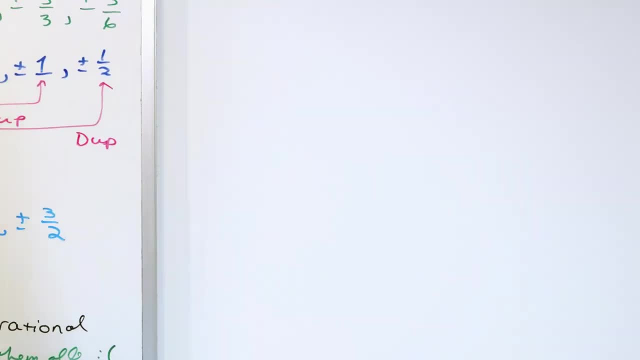 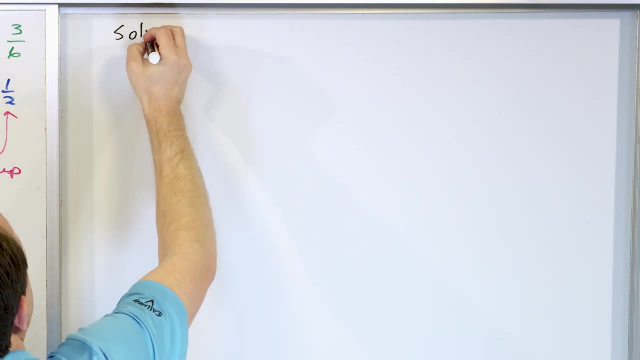 easier. the problem is going to be. So let's crawl before we can walk. Now that we know how to figure out what the possibilities are, let's do a real problem. The problem basically says: I want to solve, And your problem will say something like this: Solve the following. 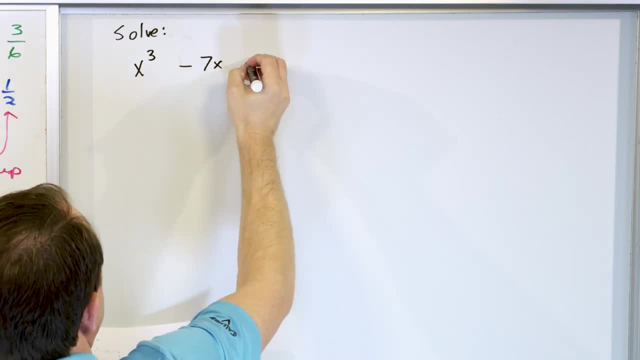 polynomial x cubed minus 7x plus 6.. And obviously we're finding the root, So we're going to set it equal to zero. So you want to solve this. Now you know that there's three roots, So you know that there. 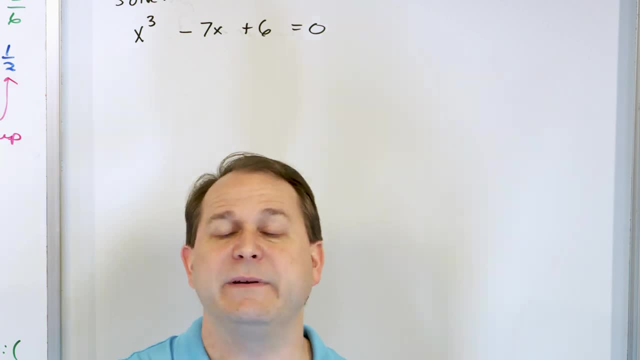 can be some rational roots in there, There can be some irrational roots in there, There can be some complex roots in there. But you know you could do Descartes' rule of sines if you wanted to And it would tell you how many positive and negative roots you have. 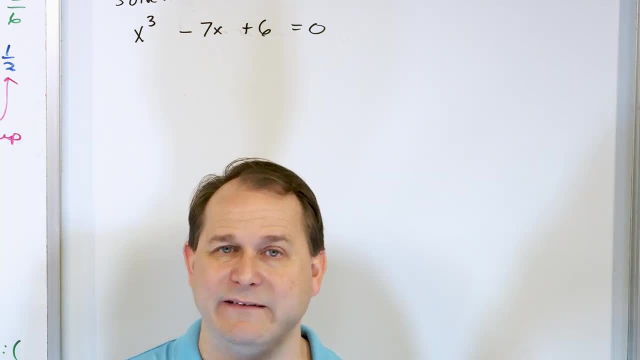 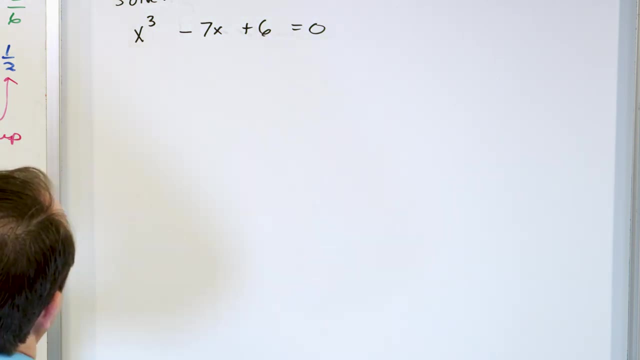 We're not going to do that. We already learned that skill. Now we're going to go and try to figure out and see if we can find out what roots are. actually satisfied this guy? Which means when it says solve it, it means find all the roots, All right. So the way we're 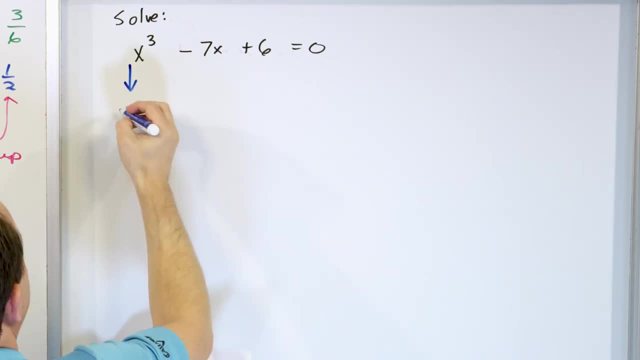 going to do. this is: the factors of this thing are plus or minus the coefficient in front, plus or minus 1.. That's the only factors of 1 is the number 1 itself. You might say: why is negative 1 a factor? Well, negative 1 times negative 1 would give me positive 1.. So it's. 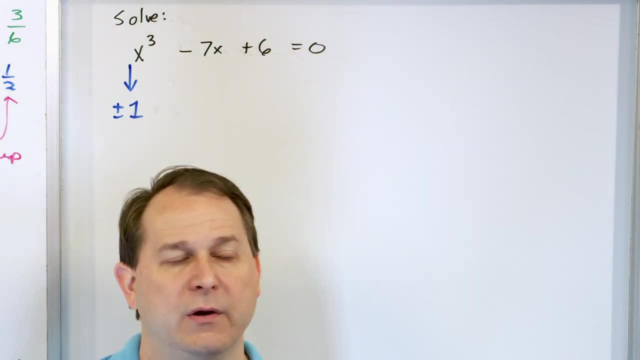 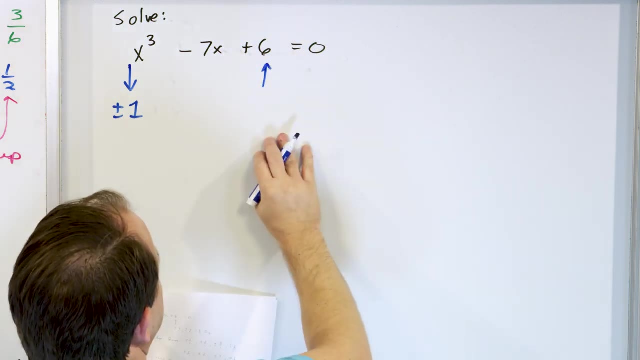 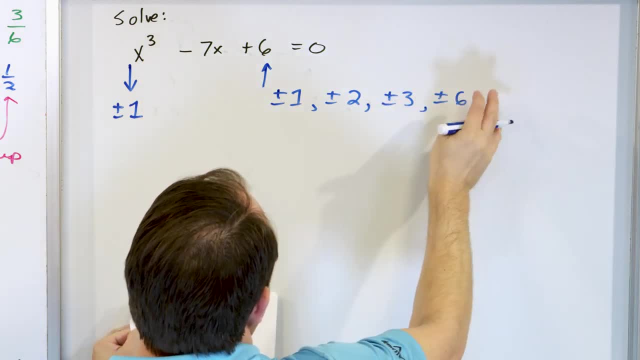 Plus or minus 2,, plus or minus 3, and plus or minus 6.. Those are the only factors. There's 2 times 4 is 8.. There's 8 of them, right? But in order to figure out what the rational. 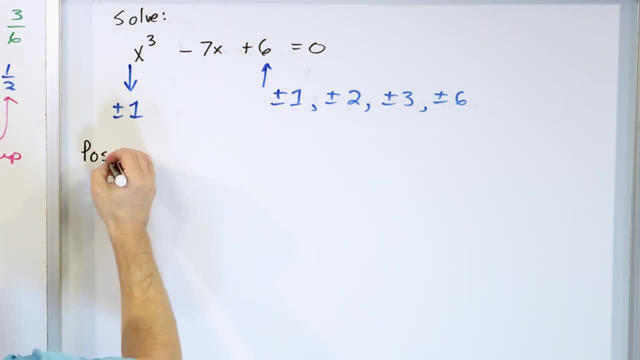 root possibilities are the possible rational roots, the rat roots. I call it rat roots, but whatever It's called rational roots, It's going to be these factors divided by these factors, which is exactly what we did. We did essentially. let me just double check. 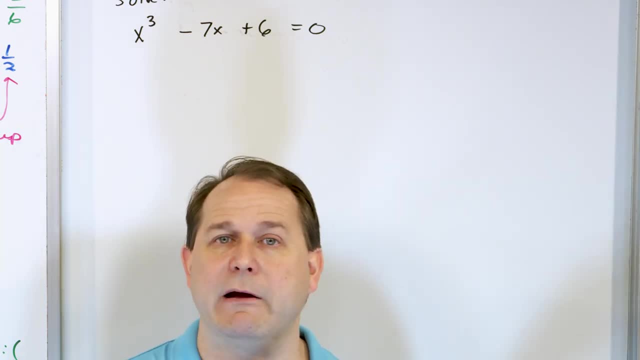 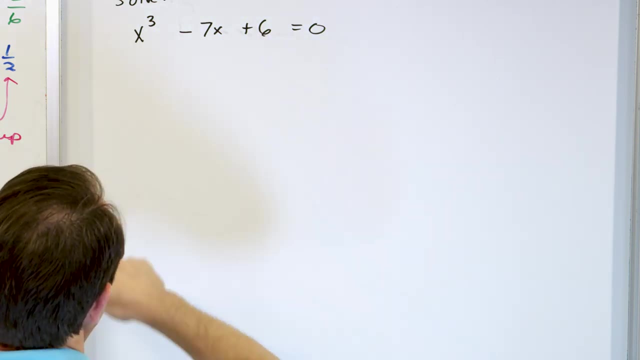 We're not going to do that. We already learned that skill. Now we're going to go and try to figure out and see if we can find out what roots are actually satisfied with this guy's. which means when it says solve it, it means find all the roots. 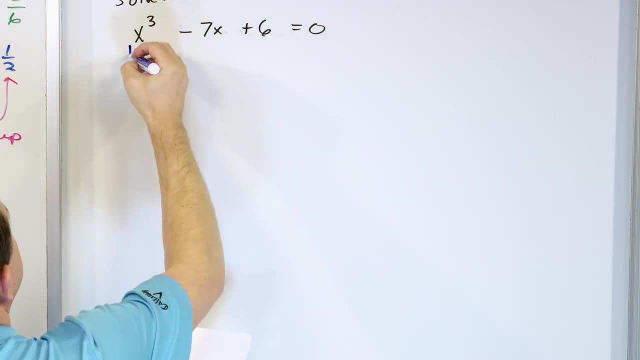 All right. So the way we're going to do this is the fact that we're going to do this. the factors of this thing are plus or minus, the coefficient in front, plus or minus 1.. That's the only factors of 1 is the number 1 itself. 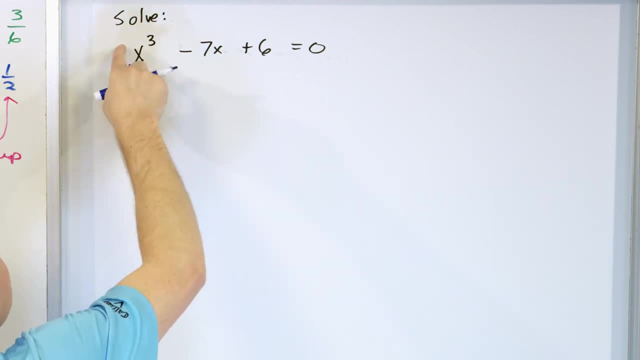 You might say: why is negative 1 a factor? Well, negative 1 times negative 1 would give me positive 1.. So it's a factor, if you can find anything at all, to multiply by it to give you what you have. 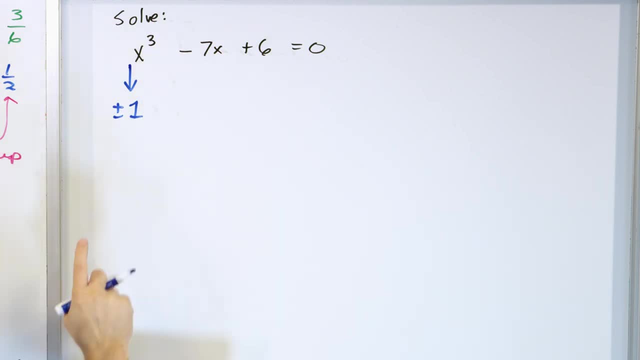 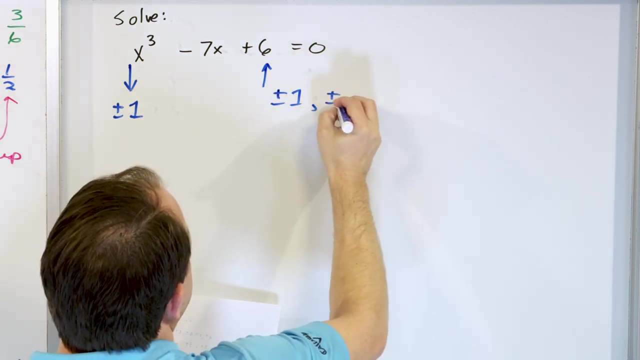 So the factors of this- you're always going to have plus or minuses any time you write it down- is 1.. Now the factors of this guy. we just wrote the list down, so we're very familiar. It's plus or minus 1,. plus or minus 2,. 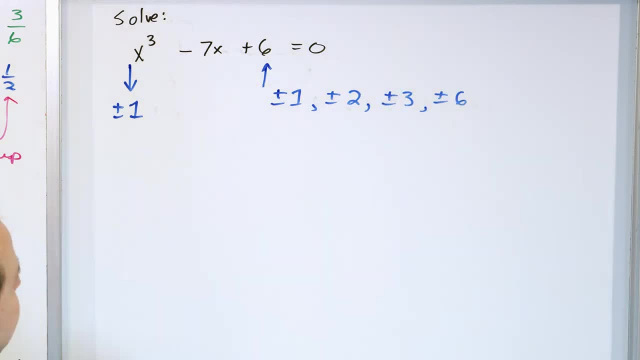 plus or minus 3, and plus or minus 6.. Those are the only factors. There's: 2 times 4 is 8.. There's 8 of them, right, But in order to figure out what the rational root possibilities are, the possible rational roots, the rat roots: 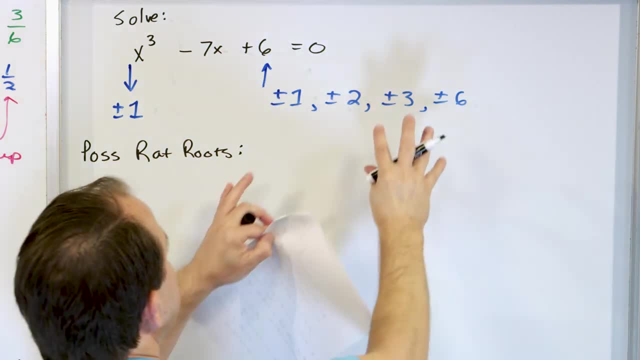 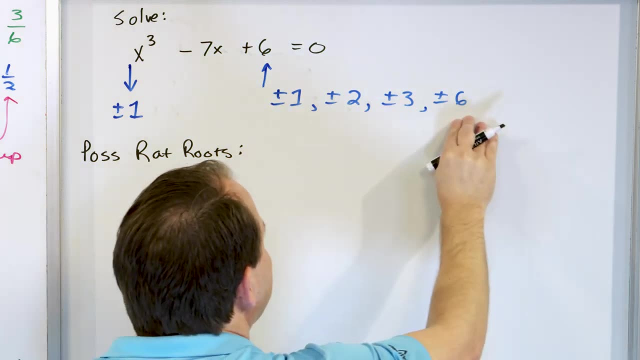 I call it rat roots, but whatever it's called rational roots is going to be these factors divided by these factors, which is exactly what we did. We did essentially. let me just double check h over k, So these were called the h factors. 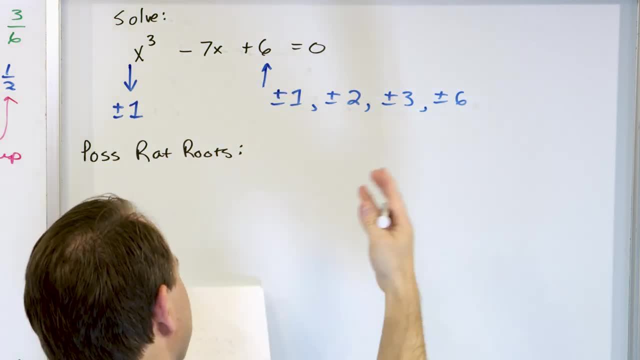 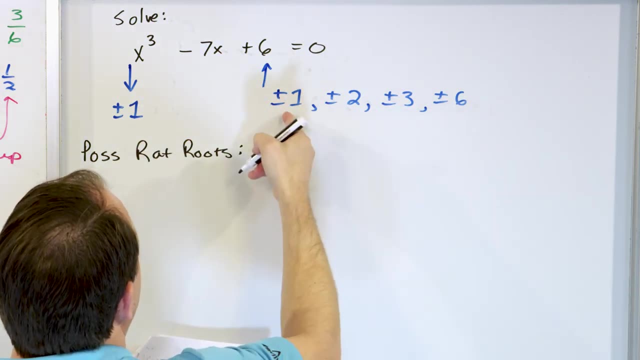 These were called the k factors, So h over k. But we're getting a little bit into solving the problem. You don't have to write h and k down all the time, You just list the factors. list the factors and then we say that we're going to have plus or minus 1 over 1.. 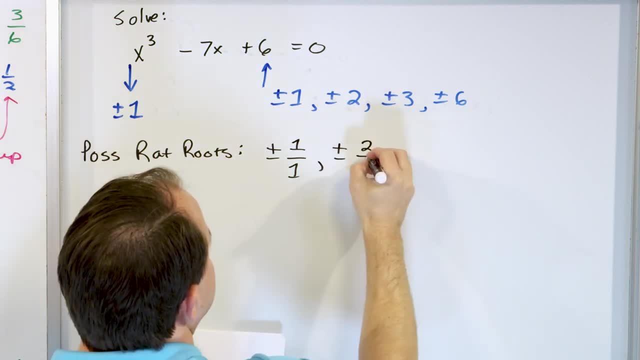 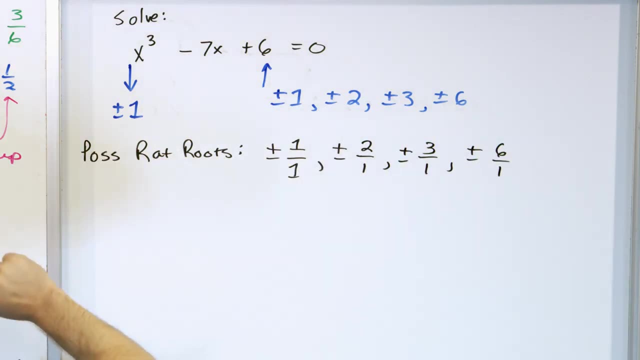 Then we can have plus or minus 2 over 1, plus or minus 3 over 1, plus or minus 6 over 1.. Because this only had really two factors anyway. so you're taking each of these and dividing by this. 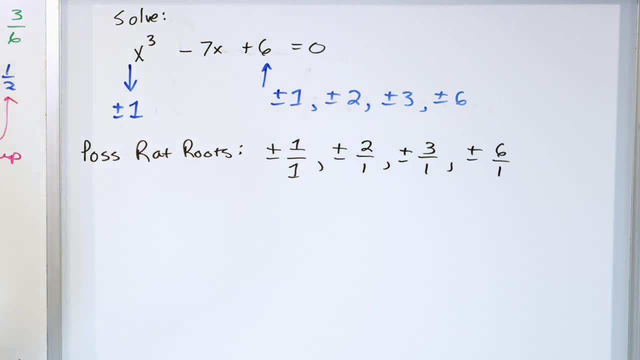 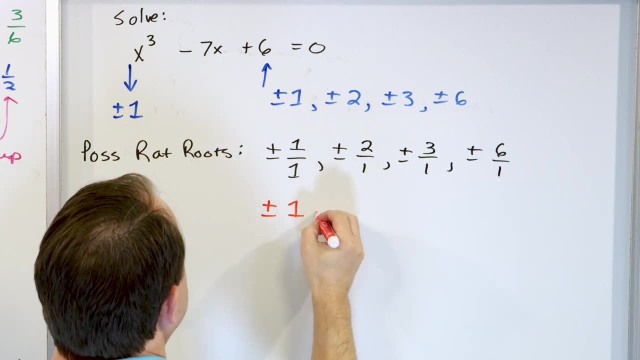 so the list is much shorter than it was in the previous problem. Now we can simplify this list By just looking at it and saying: we can simplify it by plus or minus 1, over 1 being 1, plus or minus 2,. 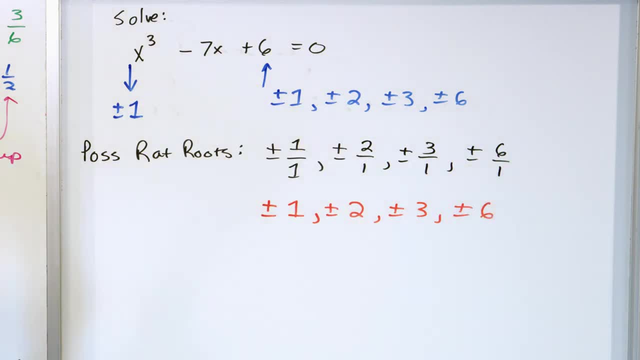 plus or minus 3, plus or minus 6.. So here we have a situation that's just kind of nice because we have a third order, polynomial. We know we're going to have three roots total. Some can be complex, of course, or irrational. 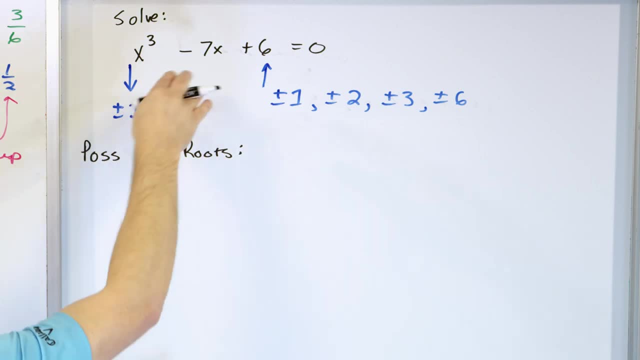 h over k. These were called the h factors, These were called the k factors- h over k. But we're getting a little bit into solving the problem. You don't have to write h and k down all the time, You just list the factors. list the factors And then we say that we're going. 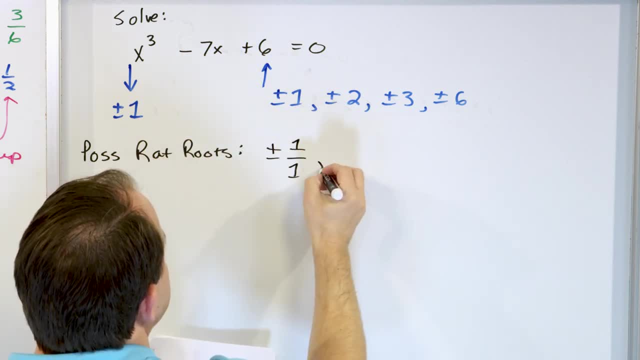 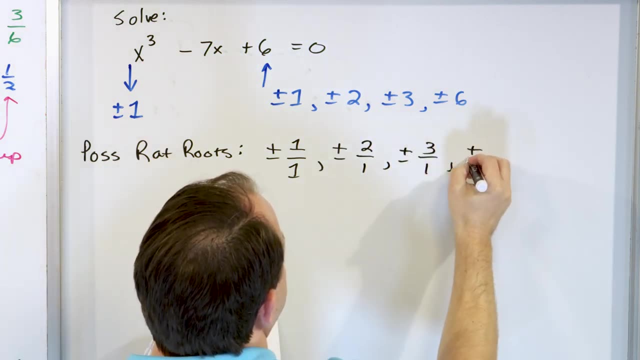 to have plus or minus 1 over 1.. Then we can have plus or minus 2 over 1, plus or minus 3 over 1, plus or minus 6 over 1.. Because this only had really two factors anyway. So 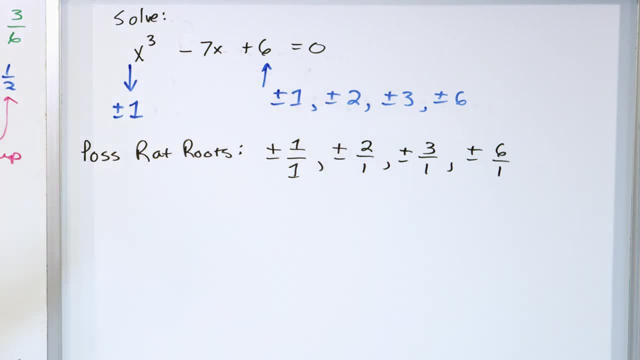 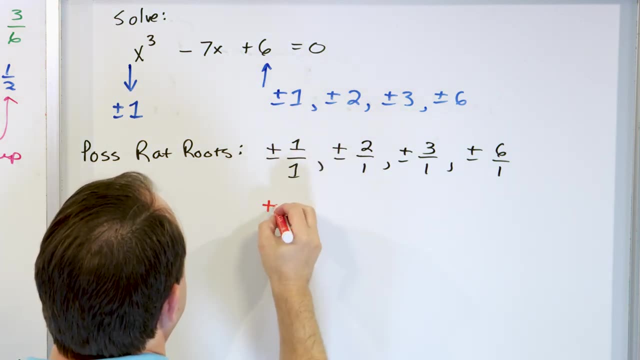 you're taking each of these and dividing by this, So the list is much shorter than it was in the previous problem. Now we can simplify this list by just looking at it and saying: we can simplify it by plus or minus 1 over 1 being 1, plus or minus 2, plus or minus 3, plus or minus 6.. So here, 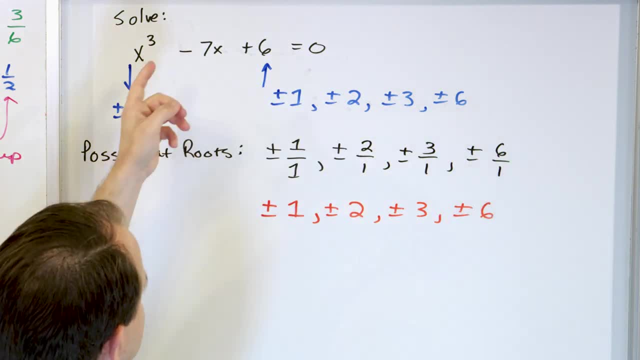 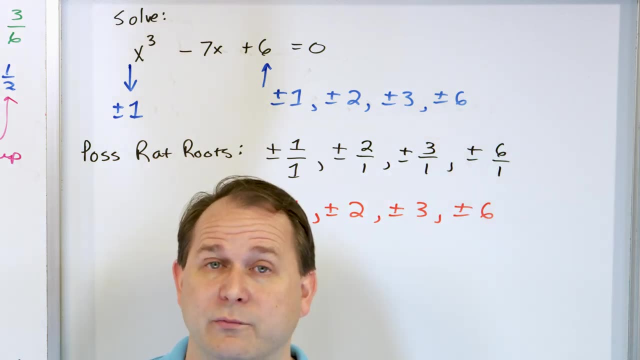 we have a situation that's just kind of nice Because we have a third order polynomial. we know we're going to have three roots total. Some can be complex, of course, or irrational, We don't know yet- But we know some could be rational, which means they're numbers. 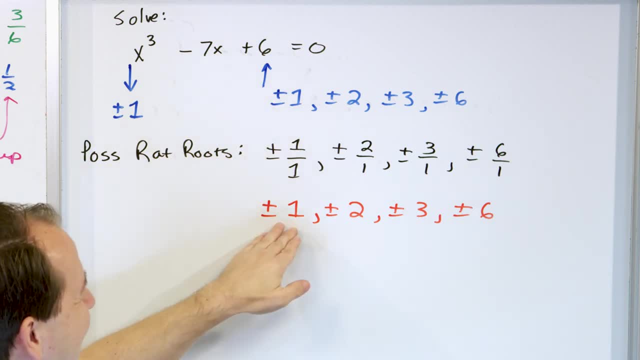 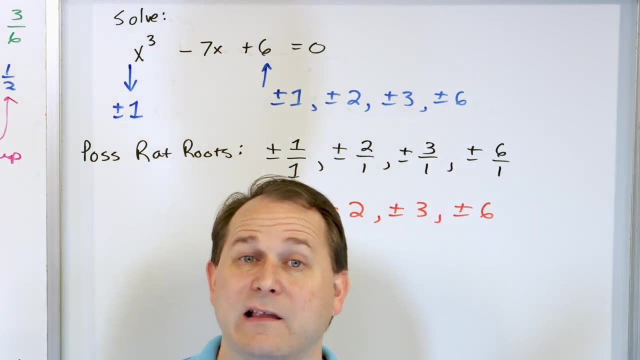 or fractions, But we know that if it has any rational roots at all, it has to be in this list. So there's 4 times 2, 8 possibilities here. So really, if you had lots of time on your hands or a computer on your hands, what you would do is take every one of these things. 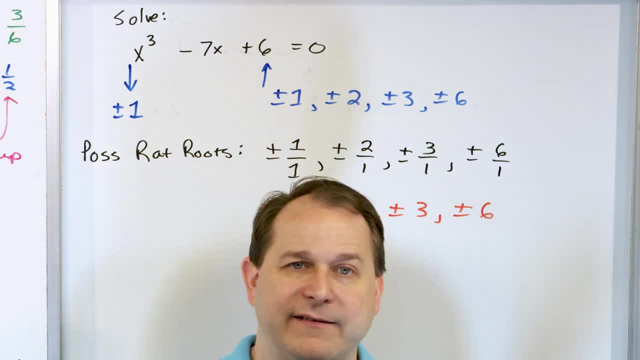 and put it into the equation and see if it equals 0. That's going to totally find out if all of them are rational. It's going to figure out all of the rational roots because you're going to substitute every last one of them. But you can see that that strategy 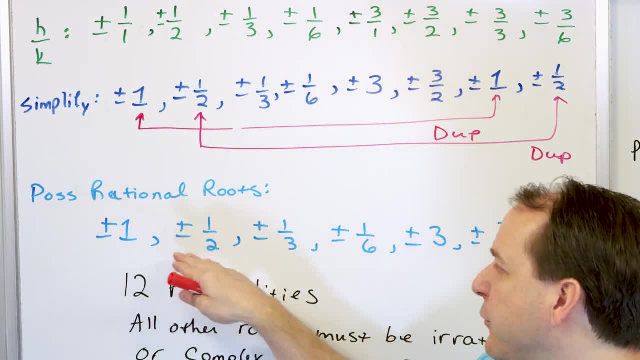 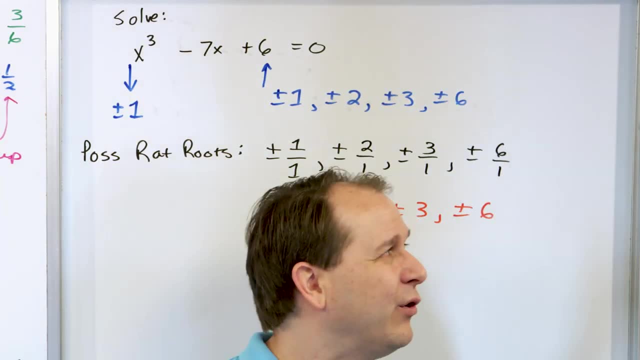 is going to get really cumbersome as we get larger problems And you have to start substituting all these fractional ones in there. So what I want you to do, what most teachers or most books will tell you to do, is don't try to substitute every one of these things in there. Just pick the easy one. The easy. 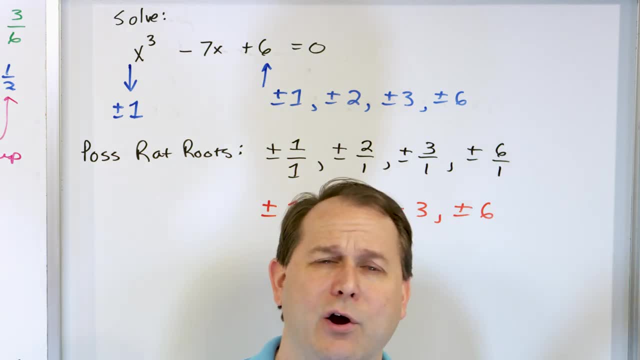 one is going to be 1.. Usually- not always, but actually always- you're going to have plus or minus. 1 is a possible rational root, because every number has a factor of 1.. So you're always going to have plus or minus 1.. And you can, of course, substitute plus. 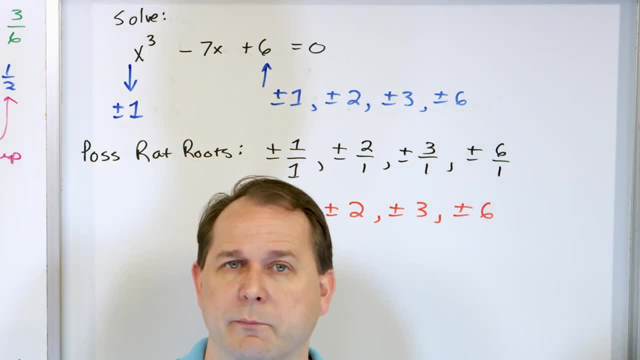 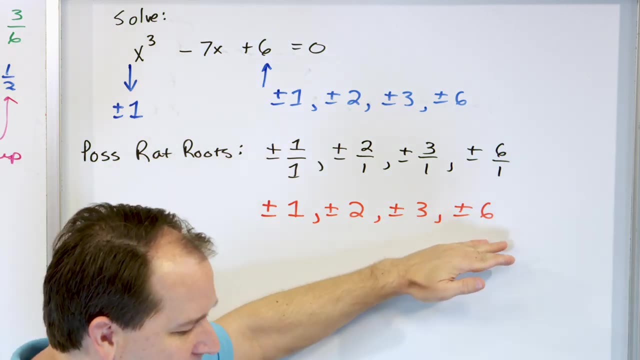 We don't know yet, but we know some could be rational, which means they're numbers or fractions. But we know that if it has any rational roots at all, it has to be in this list. So there's 4 times 2, 8 possibilities here. 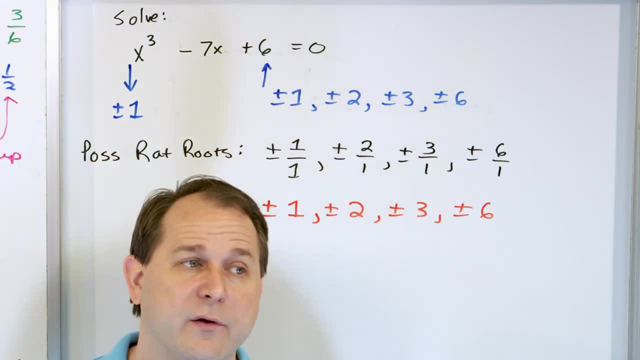 So really, if you had lots of time on your hands or a computer on your hands, what you would do is take every one of these things and put it into the equation and see if it equals 0. That's going to totally find out if all of them are rational. 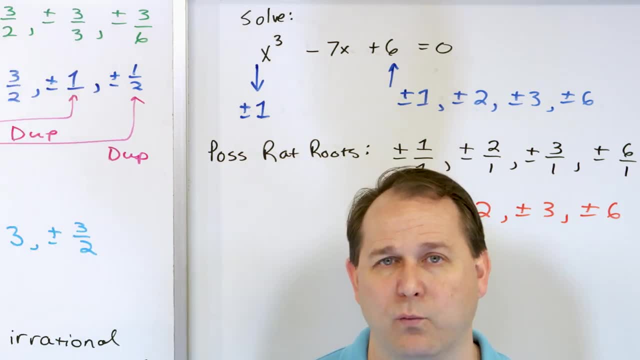 It's going to figure out all of the rational roots because you're going to substitute every last one of them. But you can see that that strategy is going to get really cumbersome as we get larger problems and you have to start substituting all. 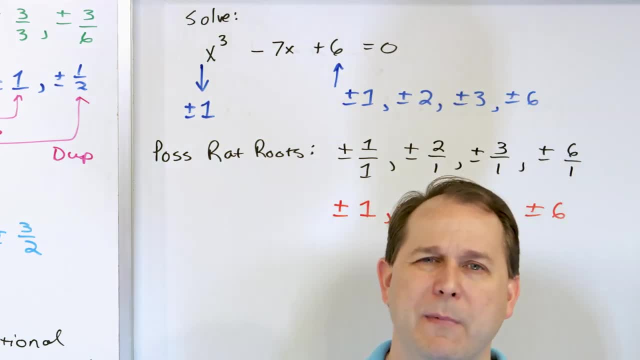 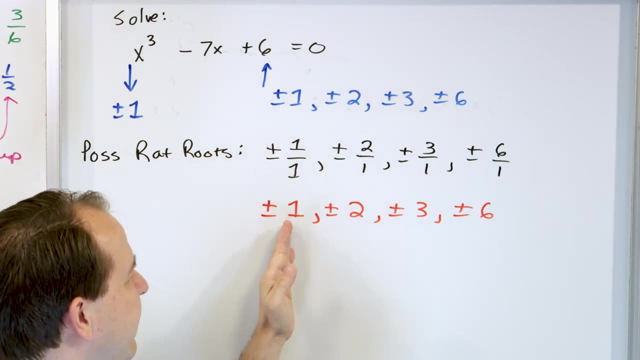 these fractional ones in there. So what I want you to do, what most teachers are, or what most books will tell you to do, is: don't try to substitute every one of these things in there. Just pick the easy one. The easy one is going to be 1.. 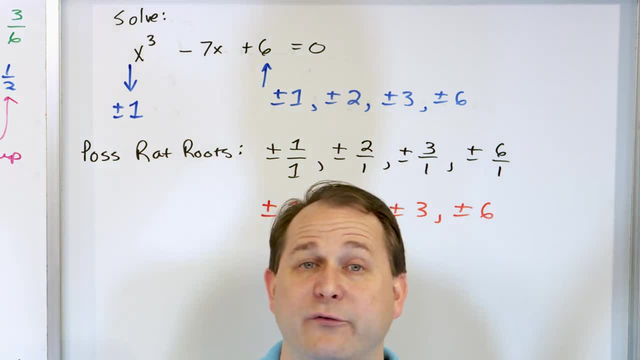 Usually- not always, but actually always- you're going to have plus or minus. 1 is a possible rational root, because every number has a factor of 1.. So you're always going to have plus or minus 1.. And you can, of course, substitute plus or minus 2.. 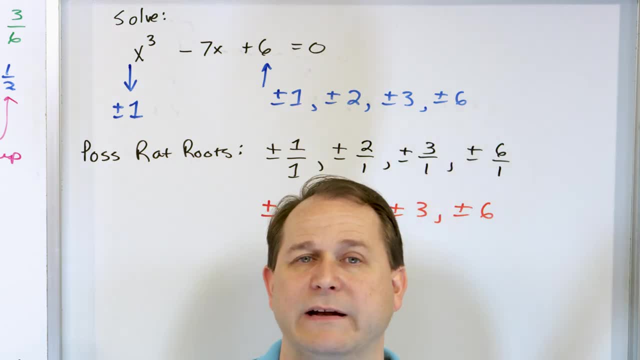 You can do that. There's nothing wrong with that. But always try to substitute plus or minus 1.. You might get lucky. If you get lucky, then I'm going to show you how to handle that, But let's go ahead and see what happens. 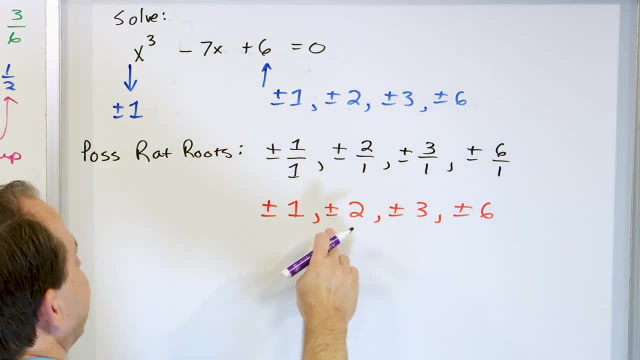 and see if we can avoid plugging in every last one of these things, Because for every time we do it we're going to have to square, cube it and all this other stuff to figure out if it's a root or not. 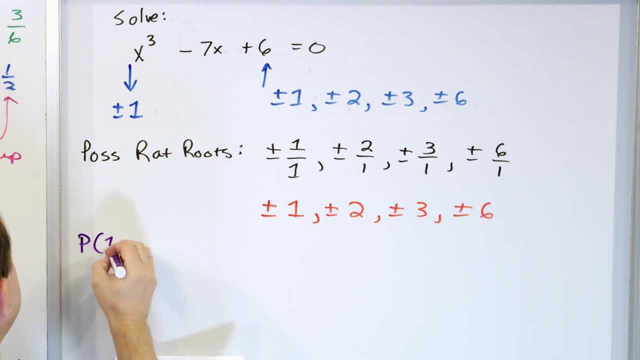 So we're going to plug in this polynomial evaluated at the number 1, because plus or minus 1 is the lowest root. Now, 1 cubed is what we're going to stick in there: Minus 7 times 1, right here, plus 6.. 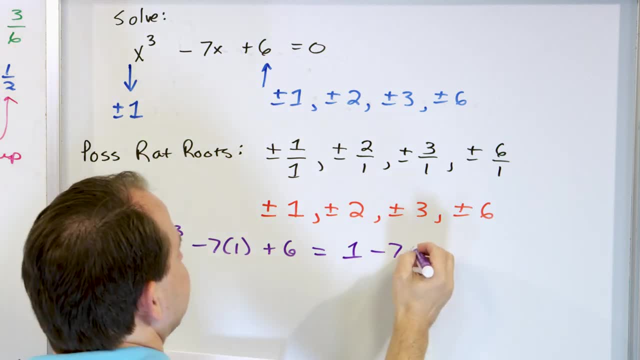 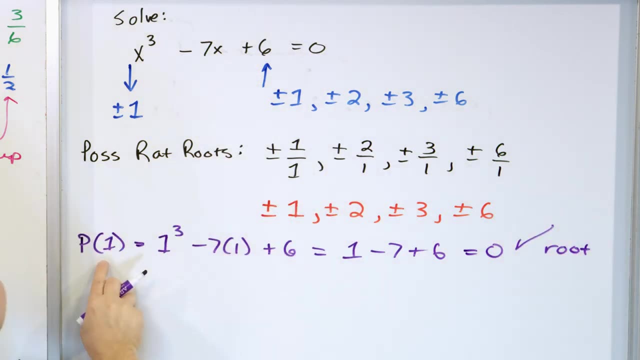 1 cubed is 1 minus 7 from this and then plus 6.. So the 1 plus 6 is 7, minus the 7 is 0. So it is a root. So you have figured out that the number 1 is actually a root. 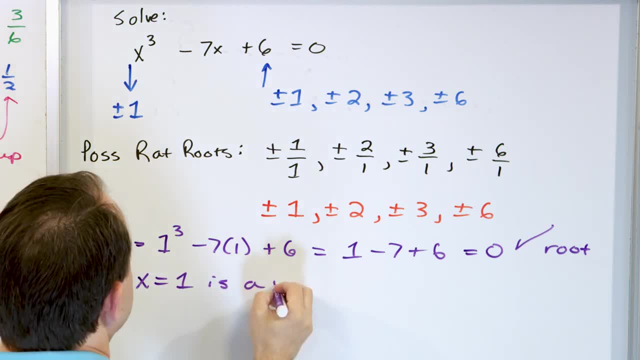 So x is equal to 1 is a root. Again, you got lucky. but reality is we choose the problem so that in the beginning you find out that that is a root. Now we have one of them down. We only have two left. 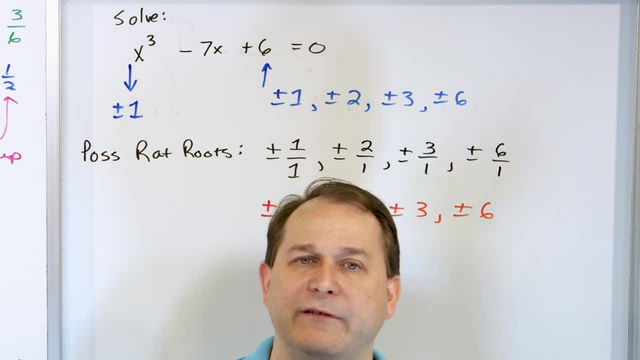 or minus 2.. You can do that- There's nothing wrong with that- But always try to substitute plus or minus 1.. You might get lucky, Right? If you get lucky, then I'm going to show you how to handle that. But let's go ahead. 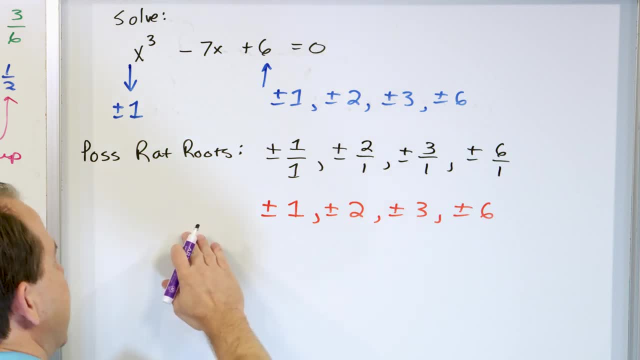 and see what happens and see if we can avoid plugging in every last one of these things, because for every time we do it we're going to have to square, cube it and all this other stuff to figure out if it's a root or not. 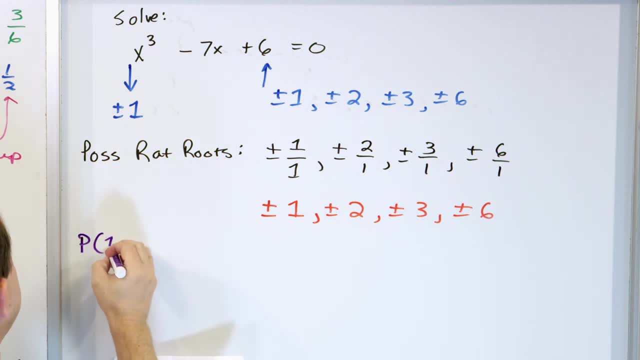 So we're going to plug in this polynomial evaluated at the number 1, because plus or minus 1 is the lowest root. Now 1 cubed is. we're going to stick in there minus 7 times 1, right here, plus 6.. 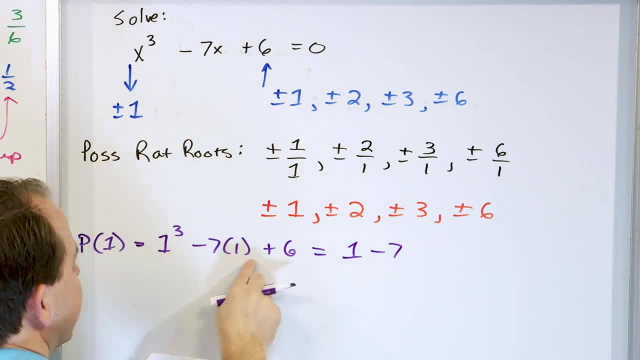 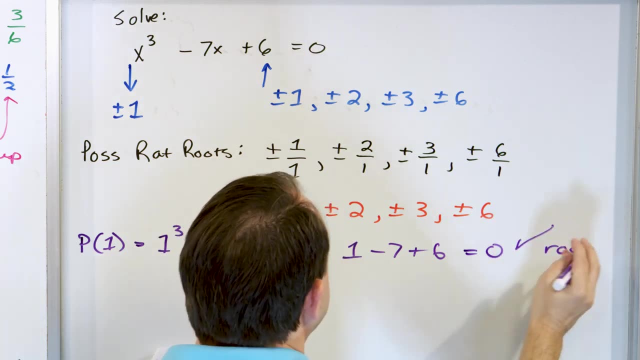 1 cubed is 1. Minus 7 from this and then plus 6. So the 1 plus 6 is 7, minus the 7 is 0. So it is a root. So you have figured out that the number 1 is actually a root. 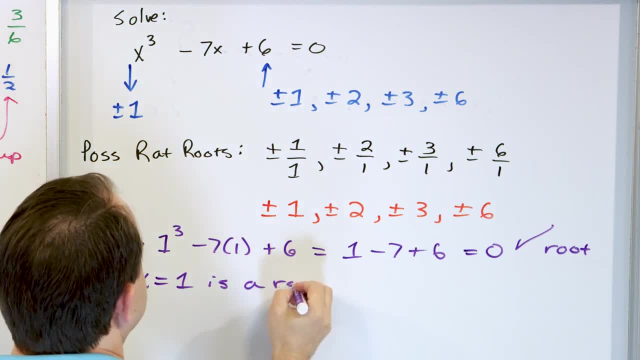 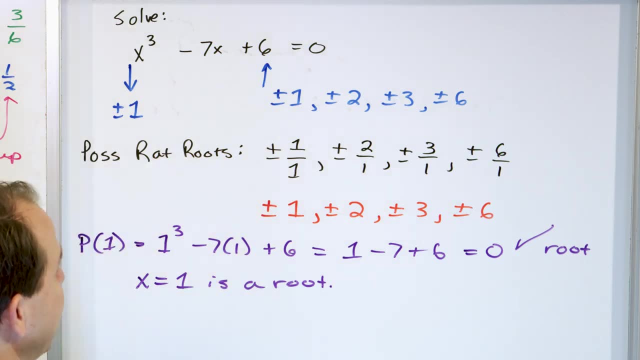 So x is equal to 1 is a root. Again, you got lucky. but reality is we choose the problem so that in the beginning you find out that that is a root. Now we have one of them down. We only have two left. 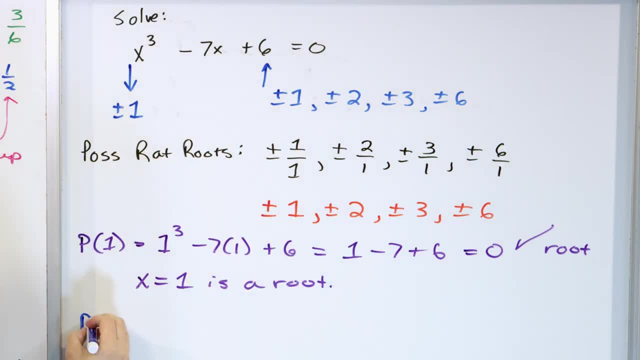 So maybe we'll get lucky again. Let's plug in negative 1.. Maybe it'll be a root as well, Maybe it'll be a negative 1.. So we put negative 1, cube it minus 7, negative 1, plus 6.. 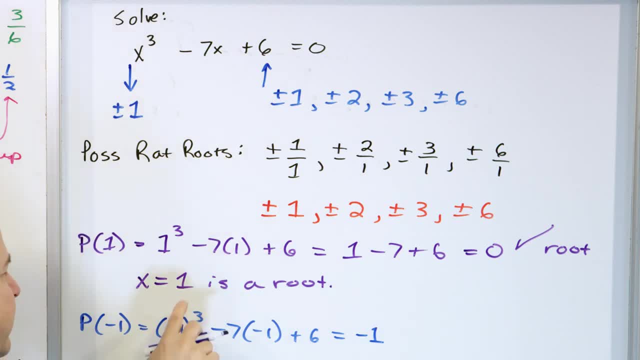 Now this negative 1 cubed evaluates to negative 1. Negative 1 times negative, 1 times negative 1. This becomes a positive 7. This becomes a positive 6,. right, So you can think of the 1 minus the 7, or negative: 1 plus the 7 is 6, and then plus. 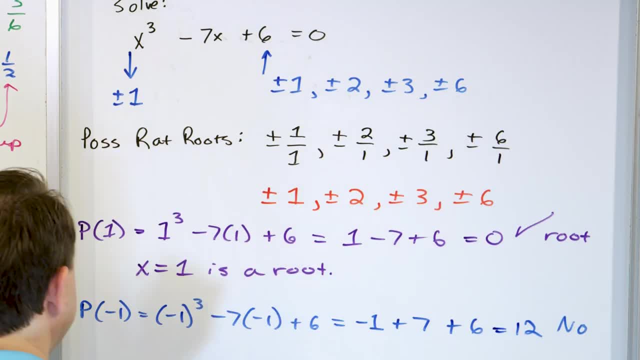 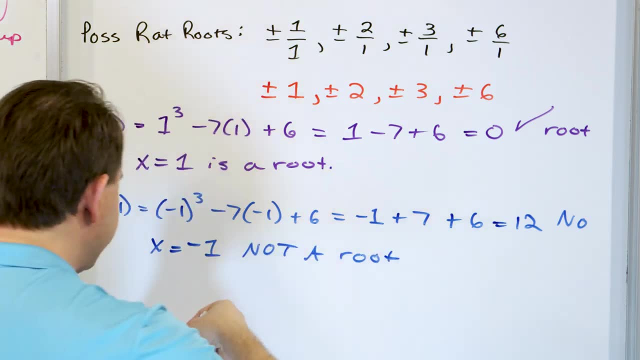 6 is 12.. So no, So we say that x is 0.. x is equal to negative 1, not a root. So you can see you're not going to get lucky all the time, right, It would be nice if everything had a root of plus or minus 1.. 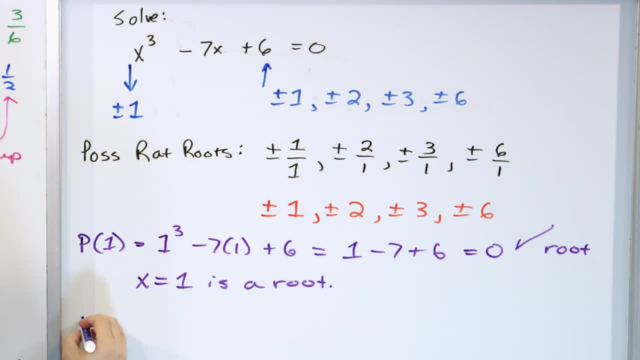 So maybe we'll get lucky again. Let's plug in negative 1.. Maybe it'll be a root as well. negative 1.. So we put negative 1.. Qubit minus 7, negative 1, plus 6.. Now this negative 1 cubed evaluates to negative 1.. 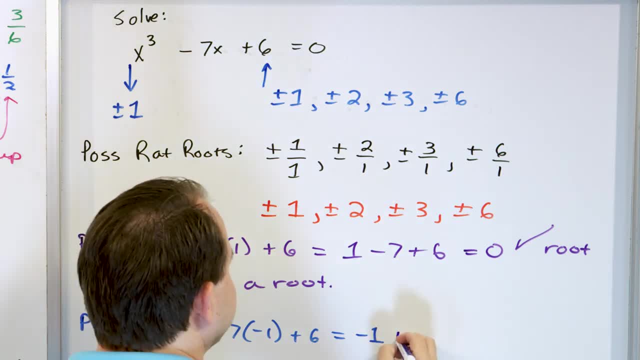 Negative, 1 times negative, 1 times negative: 1. This becomes a positive 7. This becomes a positive 6,. right, So you can think of the 1 minus the 7, or negative: 1 plus the 7 is 6, and then plus 6 is 12.. 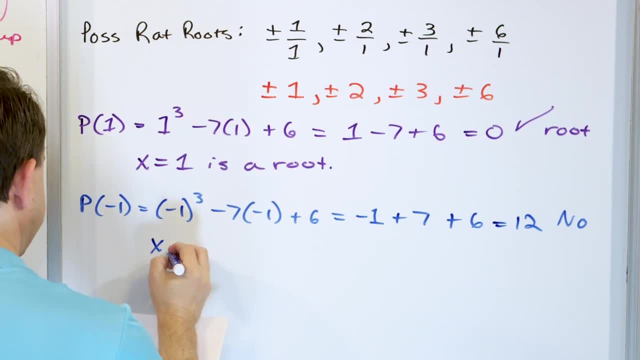 So no, So we say that x is equal to negative 1, not a root. So you can see you're not going to get lucky all the time, right, It would be nice if everything had a root of plus or minus 1.. 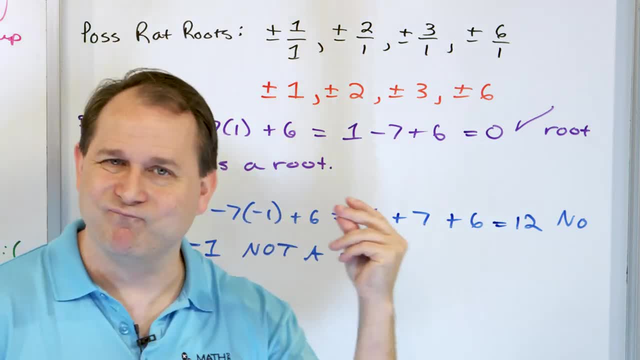 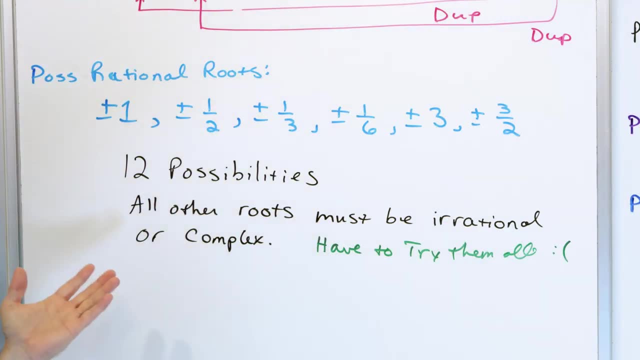 Those are easy numbers to calculate. Putting a number 1 in there is like really really simple. Putting a number 2 really isn't that hard. Putting 3 and all that isn't that hard. But what you're going to run into is in more complicated problems. 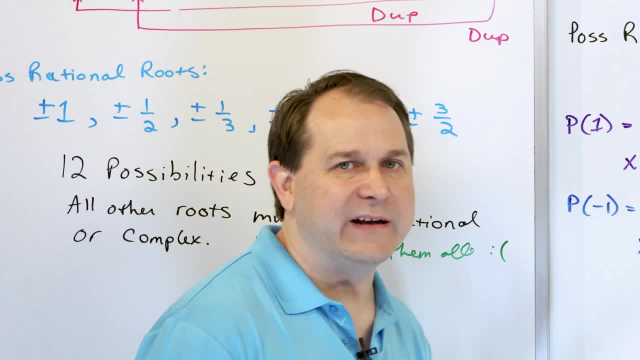 you're going to have to put in 1 half and 1 sixth and negative 1 sixth, So you have to cube it and then add it and then all the stuff with fractions, And so you're going to have to do a lot of work. 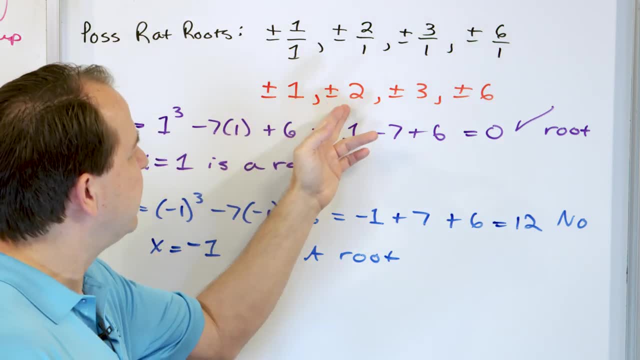 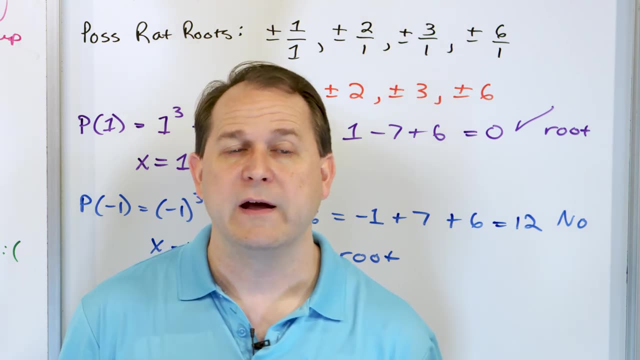 So what I want you to do is go ahead and try to substitute and keep going up your list until you find at least one of them that is a root, Because once you identify one of them as being a root, then we can use some tricks. 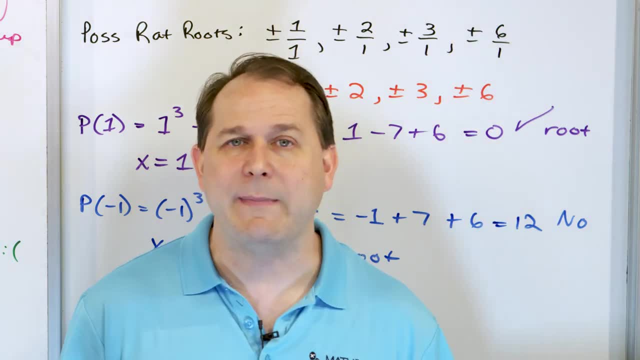 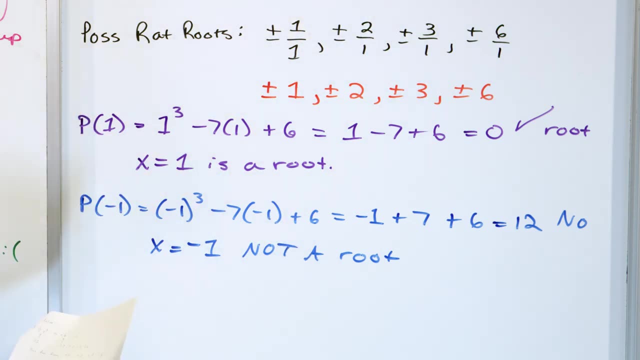 I don't want to like to call it a trick, but we can then find the remaining roots. By the way, I'm going to show you here in a second. We know that this guy's a root, So what does that actually mean? 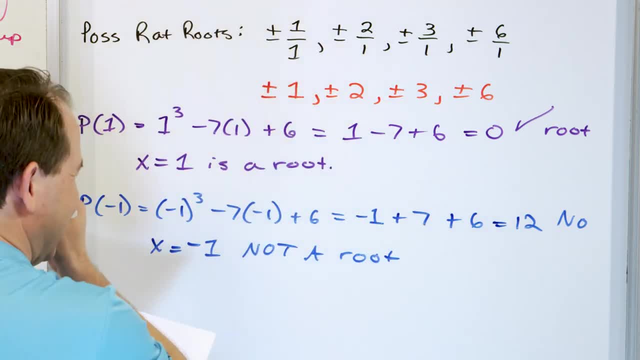 What does that actually mean? It means that if the equation I'm trying to decide if I want to even do this on this page or not, Yeah, I think I am going to do it on this page. So if x equals 1 is a root, then that: 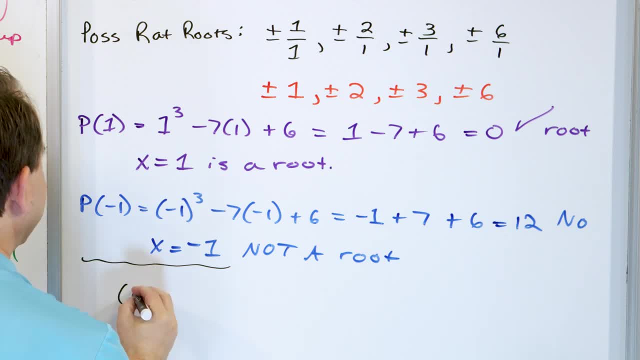 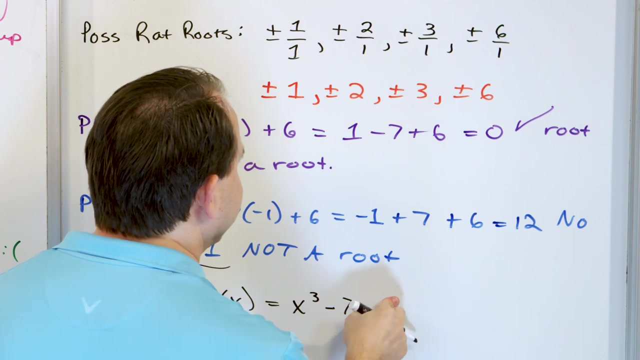 means this polynomial here can be written as a factored form of x minus 1 times some other factors of x And that's going to equal what this polynomial is. We've done this before And I realize some of you may not have seen those other lessons. 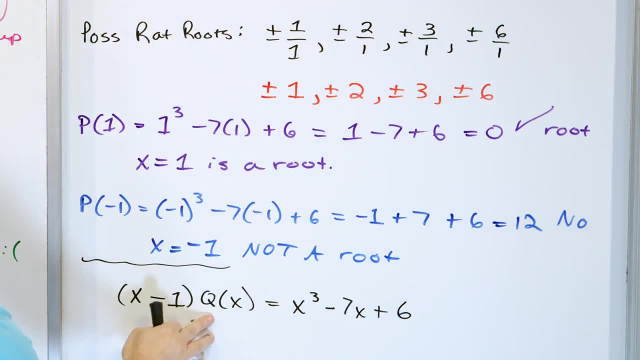 So I'm going to review it a little bit here, But the bottom line is we've actually done this before. If this looks foreign to you, then you probably should go back and look at the factor theorem and the remainder theorem. We've done the factor theorem and the remainder theorem. 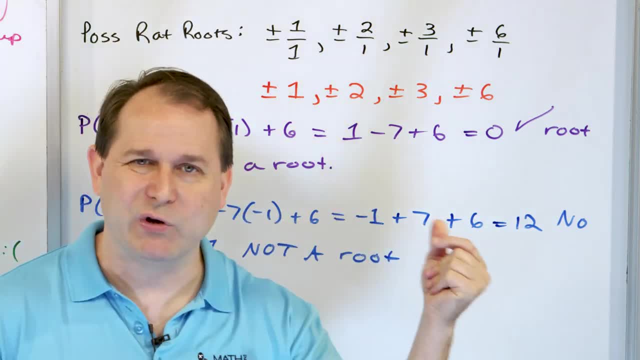 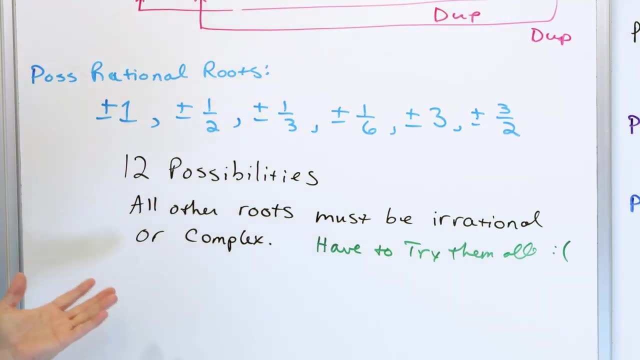 Those are easy numbers to calculate. Putting a number 1 in there is like really really simple. Putting a number 2 really isn't that hard. Putting 3 and all that isn't that hard. But what you're going to run into is in more complicated problems you're going to have 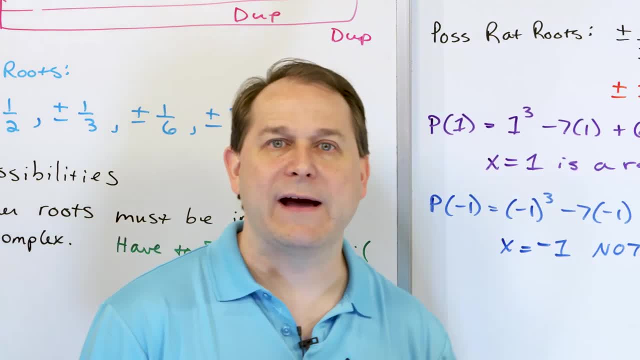 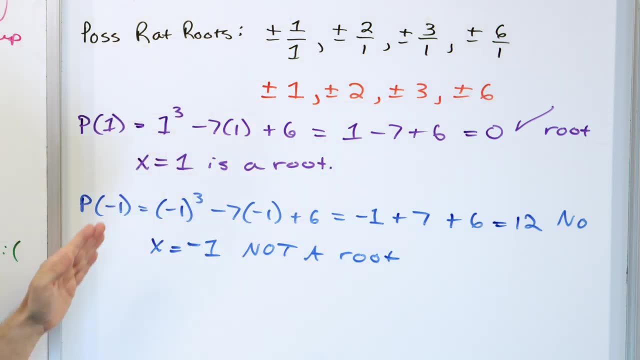 to put in 1 half and 1 sixth and negative 1 sixth. So you have to cube it and then add it, and then all this stuff with fractions, And so you're going to have to do a lot of work. So what I want you to do is go ahead and try to substitute and keep going up your list. 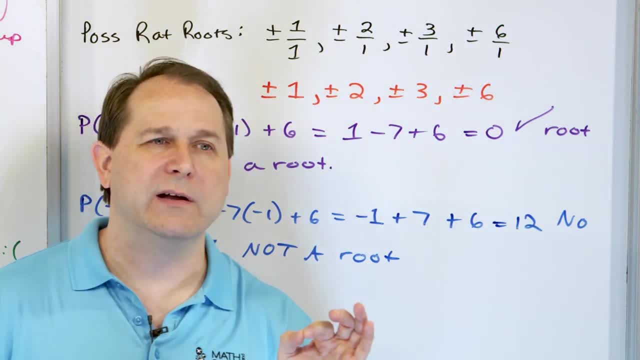 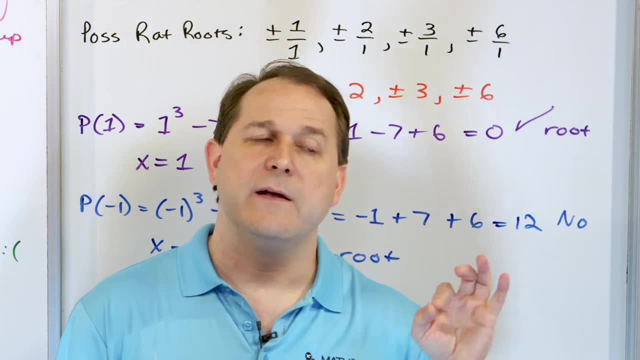 until you find at least one of them that is a root. Because once you identify one of them as being a root, then we can use some tricks. I don't want to like to call it a trick, but we can then find the remaining roots. 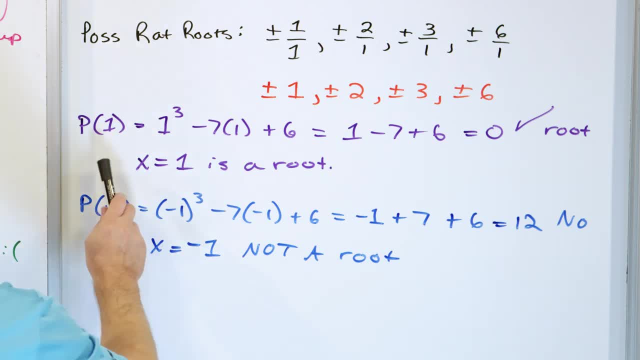 By the way, I'm going to show you here in a second. We know that this guy's a root. So what does that actually mean? right, What does that actually mean? It means that, if the equation I'm trying to decide, if I want to even do this on this- 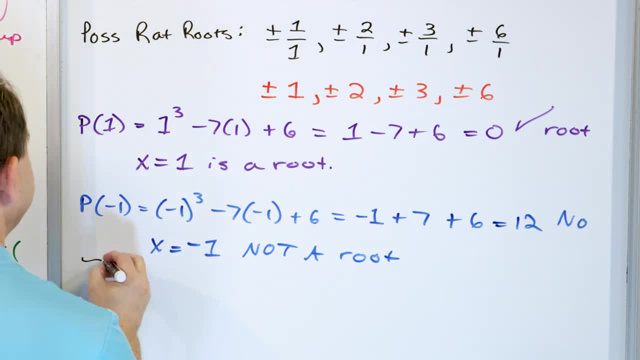 page or not? Yeah, I think I am going to do it on this page. If x equals 1 is a root, then that means this polynomial here can be written as a factored form of x minus 1 times some other factors of x. 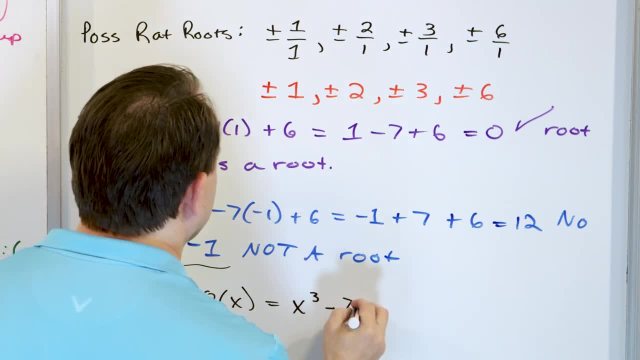 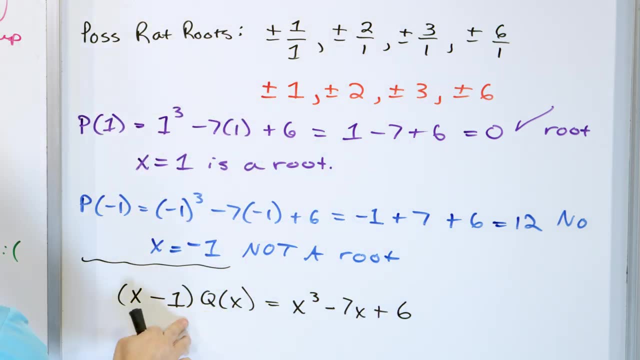 And that's going to equal what this polynomial is. We've done this before And I realize some of you may not have seen those other lessons, so I'm going to review it a little bit here. But the bottom line is we've actually done this before. 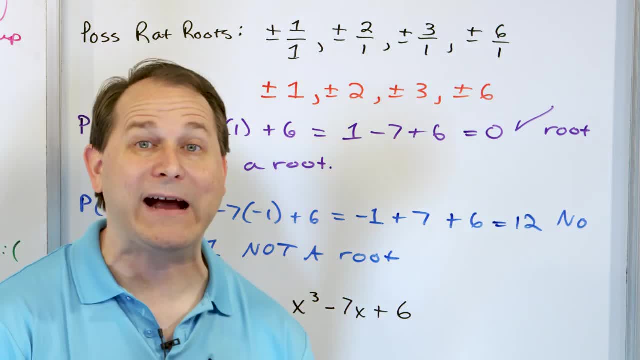 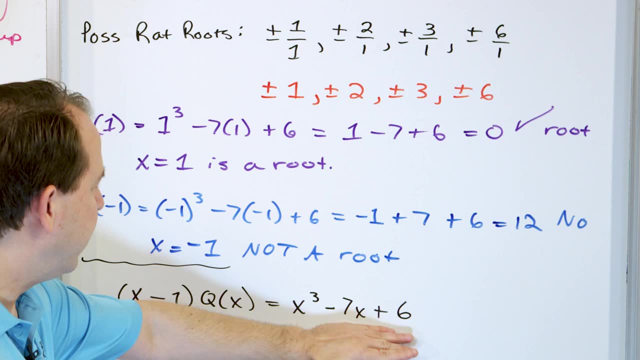 If this looks foreign to you, then you probably should go back and look at the factor theorem and the remainder theorem. We've done the factor theorem and the remainder theorem. We did problems like this before, But anyway, this is the polynomial given to us. 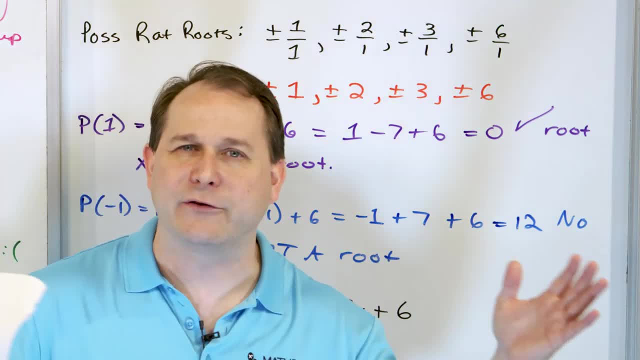 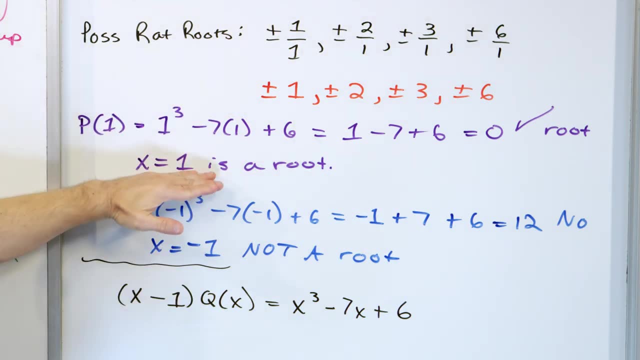 We know that if we knew all the roots, we should be able to write it in some kind of factored form, like we do for binomials or for quadratic equations. all the time One of the roots we actually already found. So we know that there has to be one parentheses as x minus 1.. 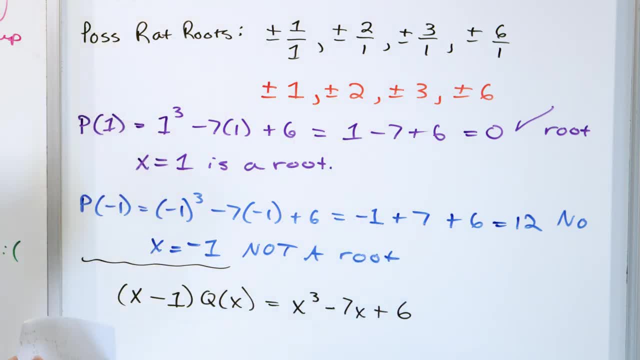 Because if you set this thing equal to 0, then you would solve for the 1, and that would be one of the roots. But that's not all of them. There has to be some other term multiplied, which I'm representing as q of x. 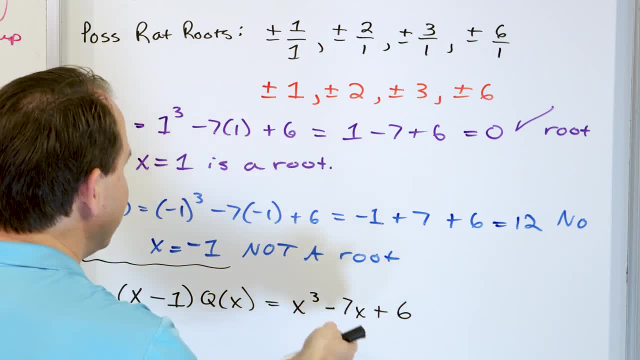 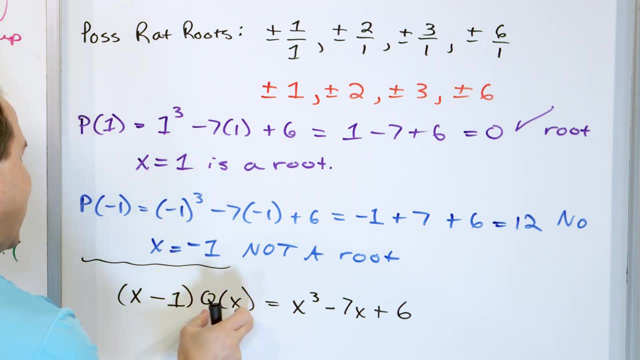 It's some function of x. In other words, it could be x minus 2 or x minus 3, as the other two roots here. I don't know what they are, But I know that there has to be something out here, because all of them multiplied together. 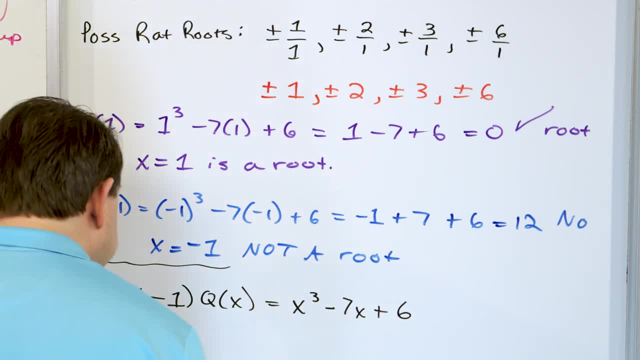 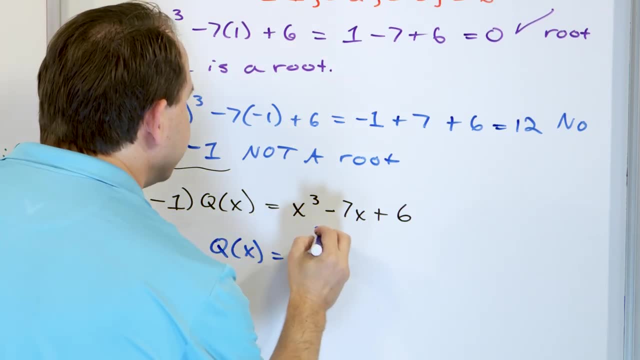 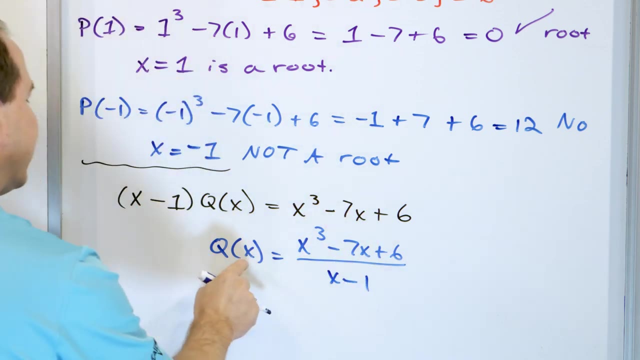 has to equal the original cubic. So what this means is that to figure out what the other roots are, we need to do long division, which I know you guys really love, But that's why we spent so much time on it. We need to take the original polynomial and divide by the x minus 1.. 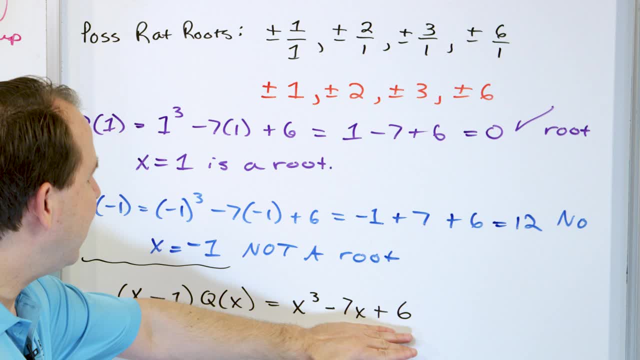 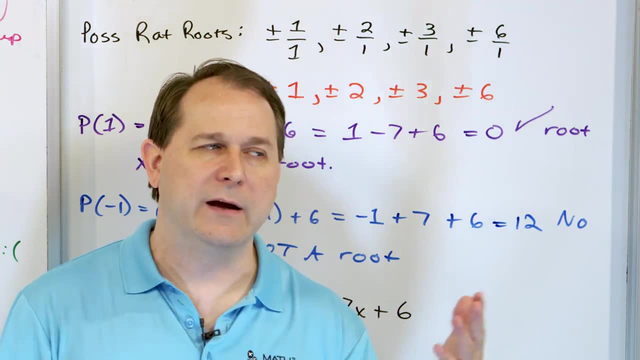 We did problems like this before, But anyway, this is the polynomial given to us. We know that if we knew all the roots, we should be able to write it in some kind of factored form, like we do for binomials or for quadratic equations. 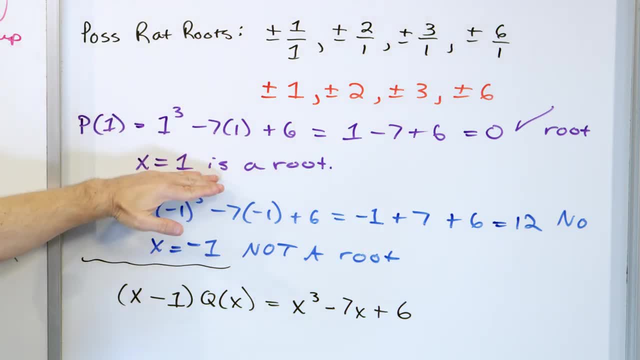 all the time, One of the roots we actually already found. So we know that there has to be 1 parentheses as x minus 1. Because if you set this thing equal to 0, then you would solve for the 1. And that would be one of the roots. 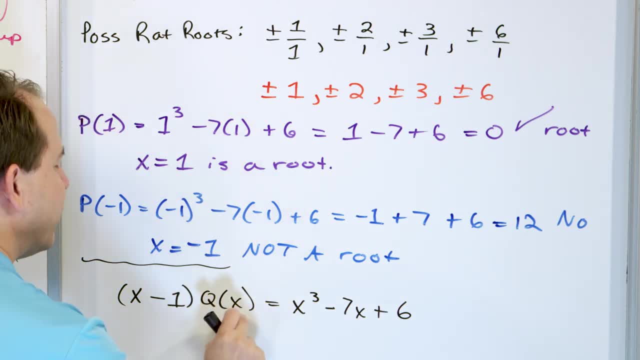 But that's not all of them. There has to be some other term multiplied, which I'm representing as q- of x. It's some function of x. In other words, it could be x minus 2 or x minus 3, as the other two roots here. 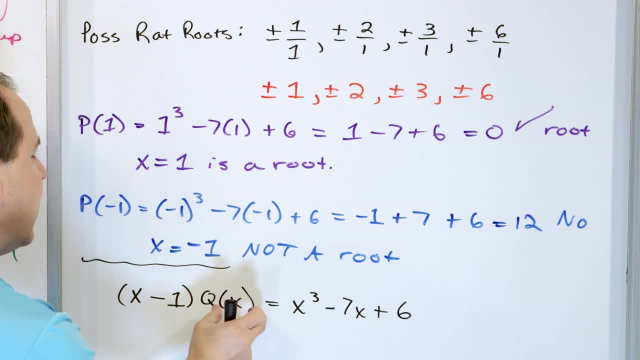 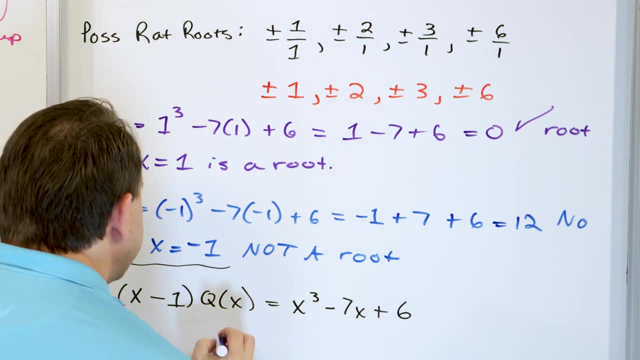 I don't know what they are, But I know that there has to be something out here, because all of them multiplied together has to equal the original cubic. So what this means is that to figure out what the other roots are, we need to do long division, which I know you guys really love. 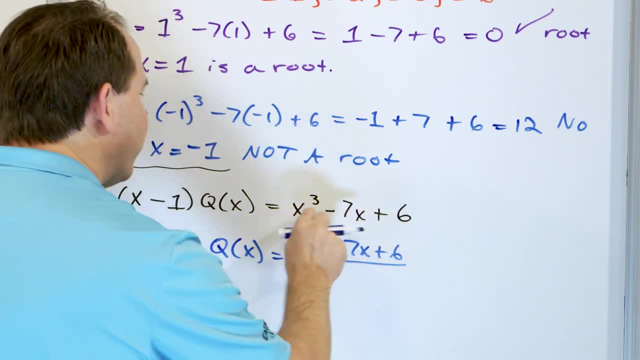 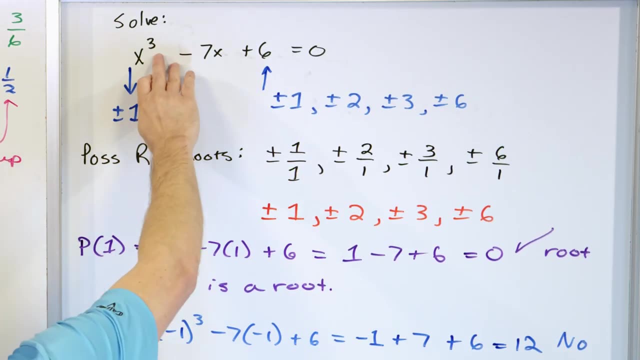 But that's why we spent so much time on it. We need to take the original polynomial and divide by the x minus 1.. That's going to give us whatever this is, And because this thing is a cubic equation and we already have one root when we divide it. 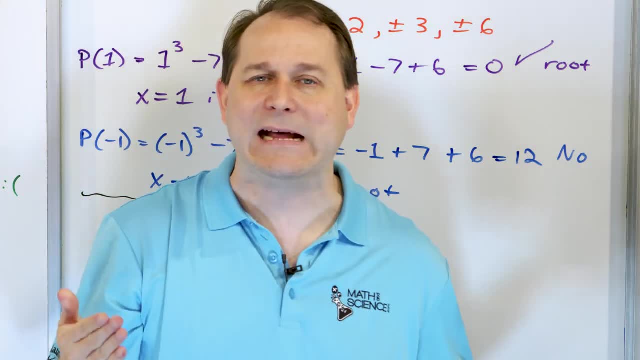 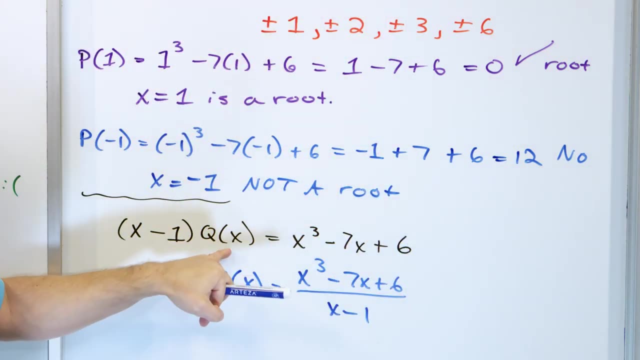 we're going to be left with q of x, which will be quadratic. It has to be an x squared quadratic because the entire thing is x cubed And we have an x minus 1 multiplied. So this has to be 1 degree lower because this is an x. 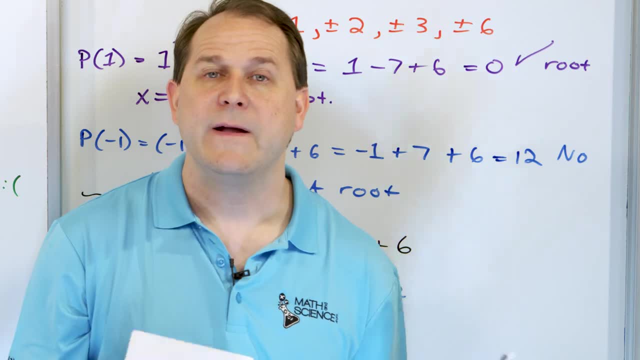 And this will have to be an x squared term. And I guess I'm trying to tell you that once we do the division, we expect to see a quadratic term, And we know how to do it, We know how to solve all quadratic equations. 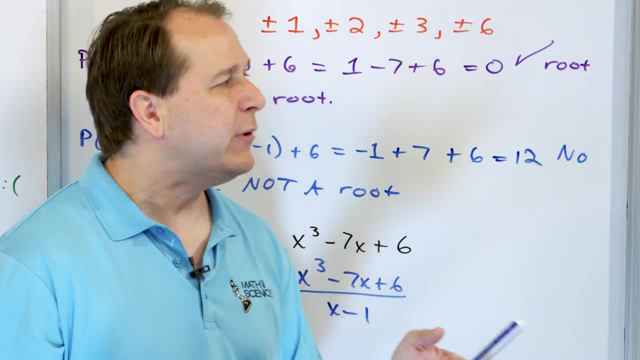 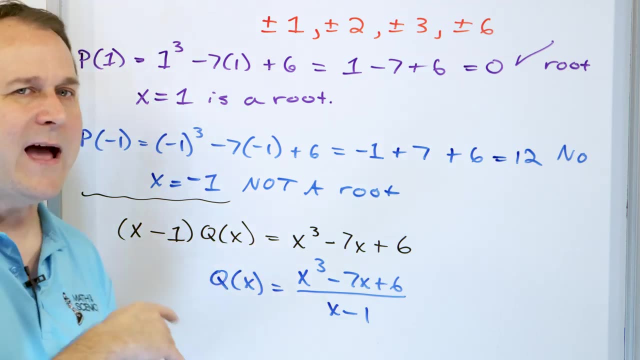 We can just use a quadratic formula even if we can't factor it. So even though you only found one root, we can do division to find what's left over as the remaining factors. Once we have that, we can always solve quadratic formulas. 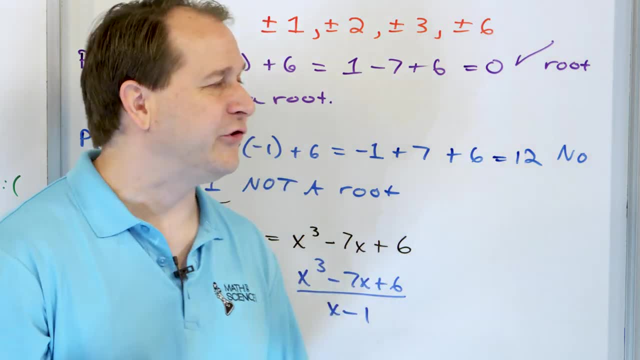 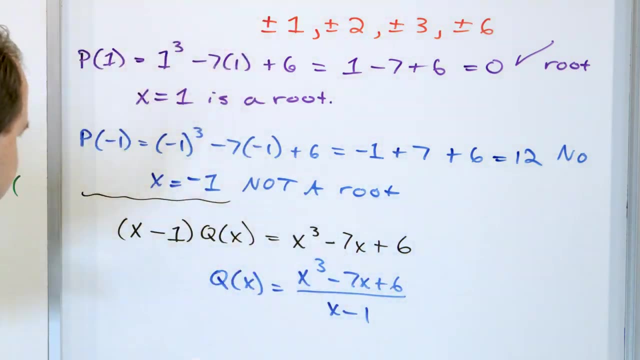 and we can find the other two, And if those other roots are rational, then they will have been in our list all along. We could, of course, continue cranking through this list, but this is going to take time as well. So what's the easiest way to do this division? 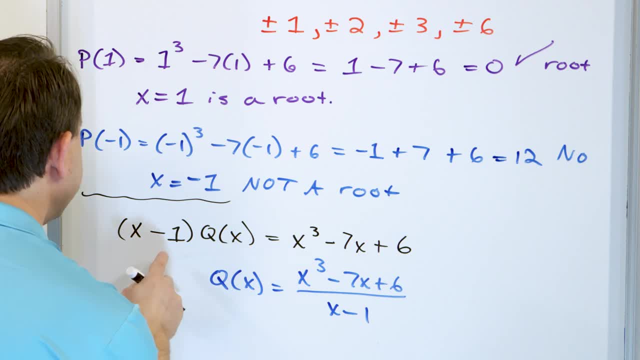 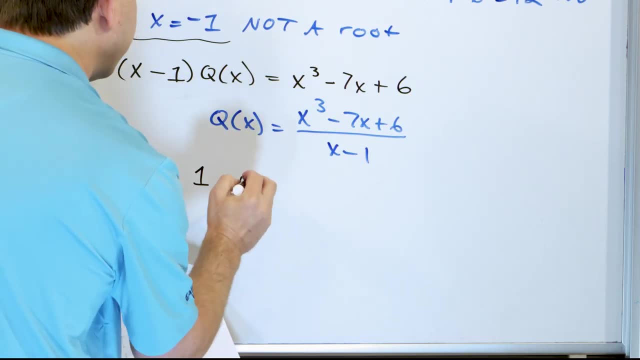 I think you will agree with me. the easiest way to do it is synthetic division. So whenever we write this down, we're dividing by 1x cubed. There is no x squared term, So we have to remind myself this is the x squared term. 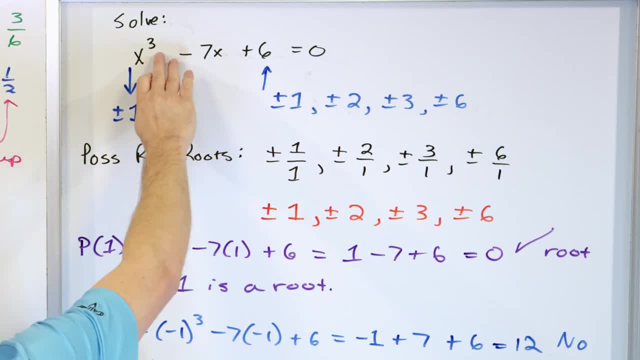 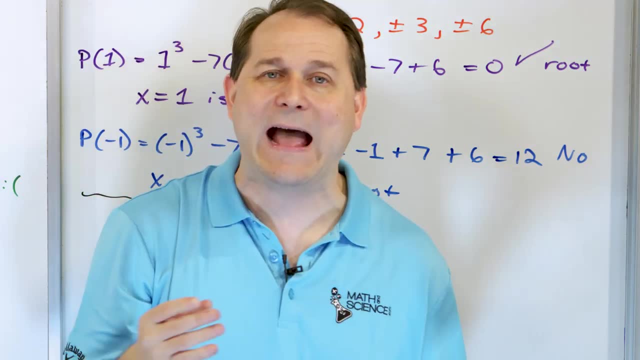 That's going to give us. whatever this is, And because this thing is a cubic equation and we already have one root, when we divide it we're going to be left with q of x, which will be quadratic. It has to be an x squared quadratic because the entire thing is x cubed and we have an. 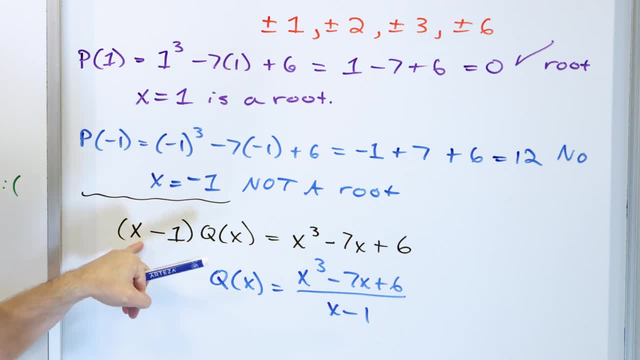 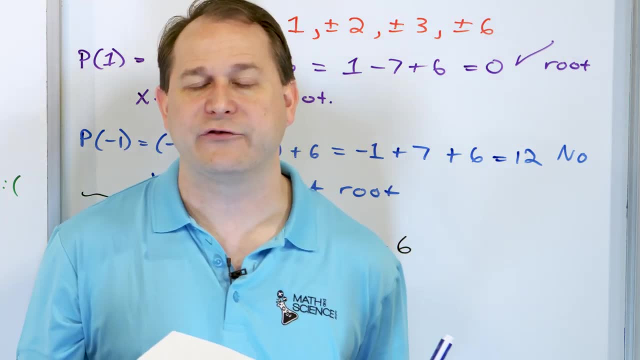 x minus 1 multiplied. So this has to be one degree lower because this is an x and this will have to be an x squared term. And I guess I'm trying to tell you, I'm trying to tell you that once we do the division, we expect to see a quadratic term. 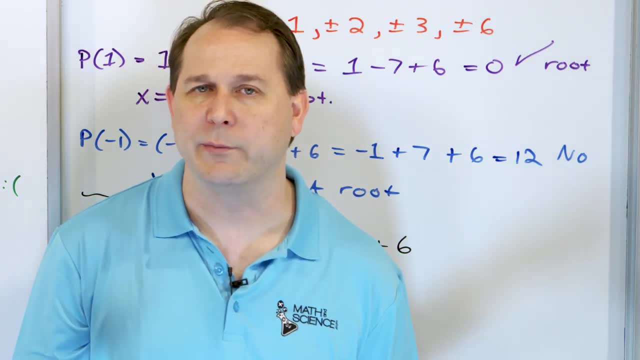 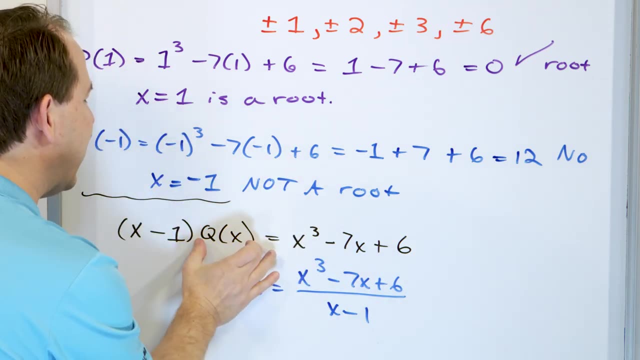 We know how to solve all quadratic equations. We can just use the quadratic formula even if we can't factor it. So even though you only found one root, we can do division to find what's left over as the remaining factors. Once we have that, we can always solve quadratic formulas and we can find the other two. 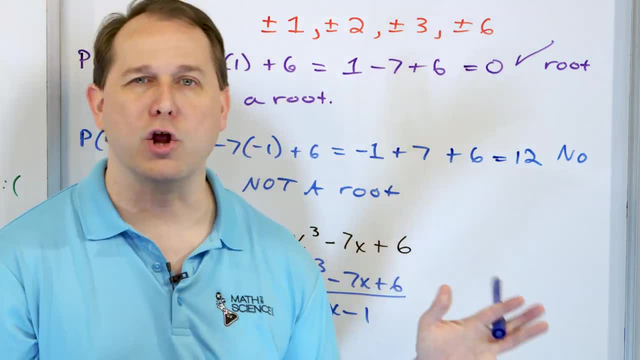 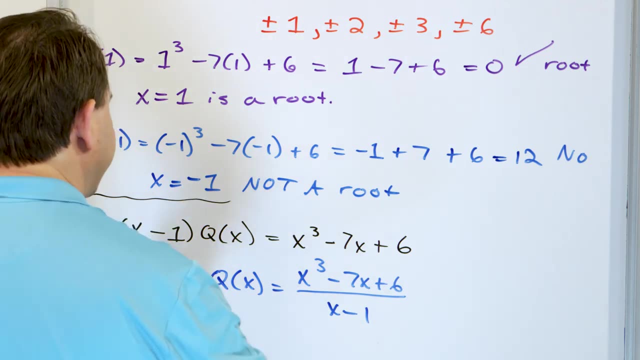 And if those other roots are rational, then they will have been in our list all along. We could, of course, continue cranking through this list, but this is going to take time as well, Okay, So what's the easiest way to do this division? 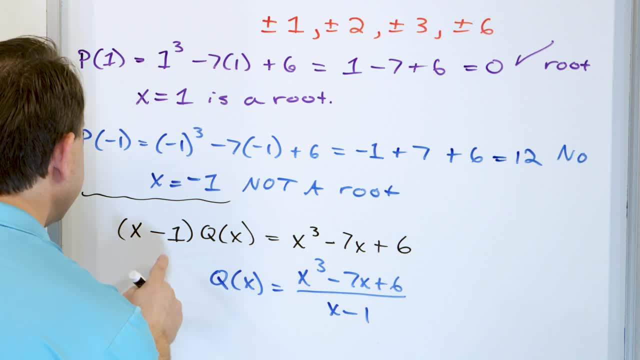 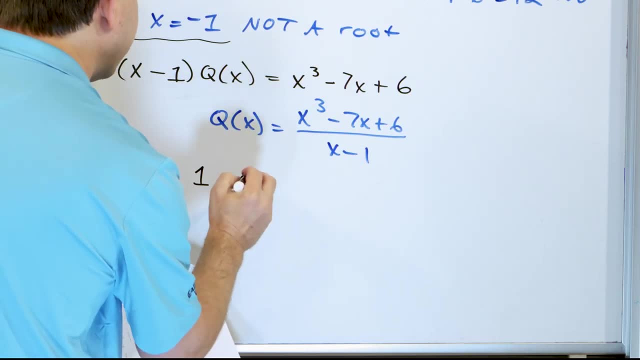 I think you will agree with me. the easiest way to do it is synthetic division. So whenever we write this down, we're dividing by one x cubed. There is no x squared term, so we have to. I'll remind myself: this is the x squared. 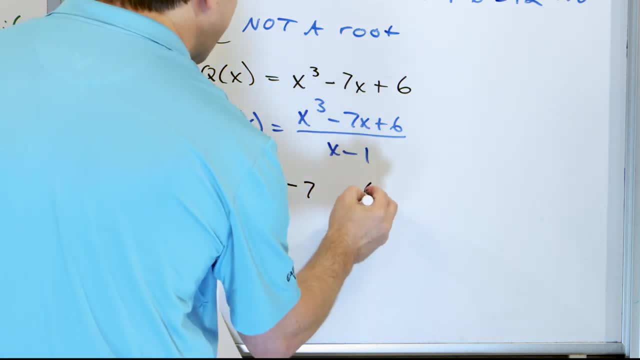 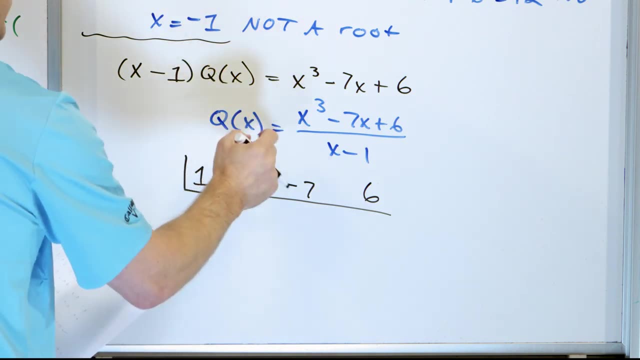 term. so I have to put a zero there. We have a negative 7 for the x term and we have a 6 there, And then I'm going to divide it by this term. But remember, when we do synthetic division we change the sign of what we're dividing. 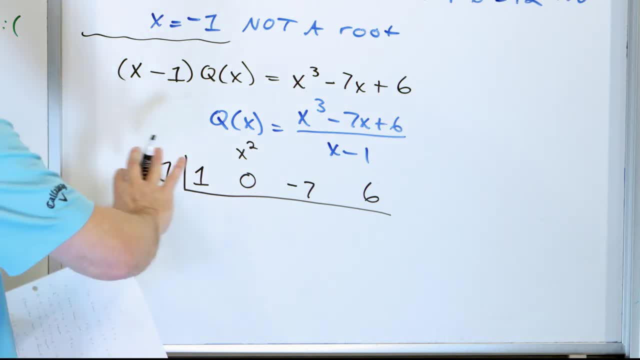 by When we do adding instead of subtracting. we covered all of this in synthetic division. So if you are looking at me cross-eyed because you don't know what I'm doing, it just means you need to go back and learn synthetic division with me. 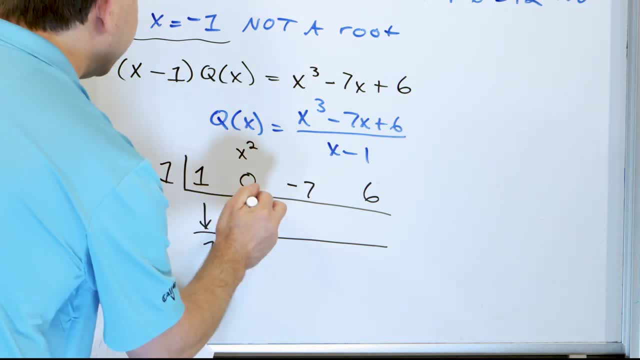 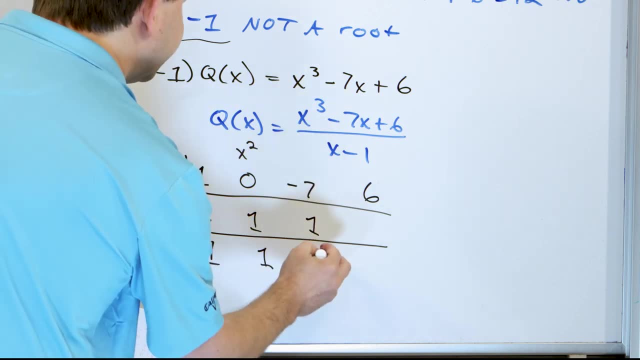 So first step is drop the 1 down. Then we multiply: 1 times 1 is 1.. Then we add: We get a 1.. Then 1 times 1 again is 1.. Then we add: We get a negative 6.. 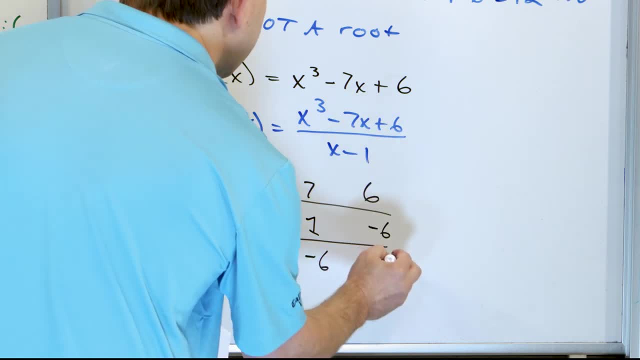 1 times negative. 6 is negative 6.. We add and we get a zero. Now, we always expect the remainder to be zero when we divide by a factor. Now, we always expect the remainder to be zero when we divide by a factor. 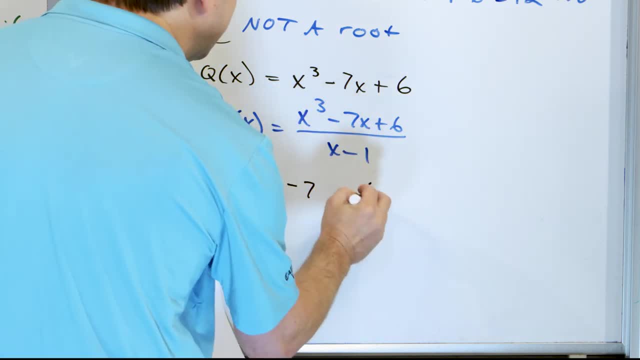 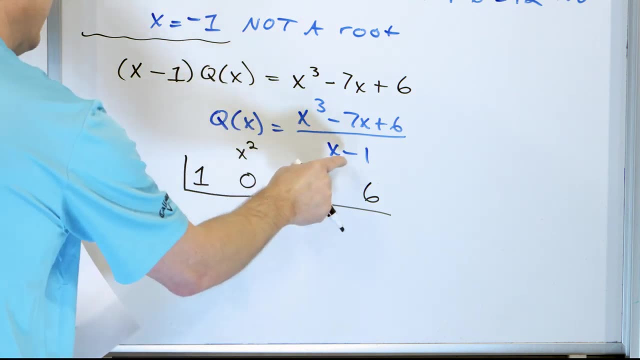 So I have to put a 0 there. We have a negative 7 for the x term and we have a 6 there, And then I'm going to divide it by this term. But remember, when we do synthetic division we change the sign of what we're dividing by. 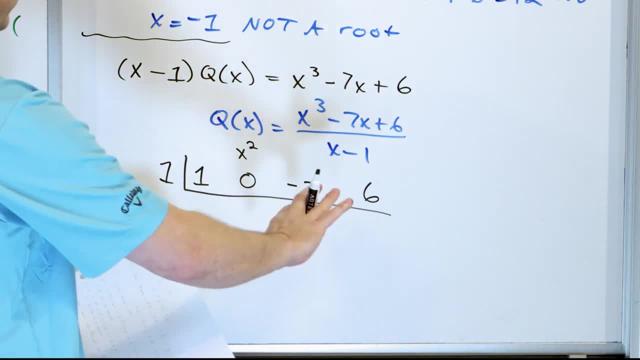 That allows us to do adding instead of subtracting. We covered all of this in synthetic division, So if you are looking at me cross-eyed because you don't know what I'm doing, it just means you need to go back and learn synthetic division. 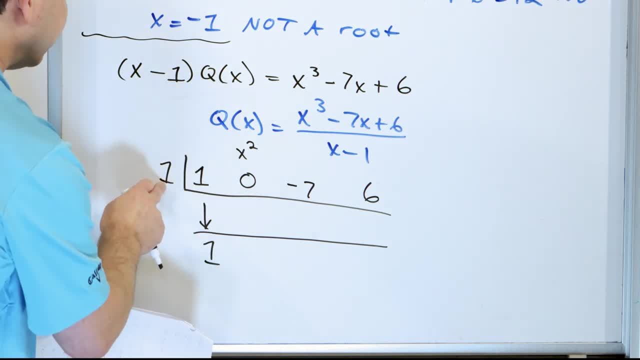 with me. So first step is drop the 1 down, Then we multiply: 1 times 1 is 1.. Then we add: We get a 1.. Then 1 times 1 again is 1.. Then we add. 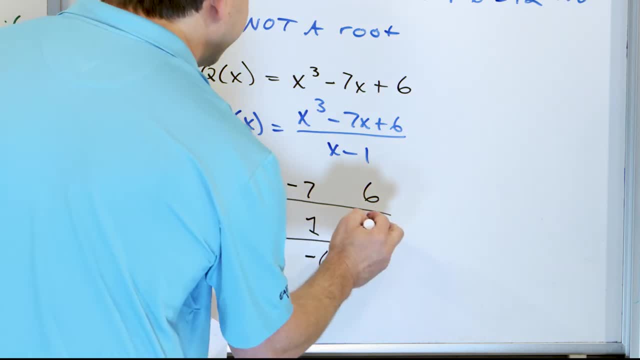 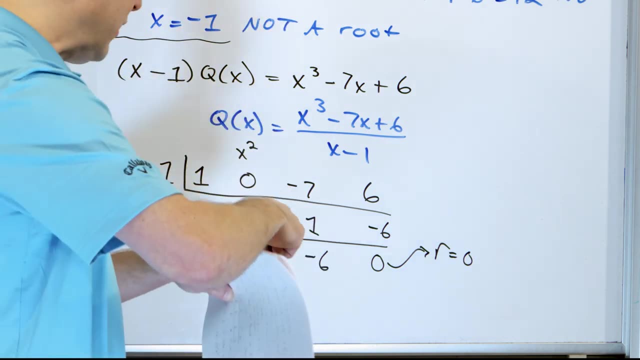 We get a negative 6.. 1 times negative 6 is negative 6.. We add and we get a 0. Now we always expect the remainder to be 0 when we divide by a factor. What I mean by that is, if I take the number 45,, 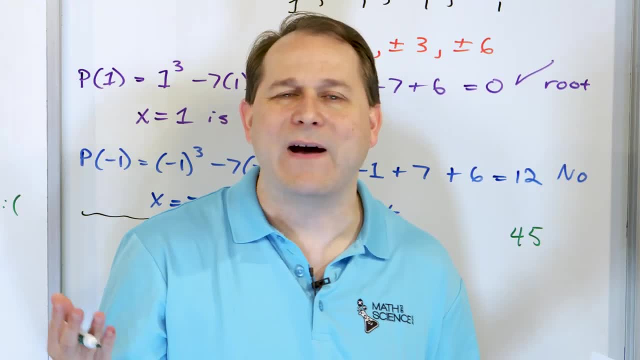 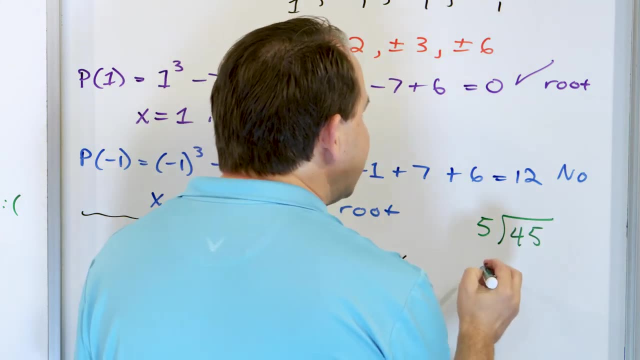 OK, that's some number. I know that the number 5 is a factor of 45. I know it divides evenly. So if I divide by 5, I know what I'm going to get is 9 with a remainder of 0, because it goes. 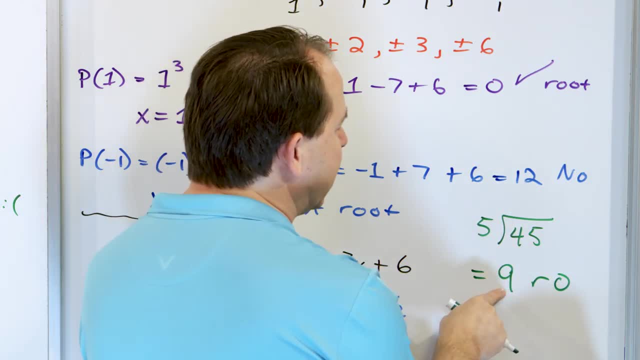 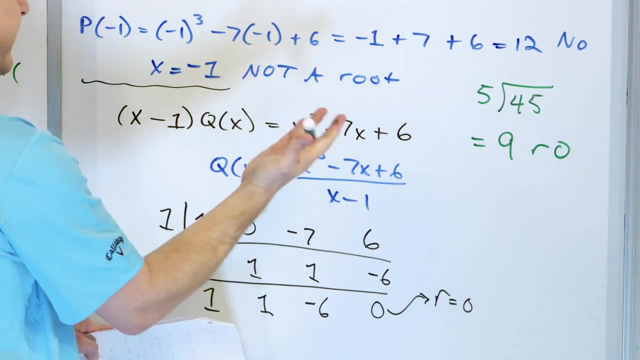 in an even number of times, Because when I divide by a factor, I expect to get something with no remainder at all left over. So what I'm saying is, when I take the polynomial, I divide by a known factor. I know it's a factor because it's a root. 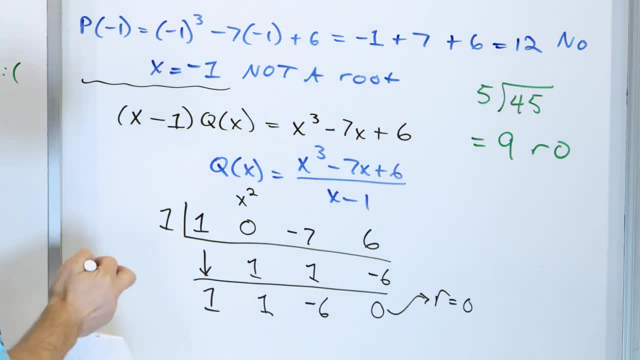 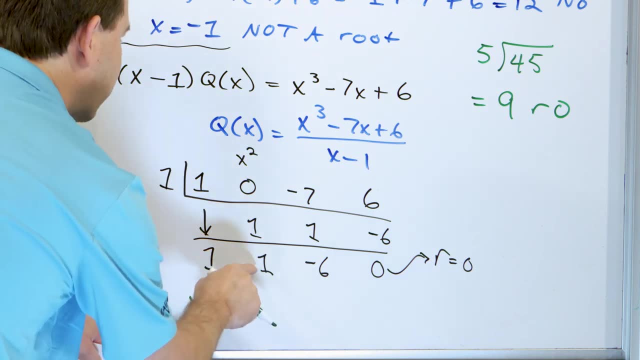 Then what I'm left with should have no remainder just like this, And so what I have found is that what's left over here is x squared. This has to be 1 degree less than the cube, So it has to be x squared. 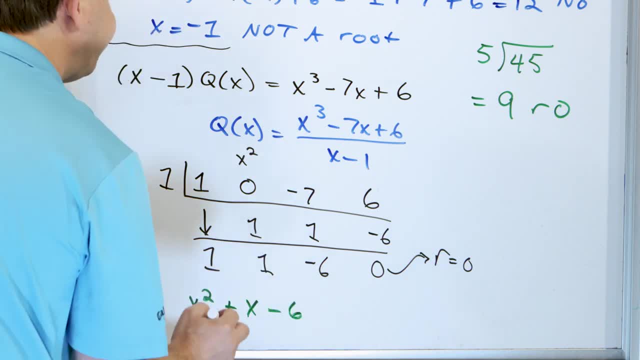 1x squared plus 1x minus 6.. This is what is left. What we found out is that q of x is equal to that. So let me just double check myself: x squared plus 6 minus 6.. So what we're saying is that these two things multiplied: 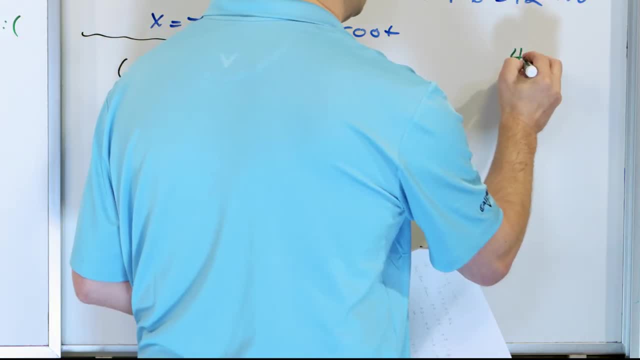 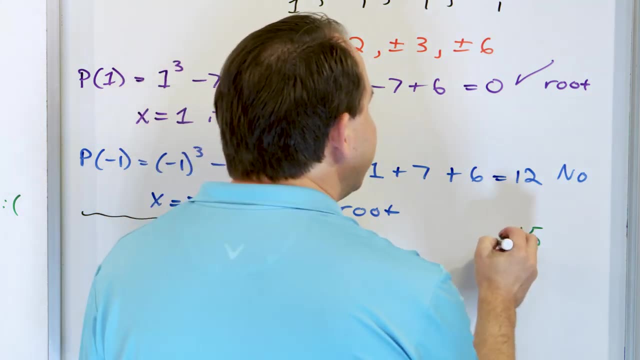 What I mean by that is, if I take the number 45- and that's some number- I know that the number 5 is a factor of 45. I know it divides evenly. So if I divide by 5, I know what I'm going to get is 9 with a remainder of 0, because 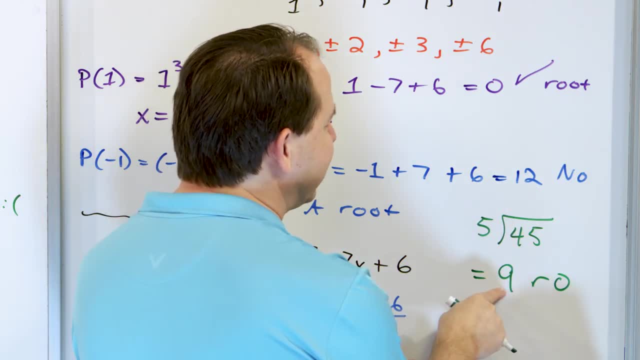 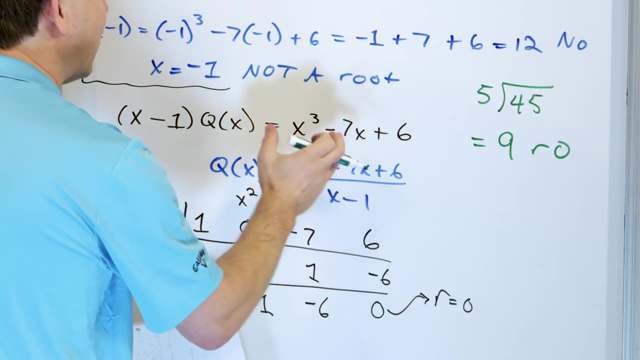 it goes in an even number of times, Because when I divide by a factor, I expect to get something with no remainder at all left over. So what I'm saying is, when I take the polynomial, I divide by a known factor. I know it's a factor because it's a root. 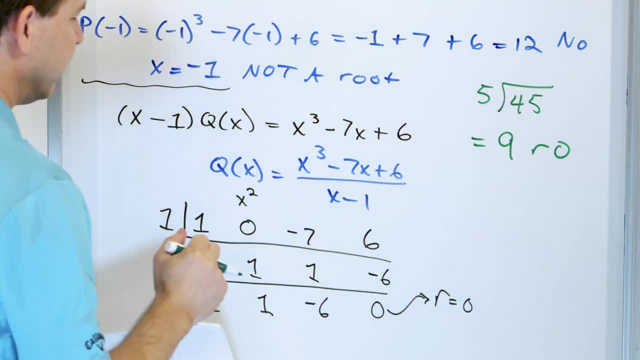 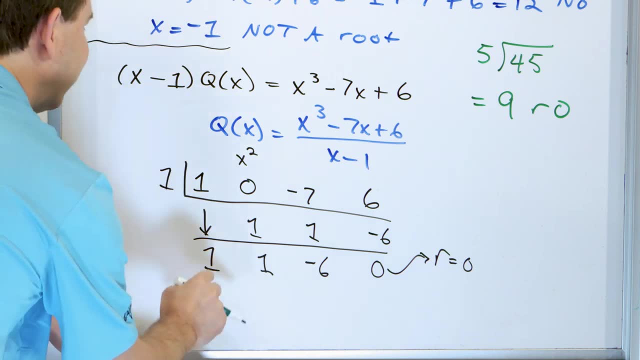 Then what I'm left with should have no remainder just like this, And so what I found is that what's left over here is x squared. This has to be one degree less than the cube, So it has to be x squared, 1x squared plus 1x minus 6. 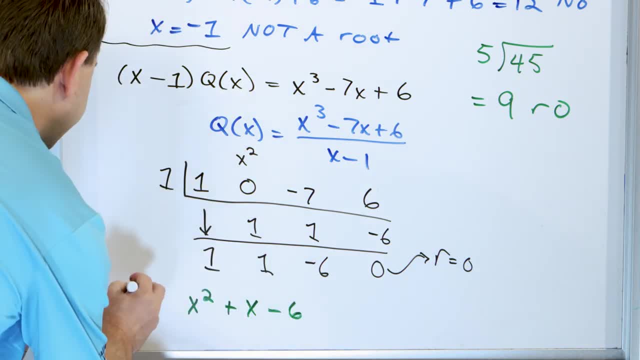 This is what is left. What we found out is that Q of X is Equal to that. So let me just double check myself: x squared plus 6 minus 6. So what we're saying is that these two things multiplied together are what multiply to give us this guy. 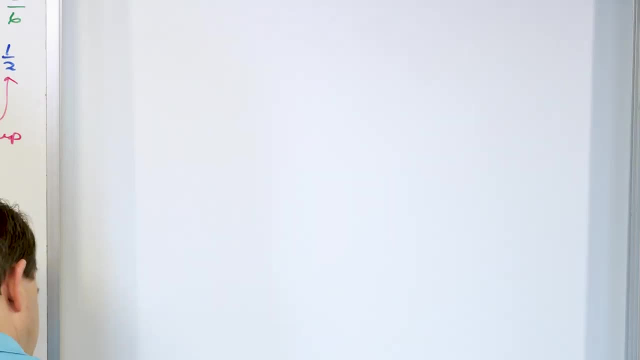 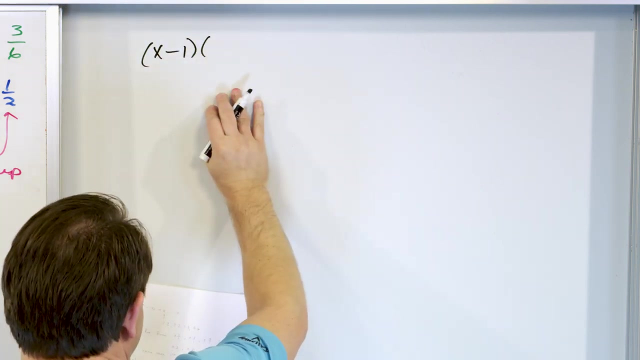 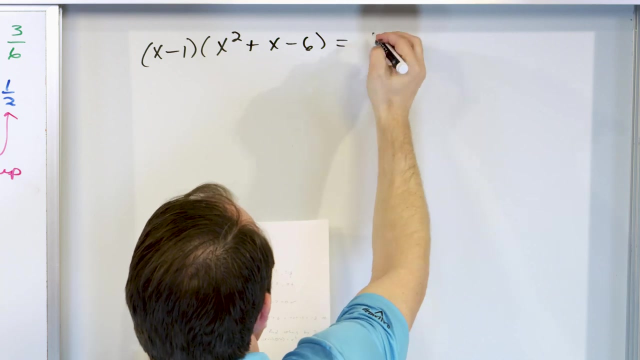 So let me write that on the last board here. What we have basically said is that x minus 1, which was that known factor that we guessed, and Then we just figured out the answer for Q to a Q of X, the division. We're saying that this has to equal x cubed. 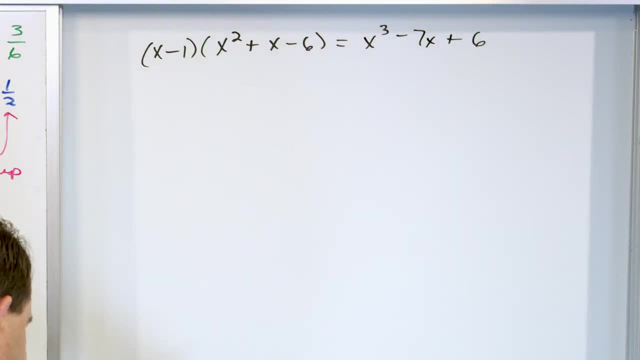 minus 7x plus 6. All right, Now we know how to solve these things, because we're trying to set them equal to 0, right, How do we set this thing equal to 0?? Basically, we have x minus 1 x squared plus x minus 6. 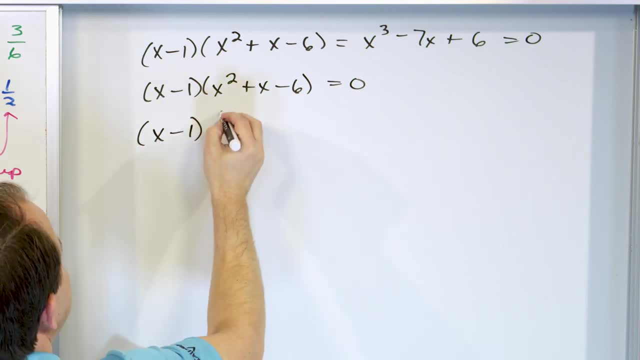 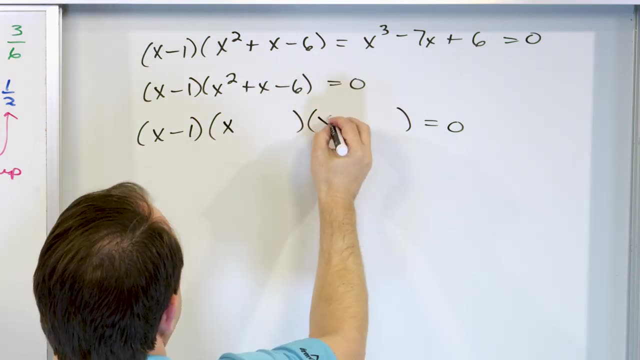 Equal 0.. Well, we already have this one already here. Now let's try to factor this if it doesn't factor. if this doesn't factor, we can still do the quadratic formula on it. but let's try to factor it: x and x, and Then 2 times 3 is 6, and if you work out the signs, 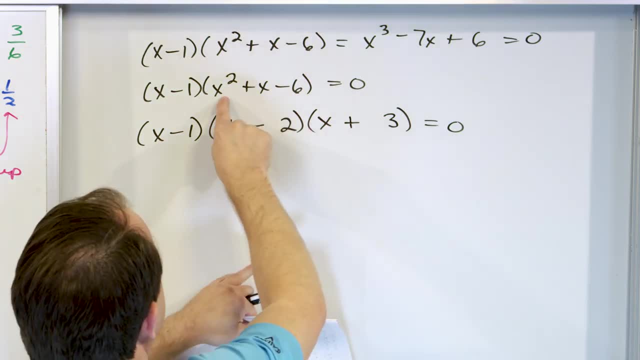 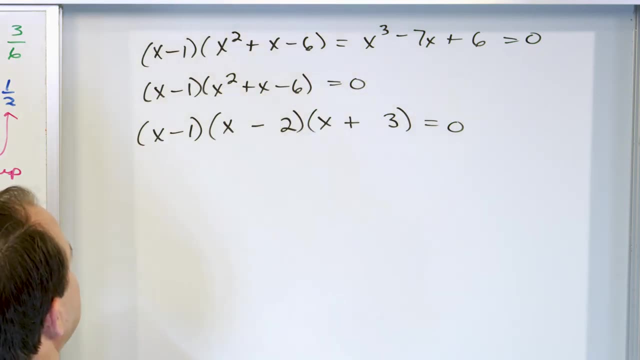 This is the way that it works, because you'll have x times x is X squared. negative 2 times 3 is negative 6.. That's negative 2x, That's positive 3x. that adds together to give you the positive X in the middle. 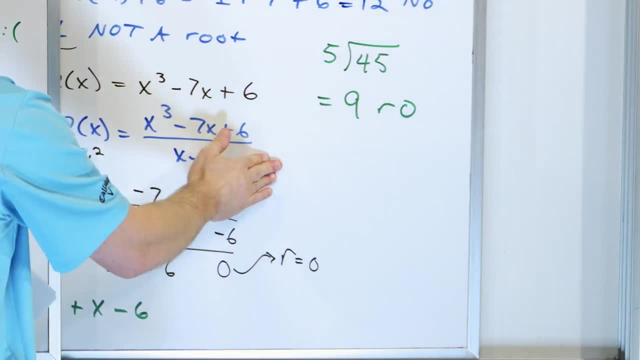 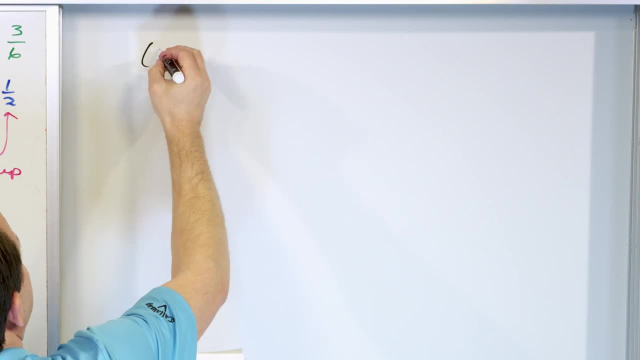 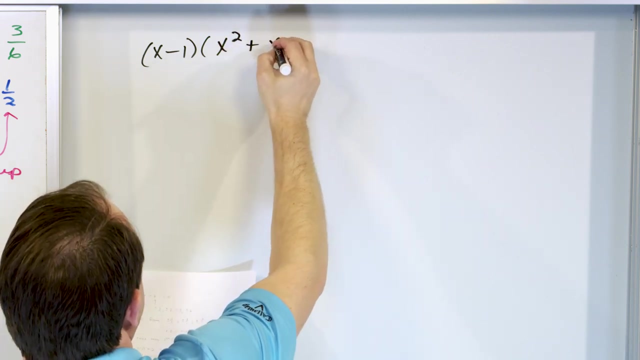 together are what multiply to give us this guy. So let me write that on the last board Here. what we have basically said is that x minus 1, which was that known factor that we guessed, and then we just figured out the answer for q of x, the division. 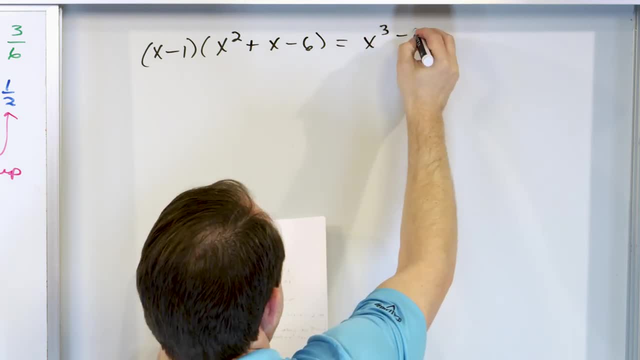 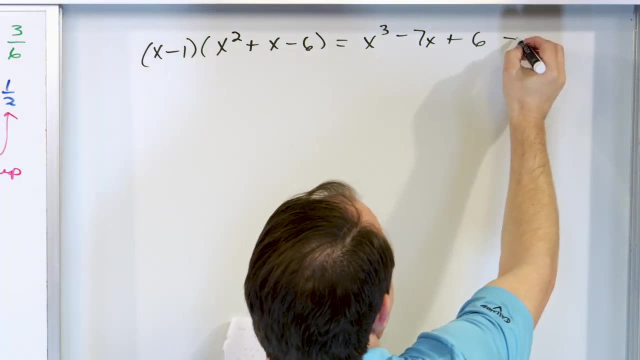 we're saying that this has to equal x cubed minus 7x plus 6.. All right, now we know how to solve these things, because we're trying to set them equal to 0, right. How do we set this thing equal to 0?? 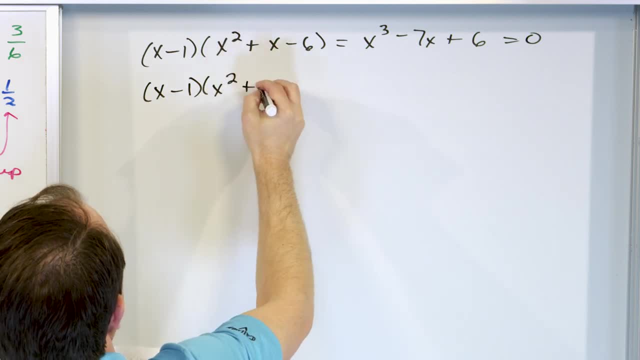 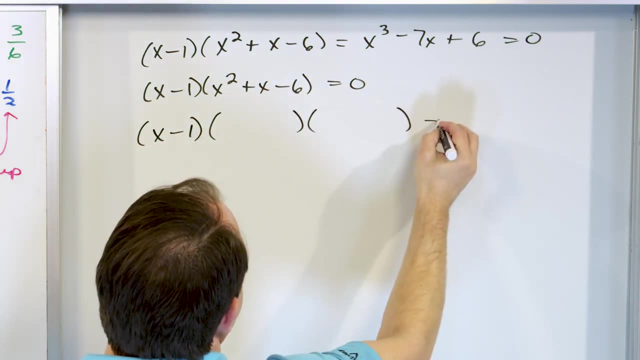 Basically, we have x minus 1.. x squared plus x minus 6 equals 0.. Well, we already have this one already here. Now let's try to factor this. If it doesn't factor. if this doesn't factor, we can still do the quadratic formula on it. 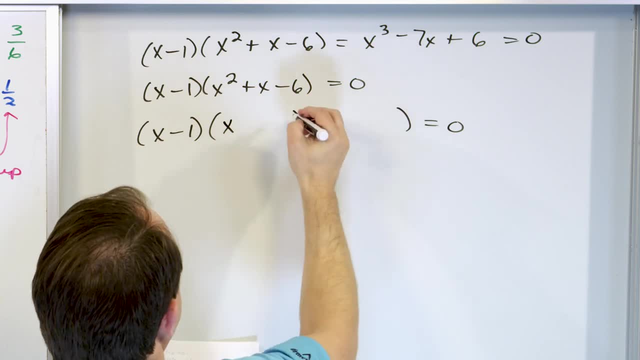 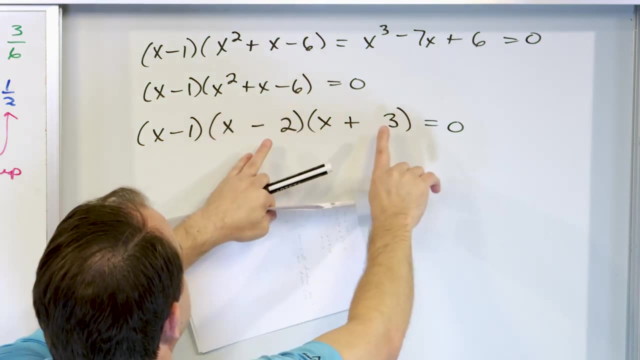 but let's try to factor it x and x and then 2 times 3 is 6.. And if you work out the signs, this is the way that it works, Because you'll have x times x is x squared Negative. 2 times 3 is negative 6.. 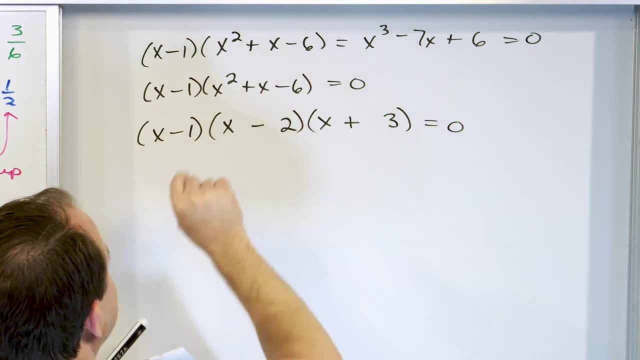 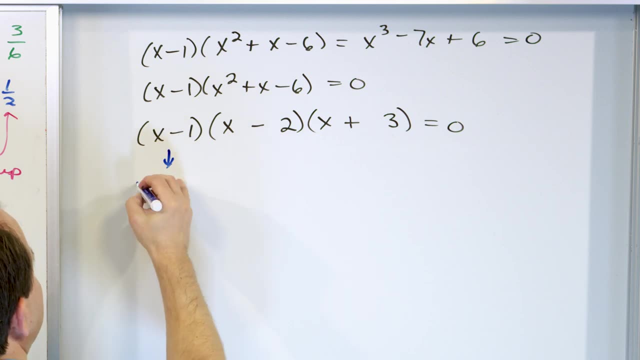 That's negative 2x, That's positive 3x, That adds together to give you the positive x And you'll have x in the middle. So you see, now we have figured out that from this, which we already knew. 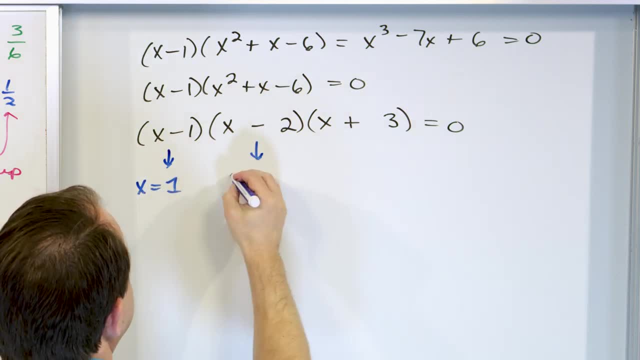 x can be equal to 1 as a root From this. when we set it equal to 0,. x can be equal to 2 as a root From this guy. when we set it equal to 0, x can be negative 3 as a root. 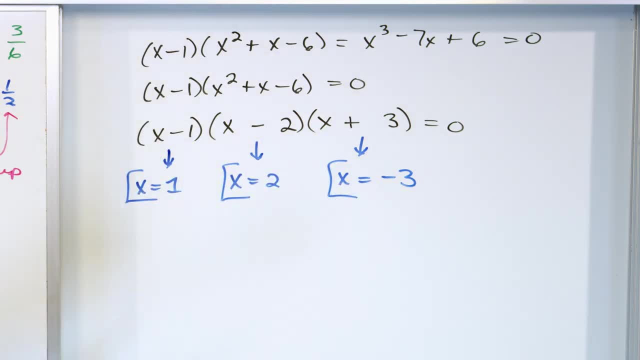 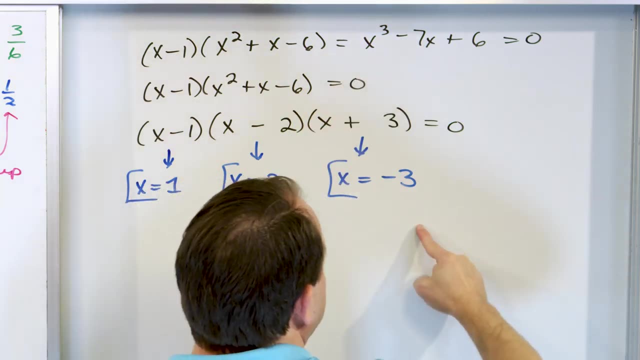 So x is equal to 1.. x is equal to 2.. x is equal to negative 3.. Those are the three roots. We didn't have any complex roots in this case. That means this cubic polynomial cuts across the x-axis in three locations. 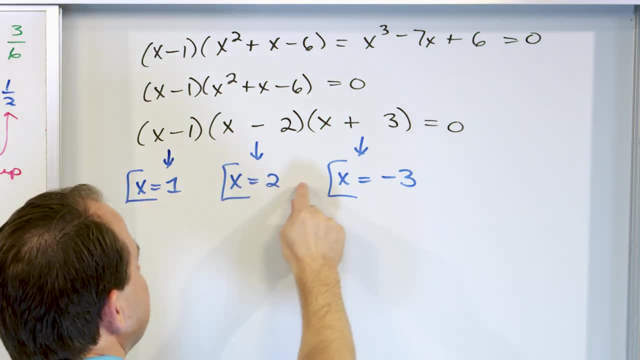 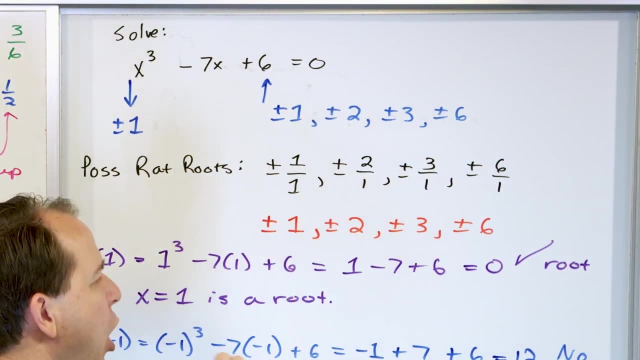 And notice we have three rational roots, So 1,, 2, and negative 3.. When we go back to our problem, our list did include 1,, 2, and negative 3.. So all of the rational roots that were actually. 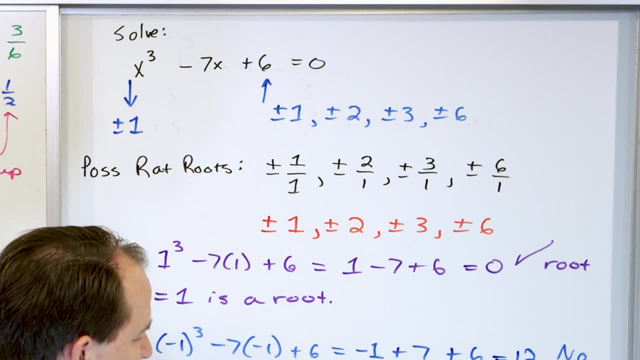 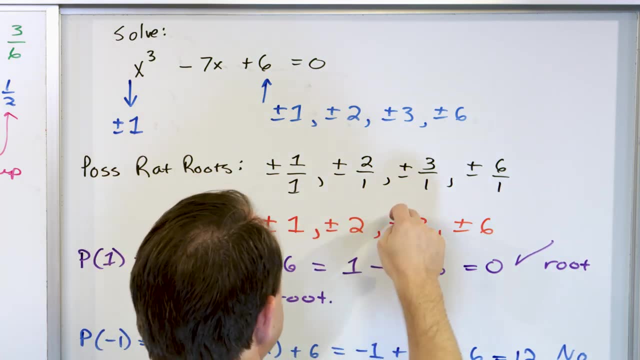 solutions of the problem were in our list. So if we didn't do this division business, we would have had to go and continue on substituting things in: plus 1, minus 1, plus 2, minus 2, plus 3, minus 3.. 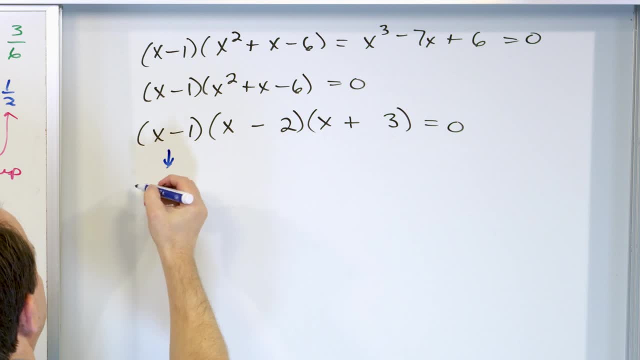 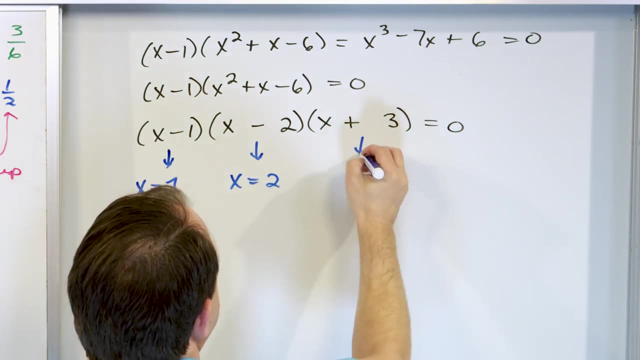 So you see, now we have figured out that from this, Which we already knew, X can be equal to 1. as a root from this, when we set it equal to 0, X can be equal to 2. as a root from this guy, when we set it equal to 0, X can be negative 3. 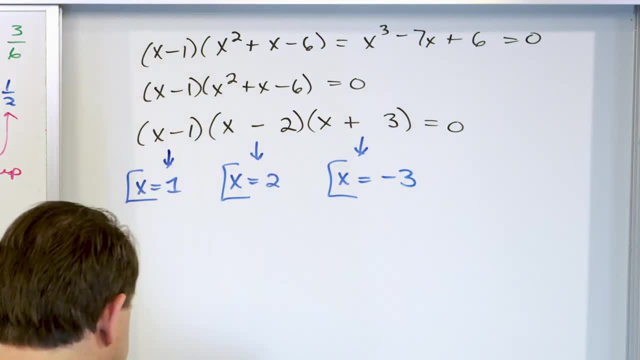 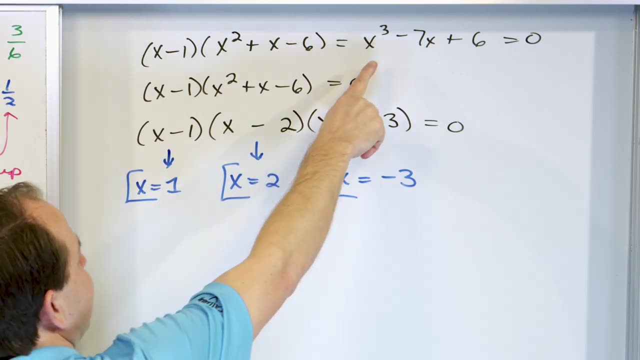 Is a root. so X is equal to 1, X is equal to 2, X is equal to negative 3. Those are the three roots. We didn't have any complex roots in this case. That means this cubic polynomial cuts across the x-axis in three locations and notice we have three rational roots. 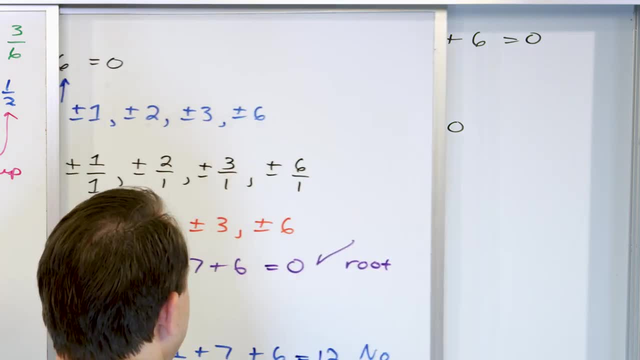 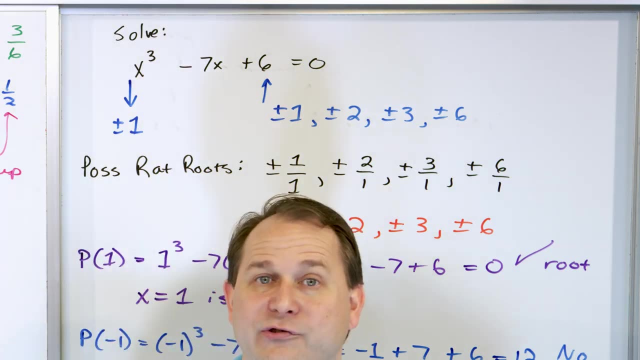 So 1, 2 and negative 3. when we go back to our problem, our list did include 1, 2 and negative 3, So all of the rational roots that were actually solutions of the problem were in our list. So if we didn't do this, division business. 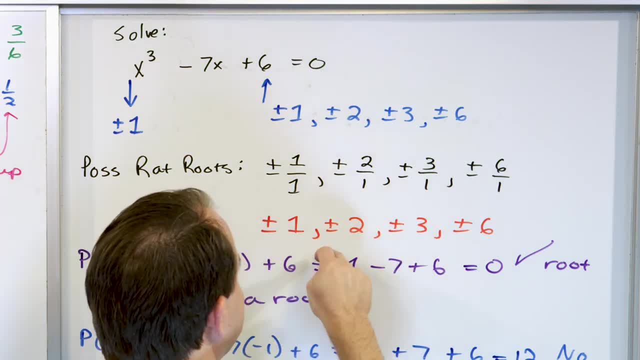 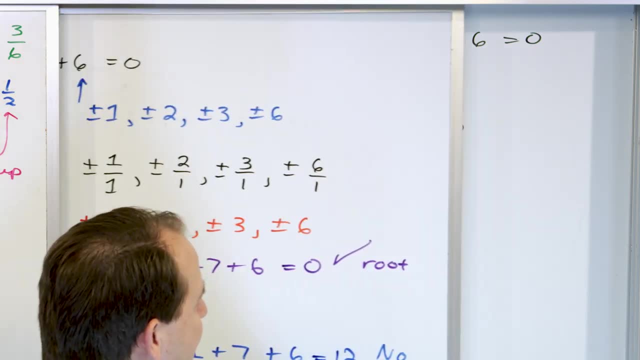 We would have had to go and continue on substituting things in: plus 1 minus 1, plus 2, minus 2, plus 3 Minus 3. we eventually would have got them all right. But the problem is you just never know when you're gonna get. you're gonna get the answer. 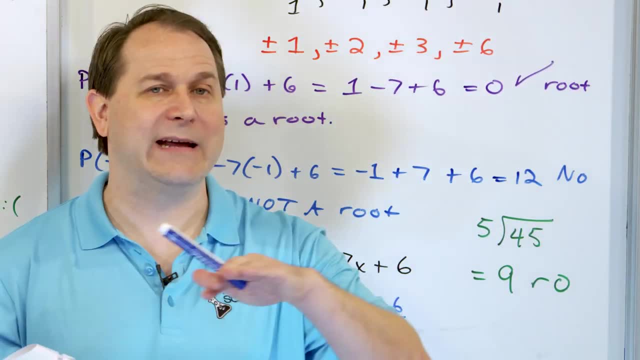 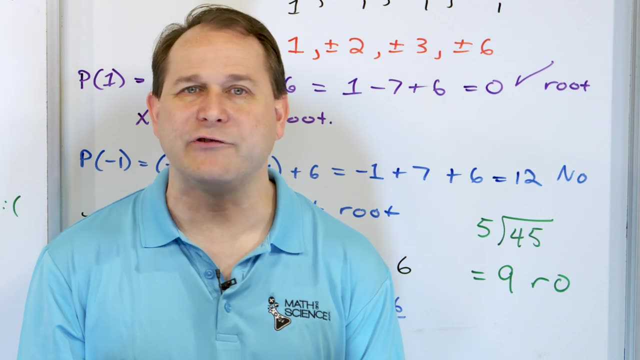 So you can be substituting in all day. You might substitute everything in that whole list and and get none of them to be in there, because all the roots might be, You know, Irrational or something else. you don't have any idea what they are, but if the polynomial has any rational roots, 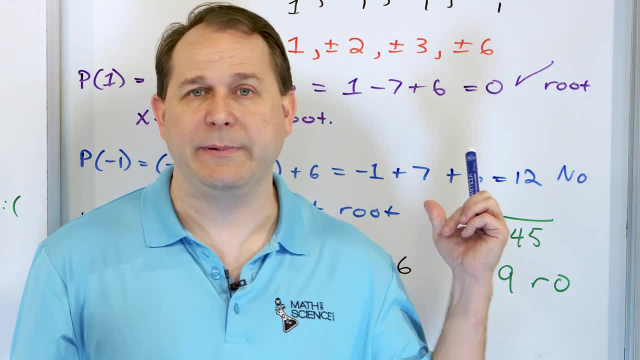 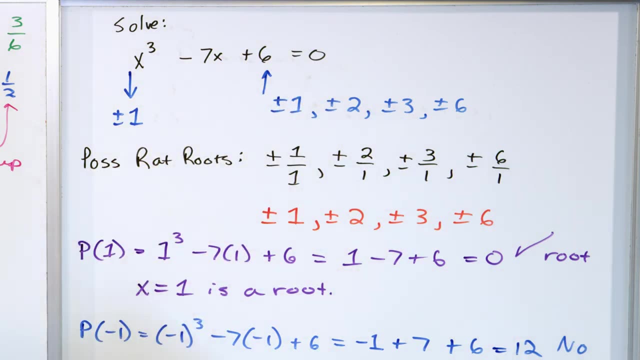 Meaning roots that are whole numbers or fractions, then they're going to be in this list. So, step number one, write your equation Down, descending. step number two: write the factors down here And up here. then you write the possible Rational roots as the divisions of all of these numbers, divided by all of these numbers. 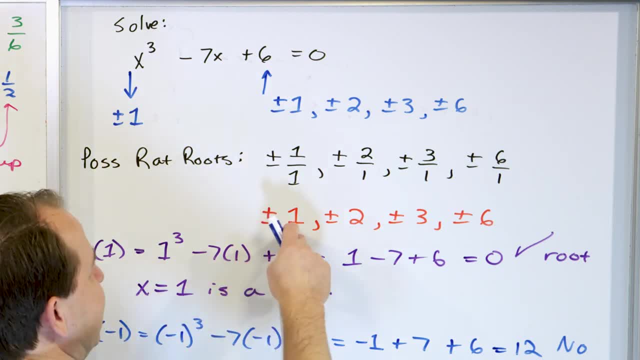 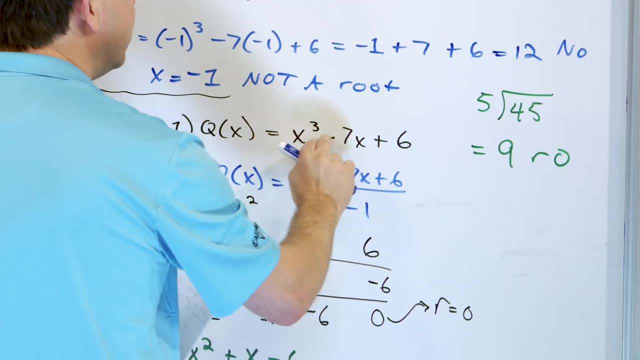 Simplify your list and then what you have to do is start guessing. start with the easy numbers, Find one. once you find one root, then you know that that root is a factor. times more factors must equal the polynomial that you Have. then by division you can figure out what the other factors are. and 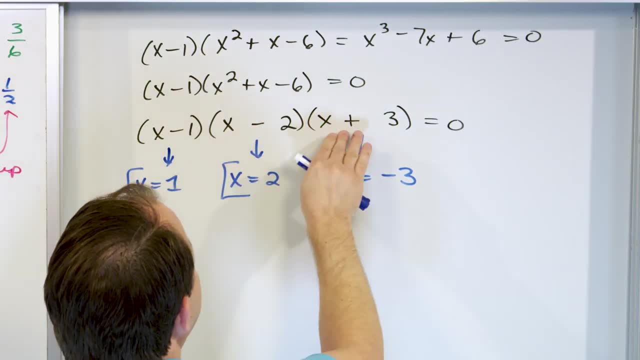 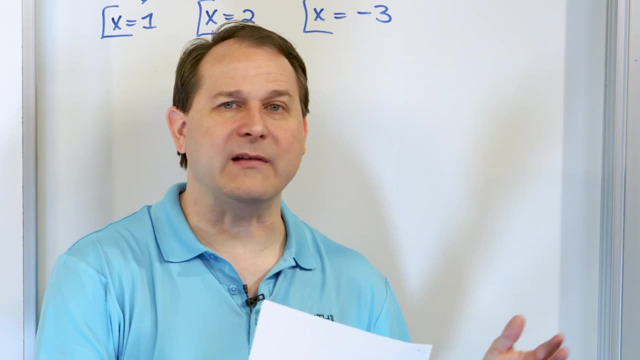 Then, once we had this, we were able to factor. if we were not Able to factor it, I could just set this quadratic equal to zero by itself and use the quadratic formula And figure out what the remaining two roots are. Maybe I get two complex roots out of it. 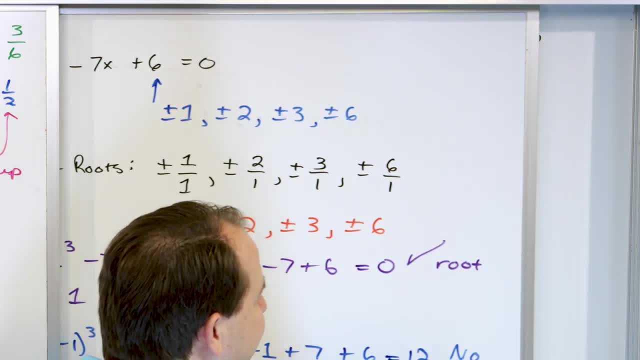 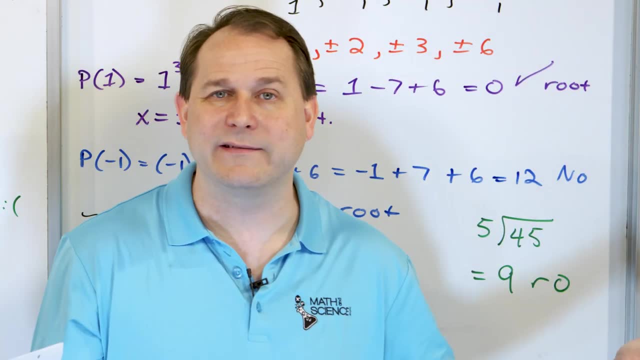 We eventually would have got them all. But the problem is you just never know when you're going to get the answer. So you can be substituting in all day. You might substitute everything in that whole list and get none of them to be in there. 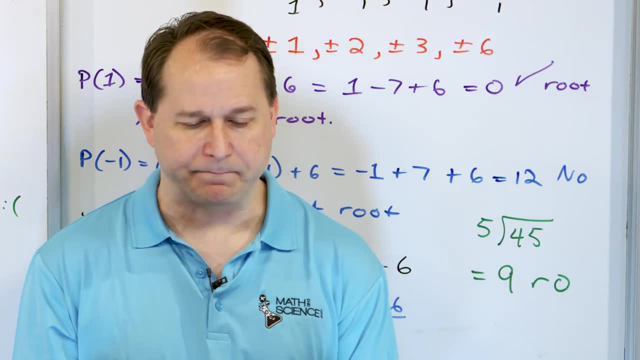 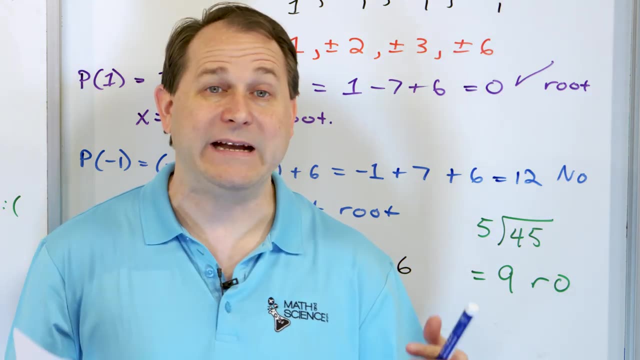 because all the roots might be irrational or something else. You don't have any idea what they are, But if the polynomial has any rational roots, meaning roots that are whole numbers or fractions, then they're going to be in this list. So step number 1, write your equation down, descending: 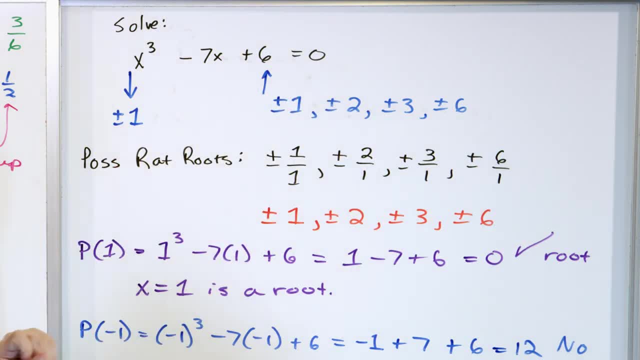 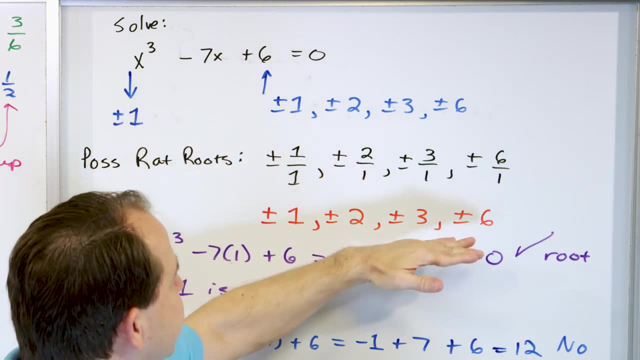 Step number 2, write the factors down here and up here. Then you write the possible rational roots as the divisible root Divisions of all of these numbers divided by all of these numbers. Simplify your list and then what you have to do.